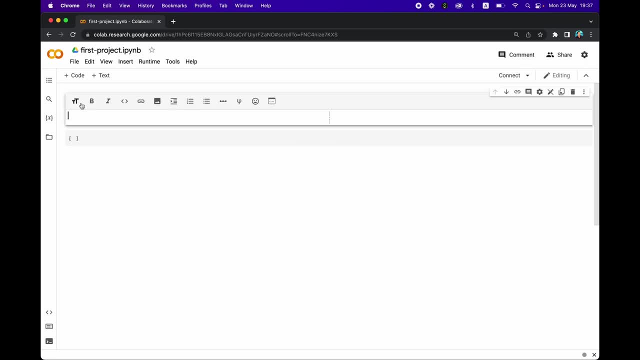 using the down button here, and then I'll double click here and I'll click on this button, which is the equivalence of a hash symbol, which will give the text a heading one. If you have two of it, it will be a heading two. So the great thing about using headings is that it allows you to neatly 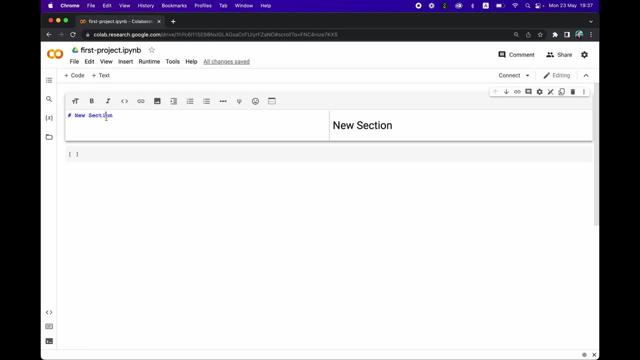 organize your Jupyter notebooks, So I'll show you. So here we're also going to make the text bold- My first ML project- And we're going to use two hash symbol, or you could click this button twice and then I'll also make it bold. 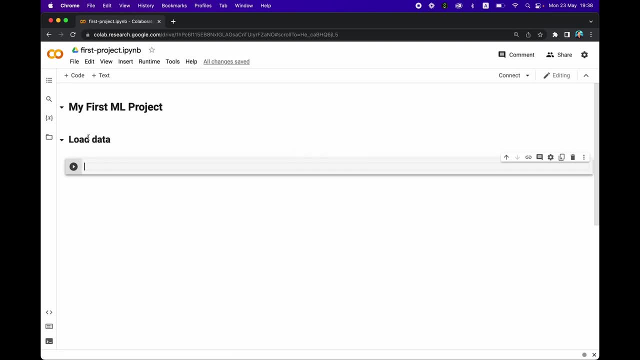 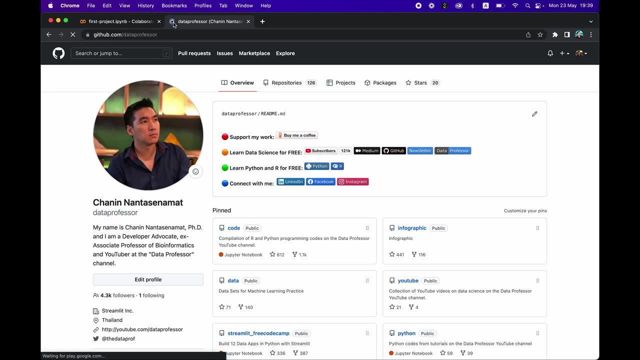 So typically we're going to start the project by loading in a data set. So let's find a data set to analyze And for that we're going to the GitHub of data professor And if you scroll down, one of the pinned repository will be called. 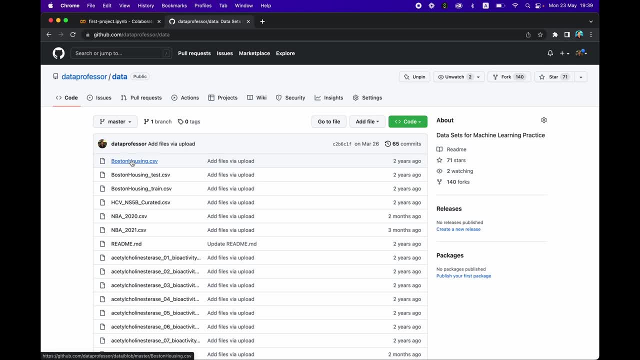 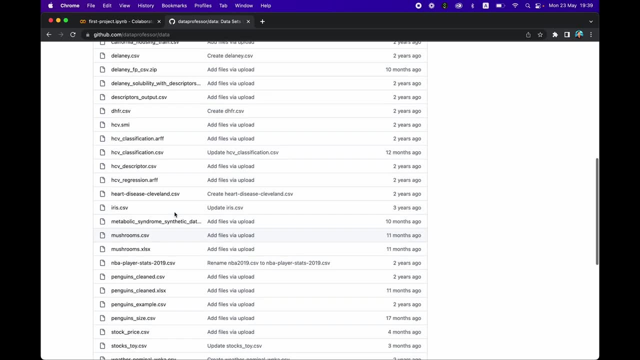 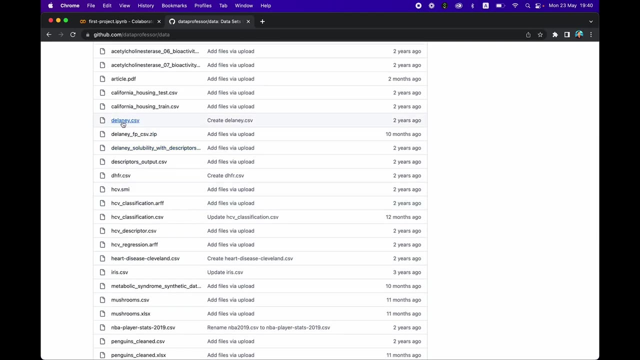 data, click on it And then there's a lot of data sets here that I have compiled over the years as a content creator. So a reasonably simple and unique data set that I would like to use here is the Delany data set, And I think it's this one. Let me have a look. 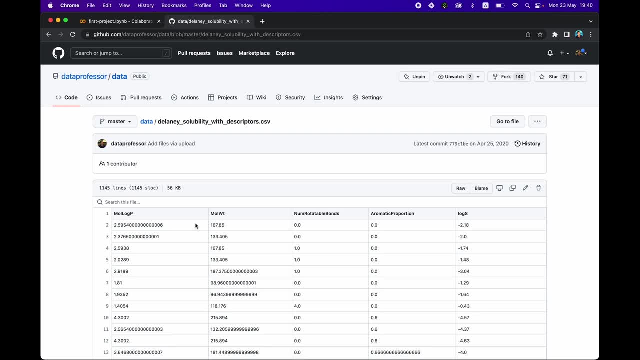 Okay, so this is a data set of the solubility of molecules And they are the fact that they are crucial for biologists and chemists in determining whether a molecule is soluble in water or solvent and whether they will be good drug candidates. And so let's have a. 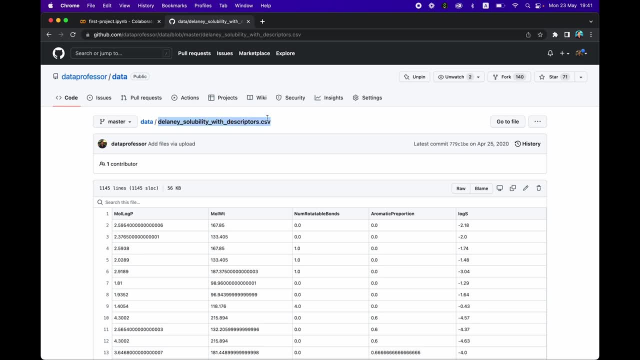 look here you can see that the data set here is in the format of a CSV And essentially it is a comma separated value file. So if you click on the raw link here, you're going to see the native file. let me zoom in And you're going to see that. 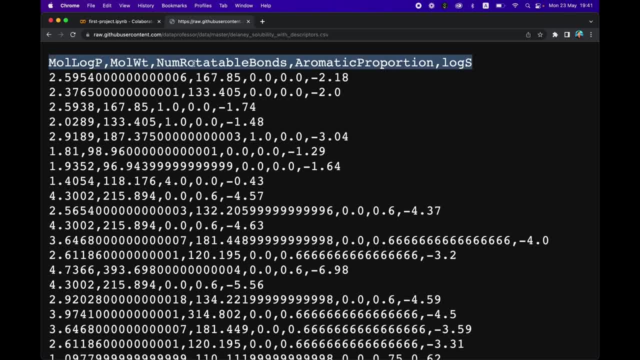 the first row will comprise of the names of the columns, And each word that you see here is the name of the column and it represents a single cell, and then you have the comma to separate it, And therefore the first word here and the second word here and the third word, and etc. 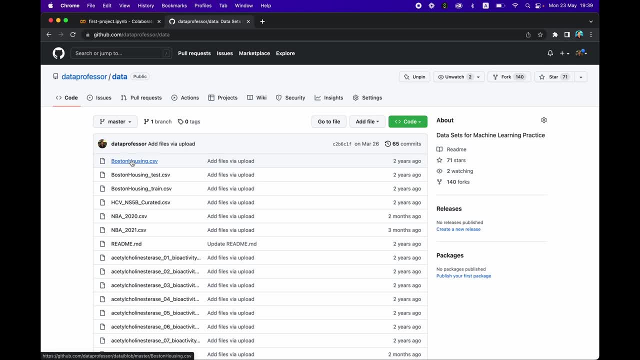 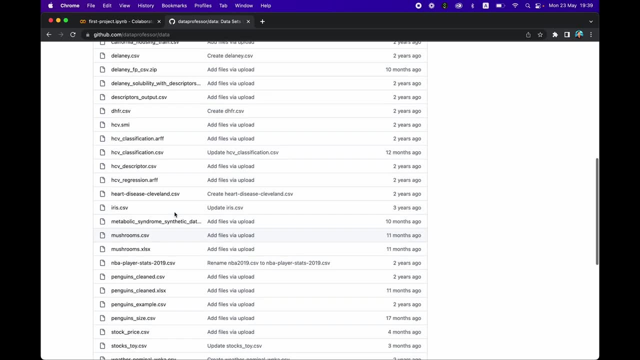 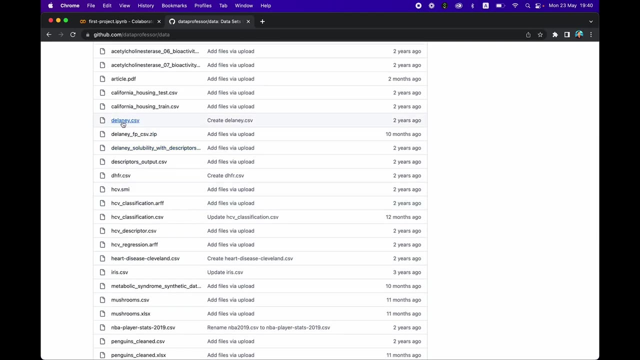 data, click on it And then there's a lot of data sets here that I have compiled over the years as a content creator. So a reasonably simple and unique data set that I would like to use here is the Delany data set, And I think it's this one. Let me have a look. 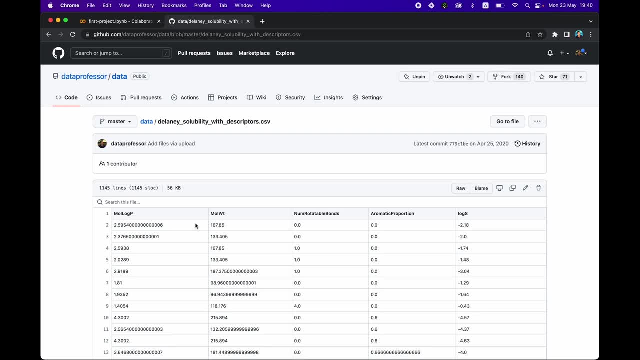 Okay, so this is a data set of the solubility of molecules And they are the fact that they are crucial for biologists and chemists in determining whether a molecule is soluble in water or solvent and whether they will be good drug candidates. And so let's have a. 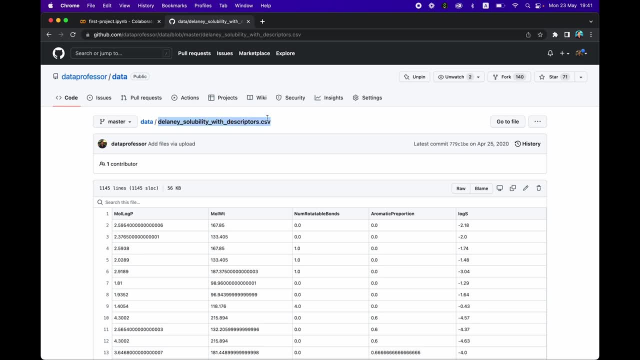 look here you can see that the data set here is in the format of a CSV And essentially it is a comma separated value file. So if you click on the raw link here, you're going to see the native file. let me zoom in And you're going to see that. 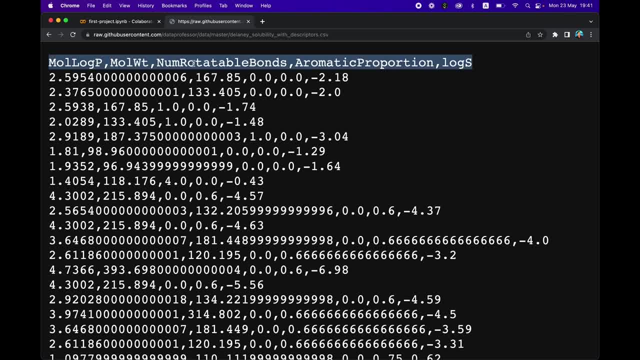 the first row will comprise of the names of the columns, And each word that you see here is the name of the column and it represents a single cell, and then you have the comma to separate it, And therefore the first word here and the second word here and the third word, and etc. 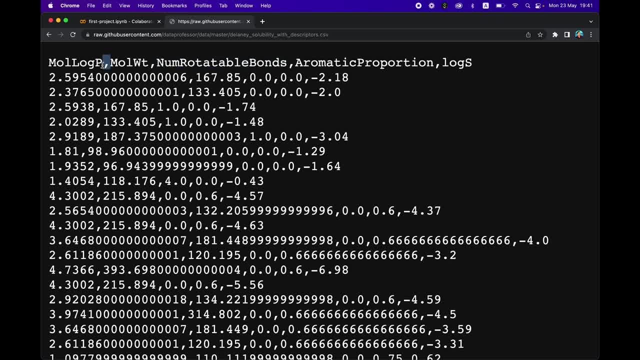 are separated by commas, Therefore. hence they are called comma separated values, because the comma will separate the values. And so here, how many columns do we have? we have one, two, three, four, five. so we have five columns, and then we have, correspondingly, from lines two until the end of: 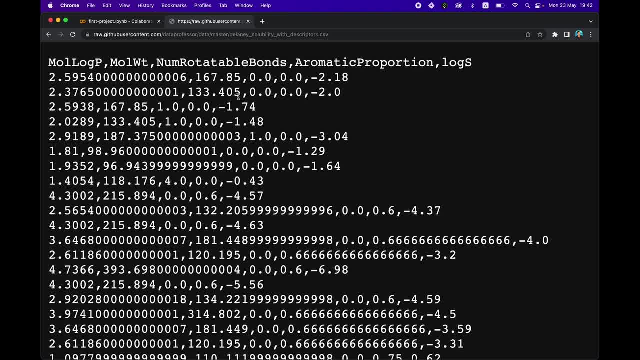 the file. they represent our data sets, And so typically what I like to do is I normally will put the y variable, or the dependent variable, or you could also call it the output variable or the y variable, So there's so many names for it, And so they are the variable that you want to predict. 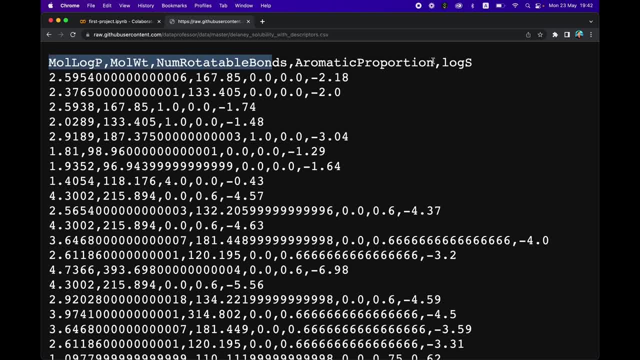 as a function of the x variables, which is the variable that you want to predict. as a function of the x variables, which is the variable that you want to predict. as a function of the x variables, which is the variable that you want to predict. as a function of the x variables, which are the ones. 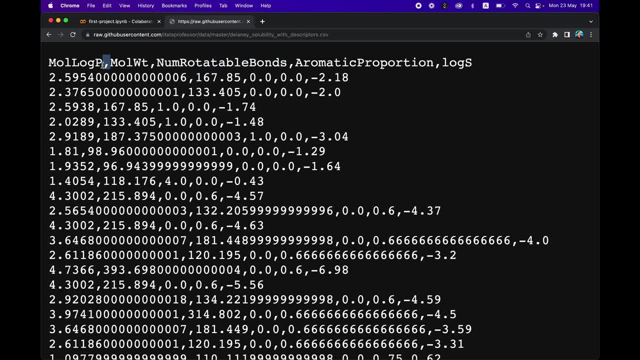 are separated by commas, Therefore. hence they are called comma separated values, because the comma will separate the values. And so here, how many columns do we have? we have one, two, three, four, five. so we have five columns, and then we have, correspondingly, from lines two until the end of: 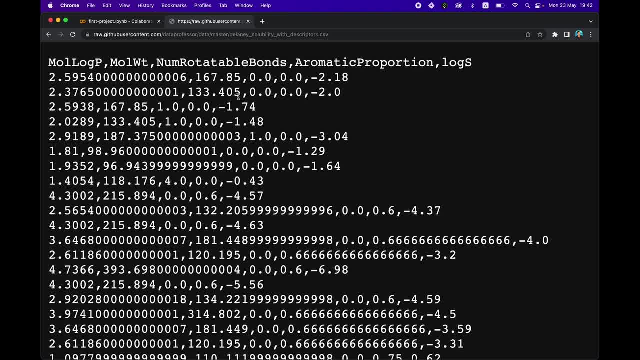 the file. they represent our data sets, And so typically what I like to do is I normally will put the y variable, or the dependent variable, or you could also call it the output variable or the y variable, So there's so many names for it, And so they are the variable that you want to predict. 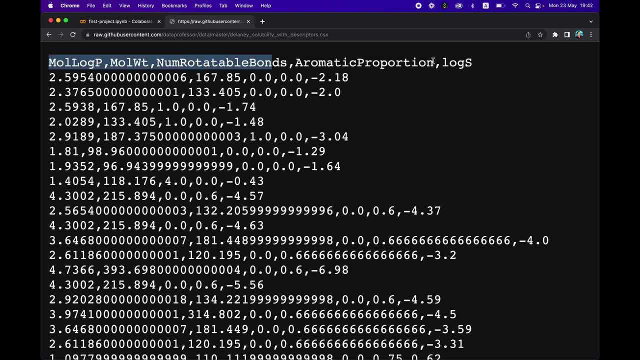 as a function of the x variables, which are the variables that you want to predict. as a function of the x variables, which are the variables that you want to predict as a function of the x variables, which are the variables that you want to predict as a function of the x variables, which are the 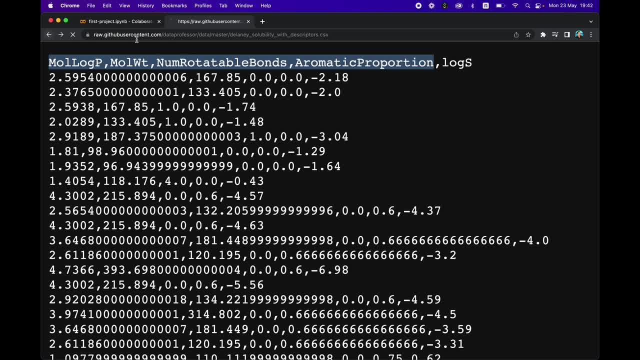 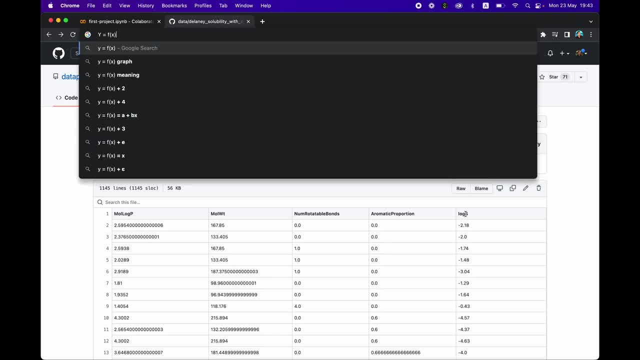 ones here that are highlighted. So you might be familiar with the equation: of y equals to f, of x, right? So y is the last column here. the y variable equals to the function of x, So we have several x here. So it is a multivariate analysis, Okay. 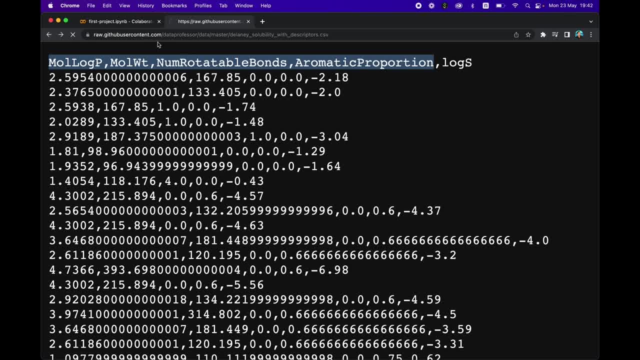 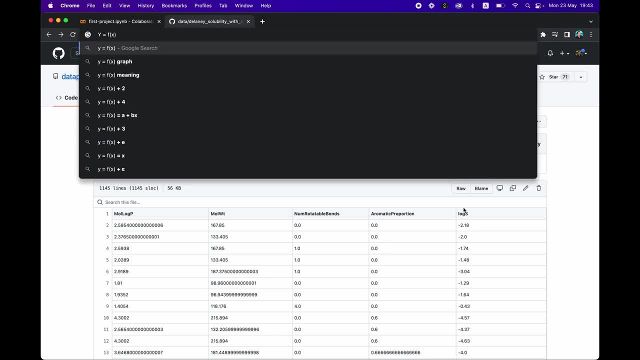 here that are highlighted. So you might be familiar with the equation: of y equals to f, of x, right? So y is the last column here. the y variable equals to the function of x, So we have several x here. So it is a multivariate analysis. Okay, so what we want to do is we're going to import. 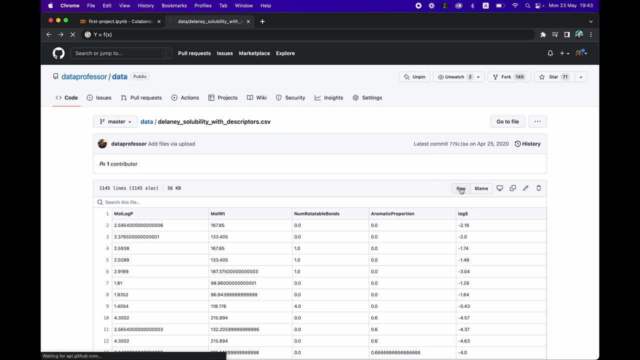 this particular data set. So I'll click here on the raw link And then I'll click here in the address bar I'm going to say import this particular data set And then I'll say import the addresplot And then I'll say import this particular data set. So I'll click here on the raw link And 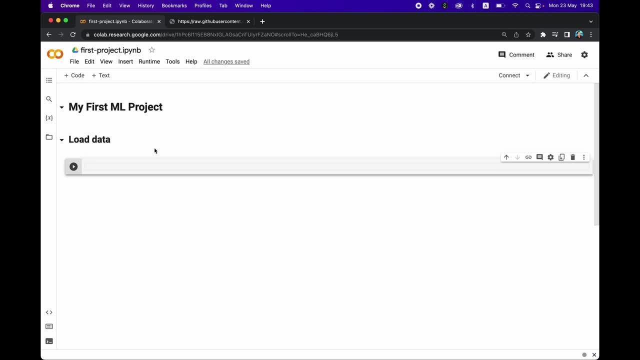 bar, right click and click on copy, and now we're going to read in the data set into the jupyter notebook. so the python library that we're going to use in order to do that is called pandas, and so we're going to import it as follows: import pandas as pd. so pd is sort of a alias for the. 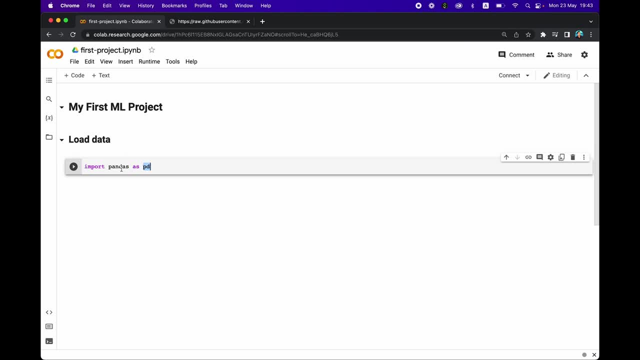 pandas library. so from here on, we're going to call pandas as pd, as mentioned here, and then we're going to read in the data set in the csv format and then we're going to assign it to a variable called df, and df is an acronym for a data frame. so let's do it. we're going to type in pd because 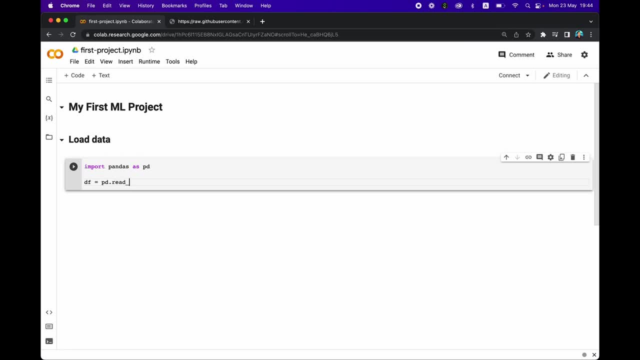 we want to use pandas and then we're going to use the function from pandas library called read csv, and then ask the input argument, which is inside the parenthesis. we're going to type in the address of the file, or you could also type in the file name, so you can see here that 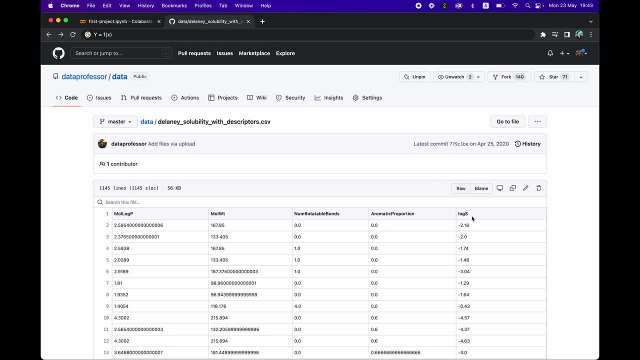 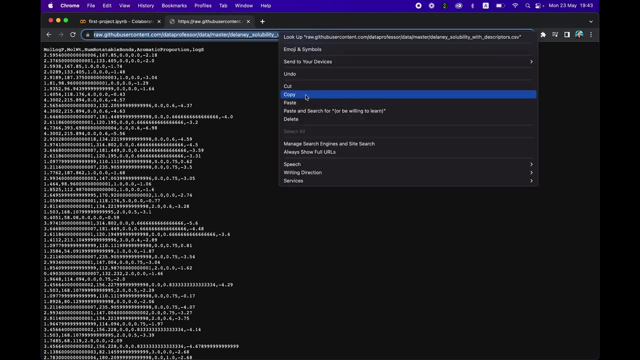 so what we want to do is we're going to import this particular data set. So I'll click here on the raw link And then I'll click here in the address bar, right click and click on copy, And now we're going to read in the data set into the Jupyter. 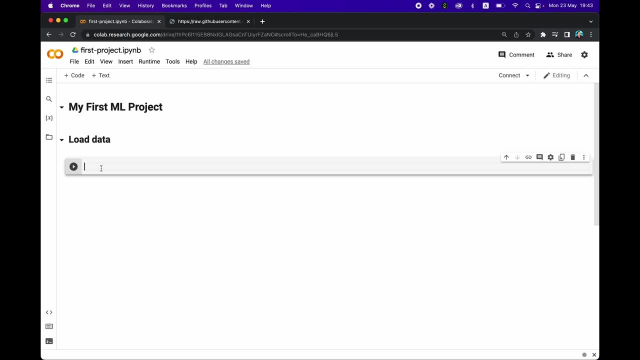 notebook. So the Python library that we're going to use in order to do that is called pandas, And so we're going to import it as follows: Import pandas as PD. So PD is sort of a alias for the pandas library. So from here on we're going to call pandas as PD, as mentioned here, And then 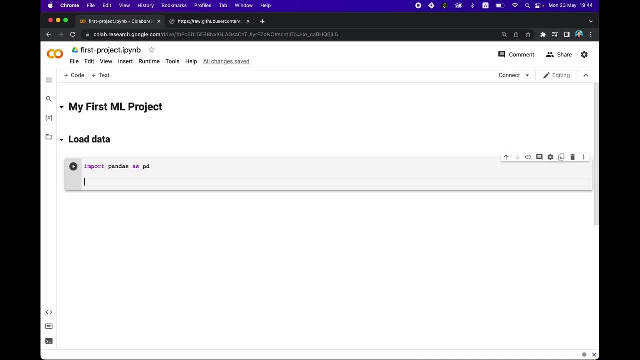 we're going to read in the data set in the CSV format And then we're going to assign it to a variable called DF, And DF is an acronym for data frame. So let's do it. we're going to type in PD because we want to use pandas, And then we're going to use the function from pandas library. 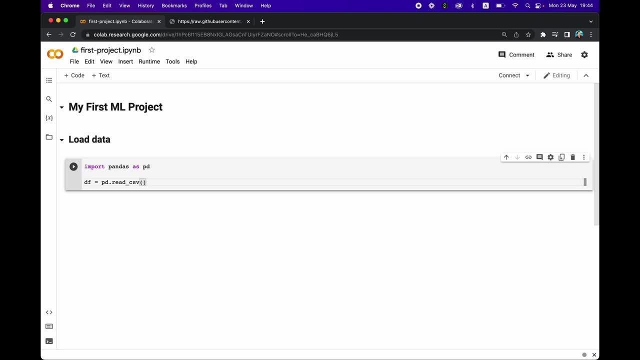 called read CSV And then, as the input argument, which is inside the parentheses, we're going to type in the address of the file, or you could also type in the file name, So you can see here that's the file name. And then we're going to type in the address of the file name, So you can. 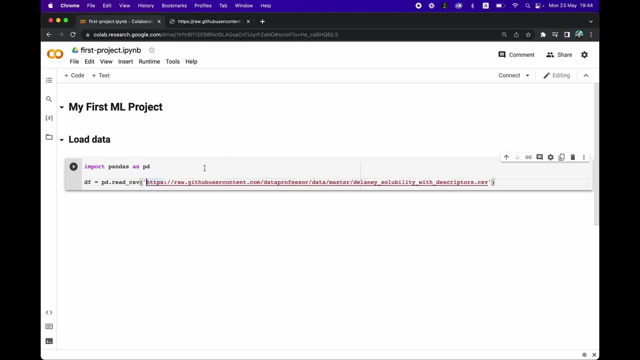 that we could, directly within the data set from the URL that we had just copied from GitHub. And so let's do it. And then, once read in, we're going to print it out by typing in DF, And I'm going to hit on the play button here to run the cell, And so, because it is just loading, you're going to see. 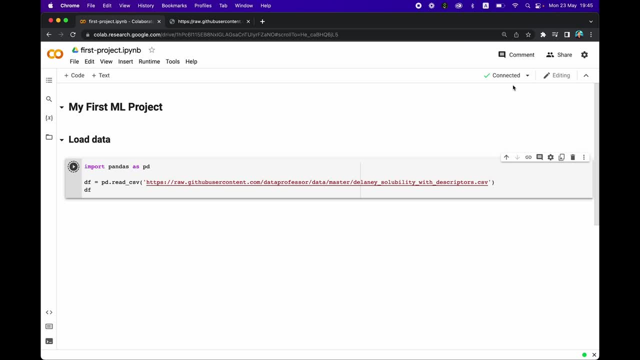 that it's connecting, So it's going to take a short moment. it's initializing and now it's connected, And now we're ready. Now you can see the RAM and the disk that are assigned to this particular cloud computing unit that we have here in the notebook. Alright, and so once you have run the 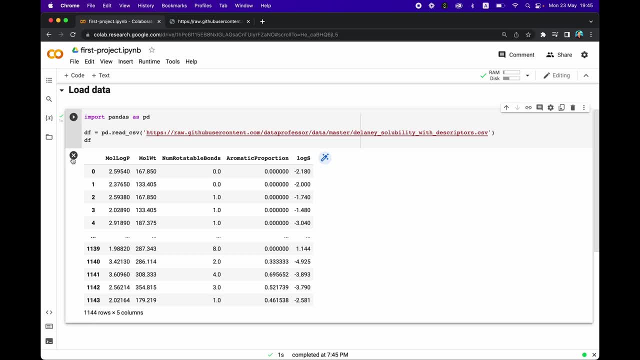 cell. you're going to see the output which is right here, which you could also close if you don't want to see it again, or you could play it again to display it again. So we're going to see the contents of the CSV file in a tabular format here. you're going to see here that the first 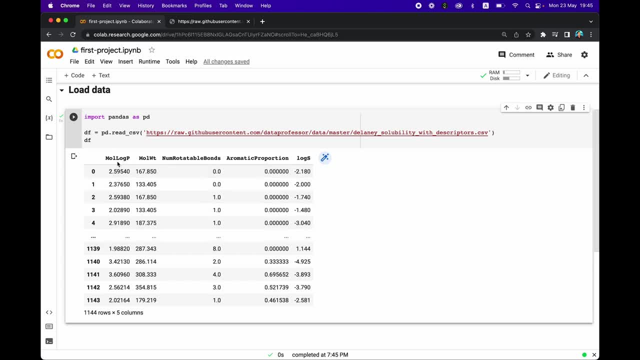 column here that you see is the index number. So officially it's not a column, So it is the index name And here you're going to see the column. So you're going to see the index number. So you're going to see the columns. mol-log-P- mol-weight năm-rotatable-bonds- i-eromatic. 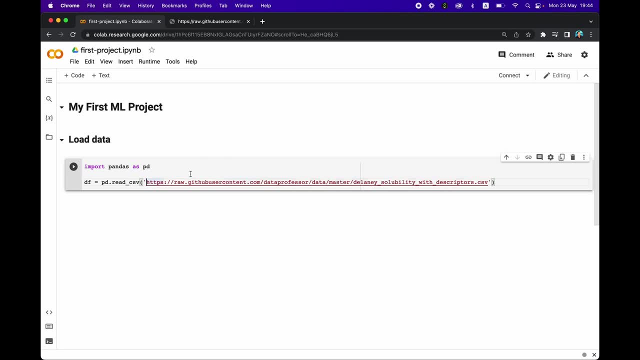 we've found the format and we need to colonialize our code. so if we're going to do this in pd, we're going to. we could directly read in the data set from the URL that we had just copied from GitHub, And so let's do it And then, once read in, we're going to print it out by typing in DF And I'm going to. 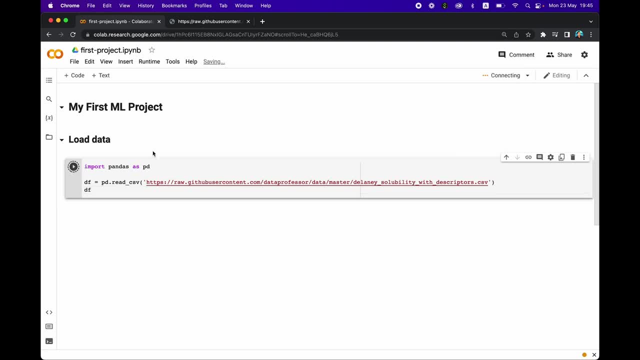 hit on the play button here to run the cell And so, because it is just loading, you're going to see that it's connecting, So it's going to take a short moment. it's initializing and now it's connected And now we're ready. Now you can see the RAM and the disk that are assigned to this. 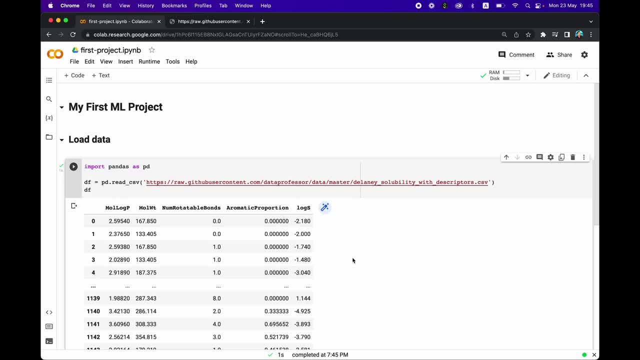 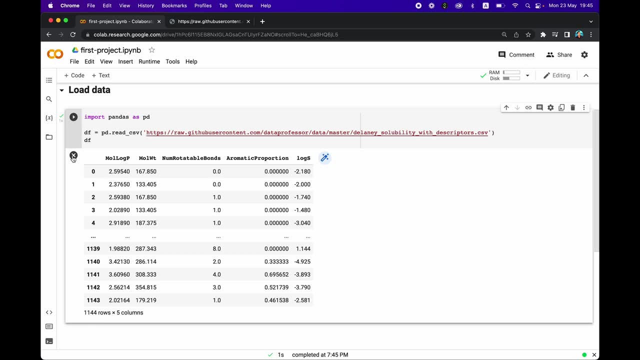 particular cloud computing unit that we have here in the notebook. Alright, and so once you have run the cell, you're going to see the output which is right here, which you could also close if you don't want to see it again, or you could play it again to display it again. So we're going to see. 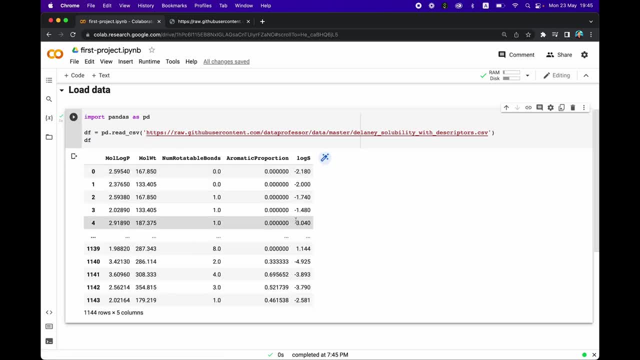 the contents of the CSV file in a tabular format. here you're going to see here that the first column here that you see is the index number. So officially it's not a column, So it is the index name. And here you're going to see the index number. And here you're going to see the index. 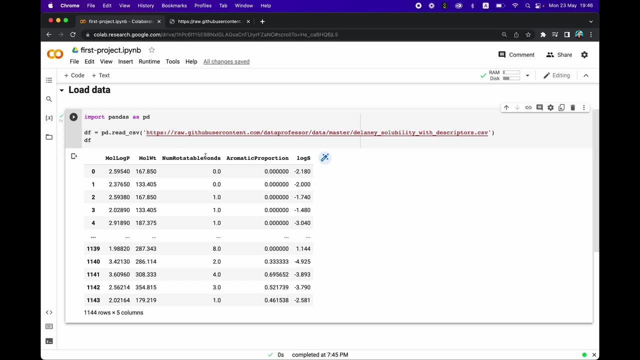 number, And here you're going to see the columns: mo, log p, mo, weight num, rotatable bonds, aromatic proportion. So these four variables represent the x variables, And so when we build a machine learning model to predict the y variable or the log s, and therefore log s is equal to the- 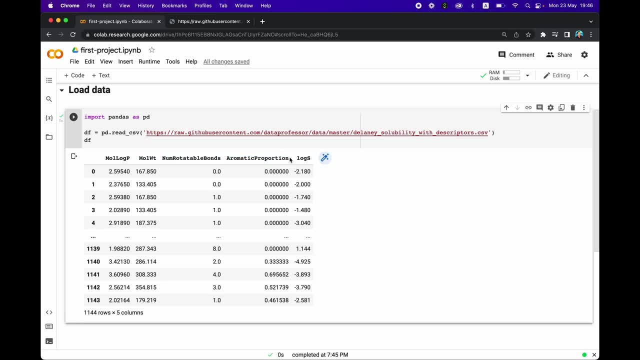 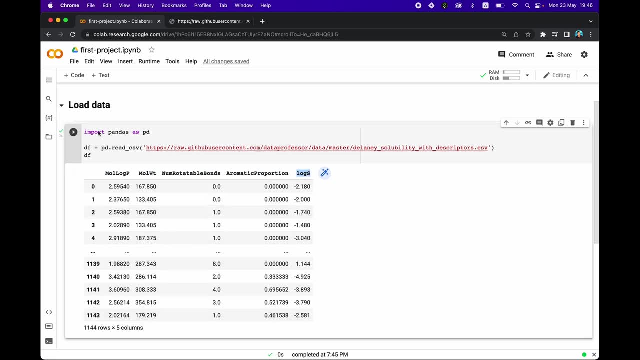 function of all of the x variables here. So in other words, we're going to use the four variables here to make a prediction on the log s variable. Okay, and so the next thing that we want to do here now is that we want to split the data frame into the x and into the y, And so let's do the. 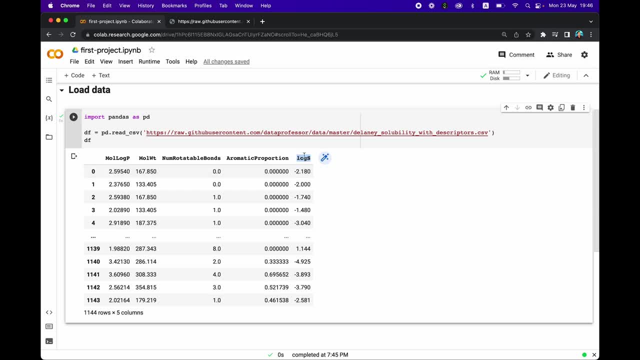 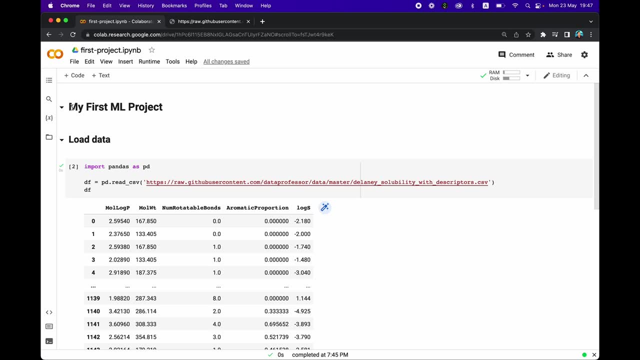 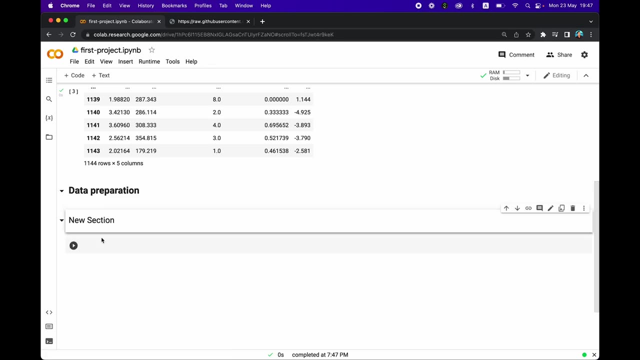 most simplest thing is to obtain the y variable. So let me show you. I'll create some text cell, I'll make it bold: data preparation. we have here the first level, here one hash symbol. we have here two hash symbol. this is make it two hash symbol. let's make this three, because we want. 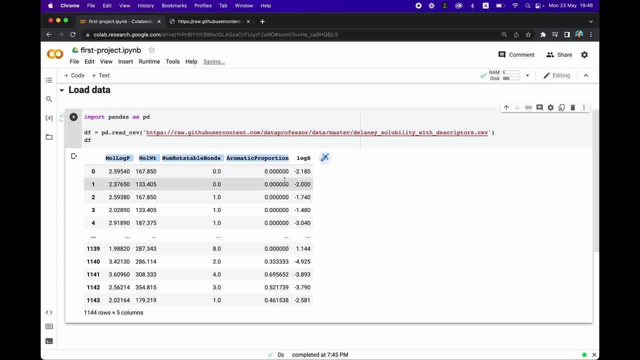 proportion. so these four variables represent the X variables, And so right here we talk about this divideBoy, right here. And so when we build a machine learning model to predict the Y variable or the log S, and therefore log S is equal to the function of all of the X variables here. 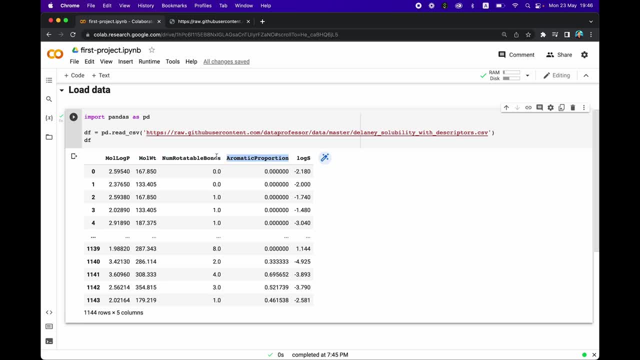 which traditionally, by default, is different from what these other satisfying بالs would be the first element in this model, but these values are called log and those elements are the variables where the elements come into play. So, in other words, we're going to use the four. 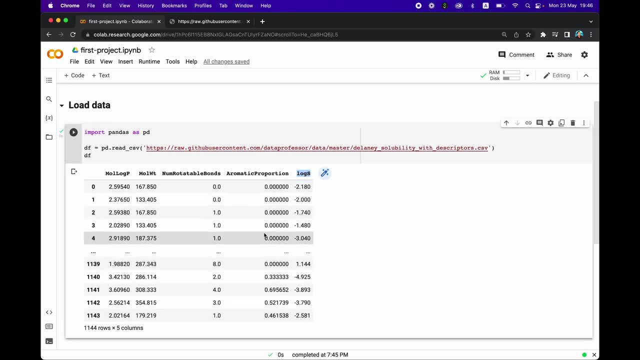 variables here, to make a prediction on the log S variable. Okay, and so the next thing that we want to do here now is to go to the première y bar here and by doing a predictive, that, Peregos, is that we want to split the data frame into the x and into the y, And so let's do the most simplest. 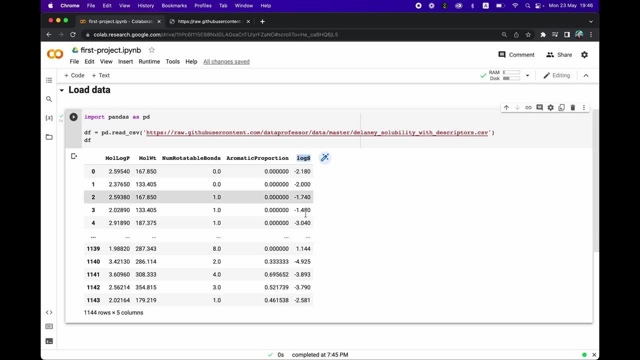 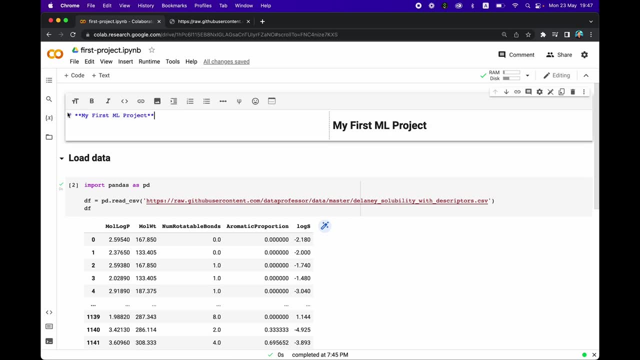 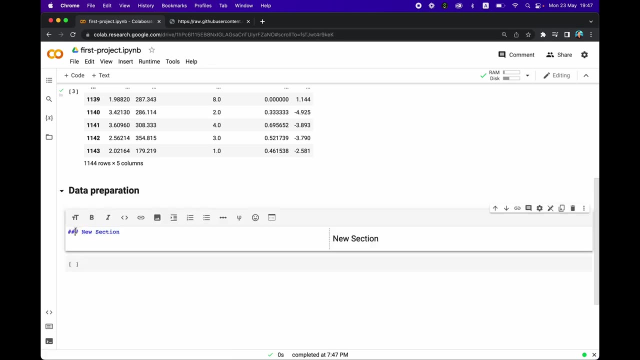 thing is to obtain the y variable. So let me show you. I'll create some text cell, I'll make it bold: data preparation. we have here the first level, here one hash symbol. we have here to hash symbol. this is make it to hash symbol. let's make this three because we want it to be a subsection of 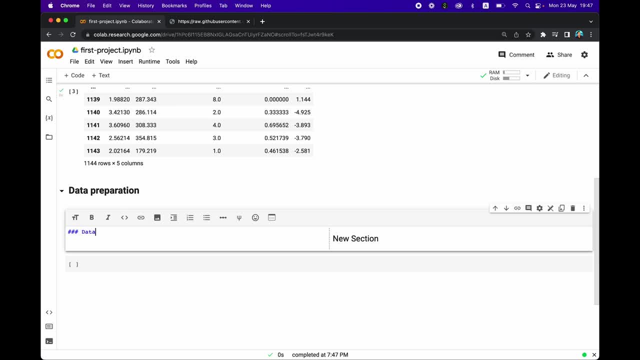 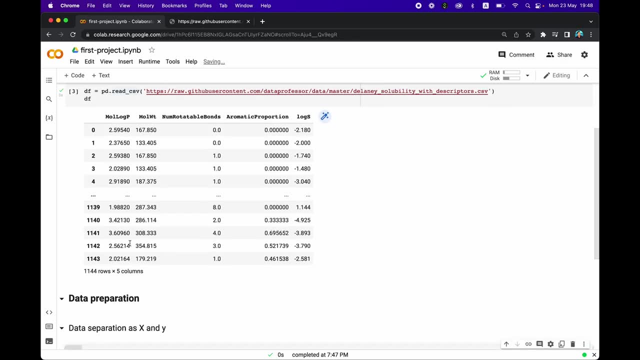 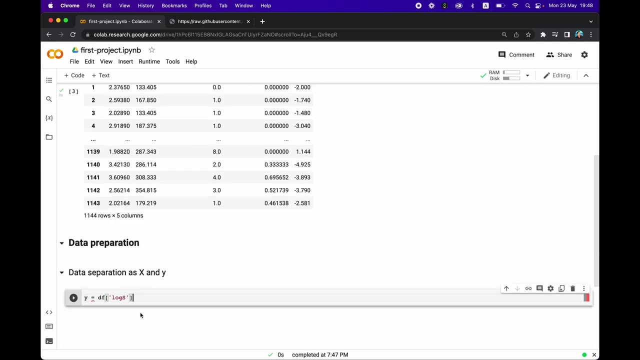 this one, And so we're going to call this data split, data separation or data separation as x and y. Okay, and so we're going to create the y and we're going to type in the F and the name of the last column here is log s. So that's how we're going to get the y and let's see, okay, and these 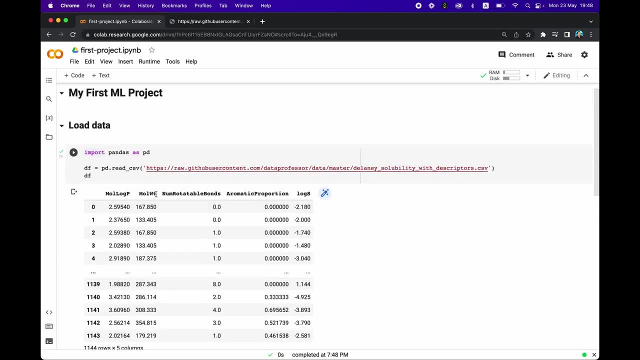 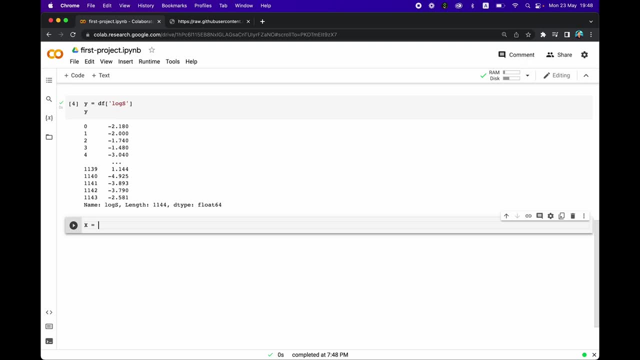 are the y log s. And now we want to get only the x variables. So we want to remove the log s. So we're going to do that type in: x equals to df, dot, drop parentheses. And then we're going to see we want to draw a log s and we want to have 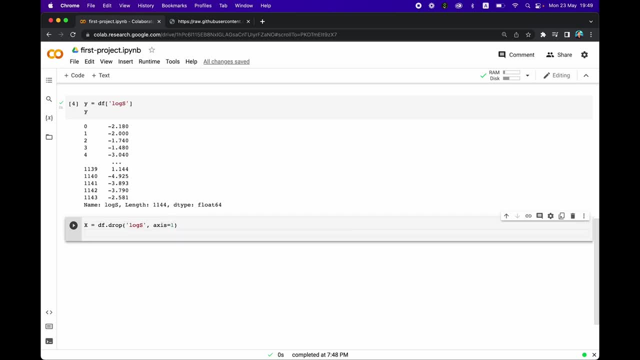 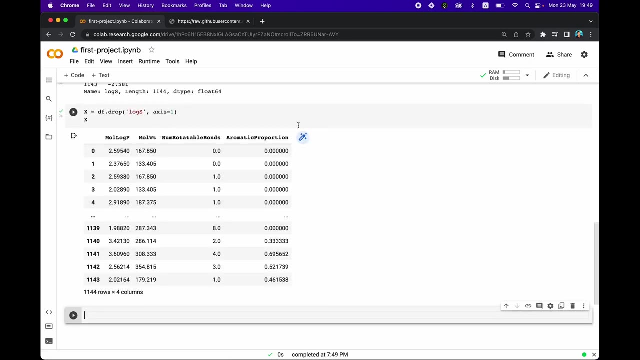 it access equals to one, because access equals to one will allow the drop function to work with the data as column mode. However, if you use access equal to zero, it will work it in the row mode. Let's see if that's correct. It is correct. you see that the log s now gone and that we have four. 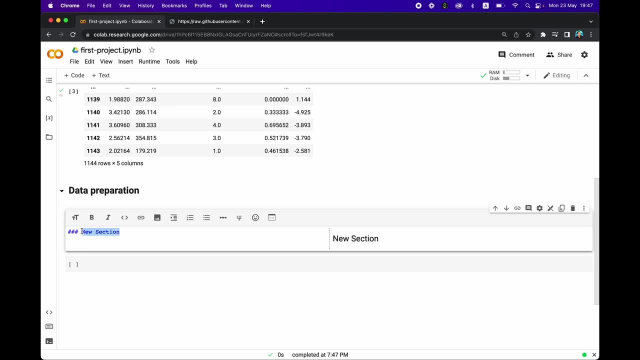 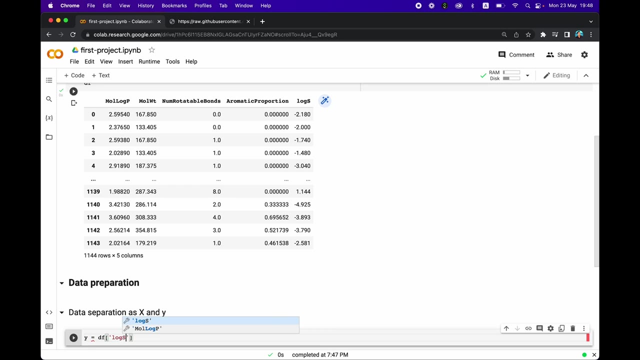 it to be a subsection of this one, And so we're going to call this data split, data separation, or data separation as x and y. Okay, and so we're going to create the y and we're going to type in df, And the name of the last column here is log s. So that's how we're. 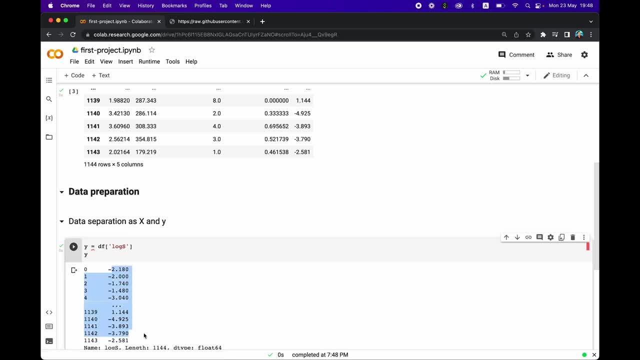 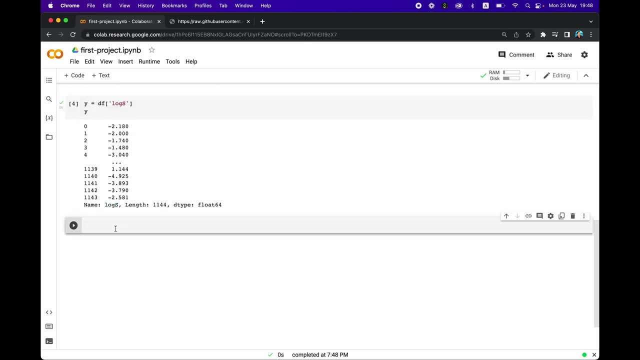 going to get the y And let's see, Okay, and these are the y log s. And now we want to get only the x variables. So we want to remove the log s. So we're going to do that type in: x equals to df dot. 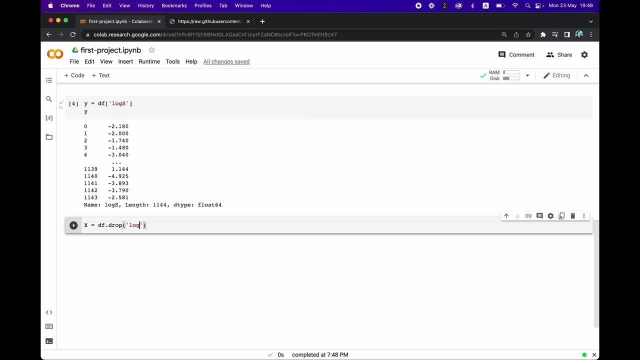 drop parentheses. And then we're going to see we want to draw log s and we want to have x equals to one, because x equals to one will allow the drop function to work with the data as column mode. However, if you use x is equal to zero, it will work it in the row mode. Let's see if that's correct. It is correct. 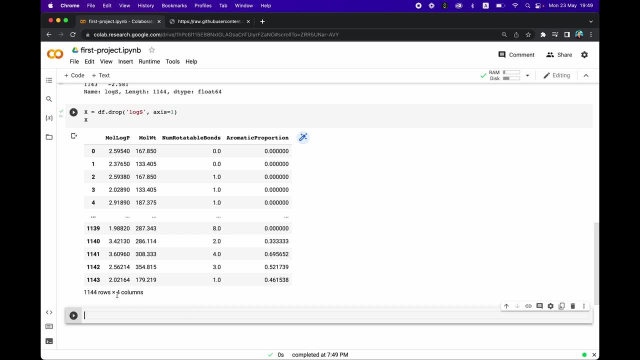 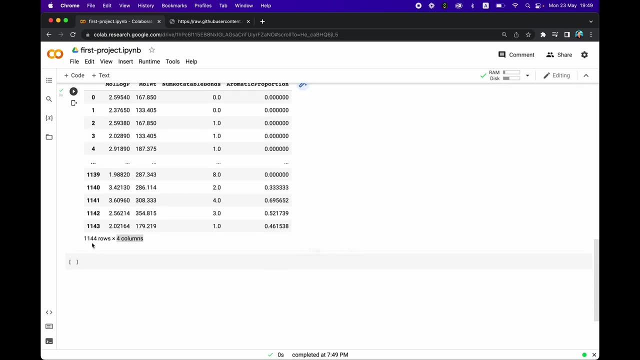 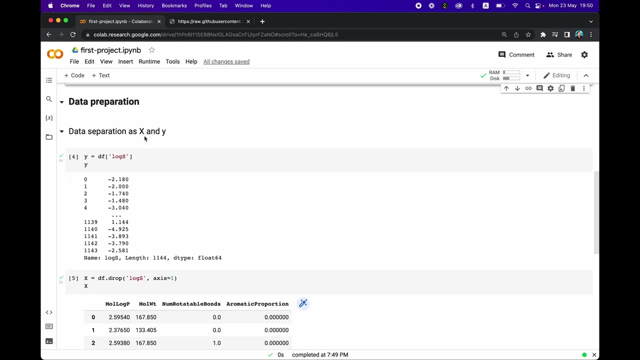 you see that the log s now gone and that we have four columns here And prior to that we have five columns, So the number of rows remain the same At 1144.. So now we have x and y in the separated form. So the next thing that we want to do is we're. 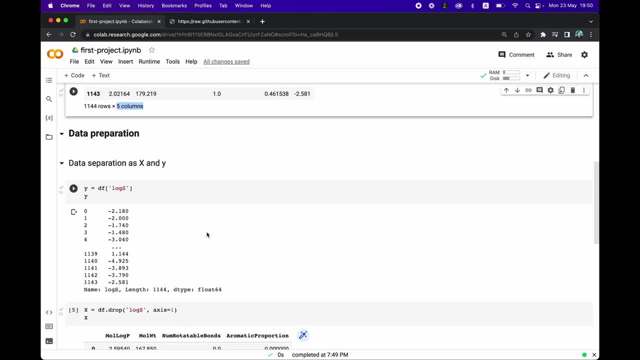 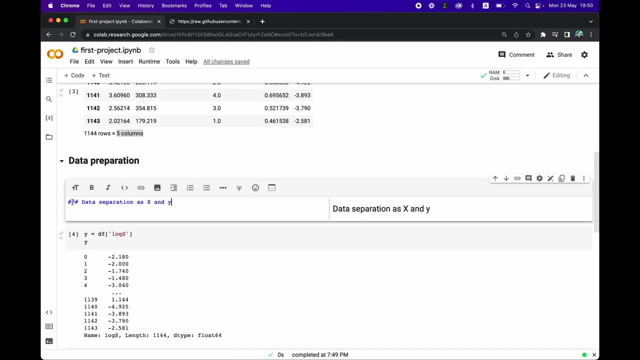 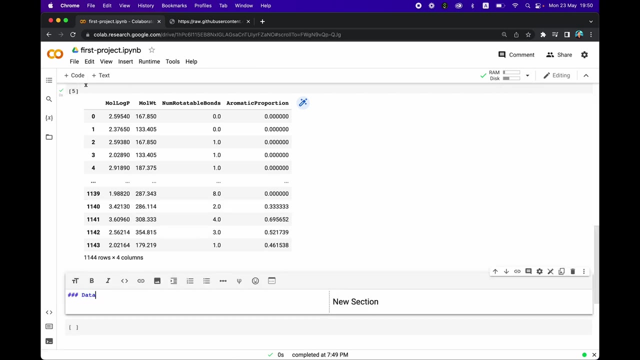 going to split the data set. we're going to split it as the training set and the testing set, So let's do it. So remember how many we need. we need three hashed symbols here. So we're going to add text cell, click it three times and then type data splitting And we're going to use the scikit learn. 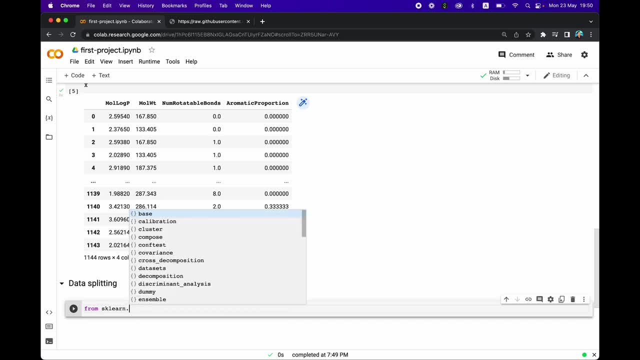 package for that. So you want to type in from sk learn dot model underscore selection, And then you want to import the train test split, train test split. And now we're going to type in x, train x test, y, train y test equals to train test splits x and y, And we're going to have the test size to be: 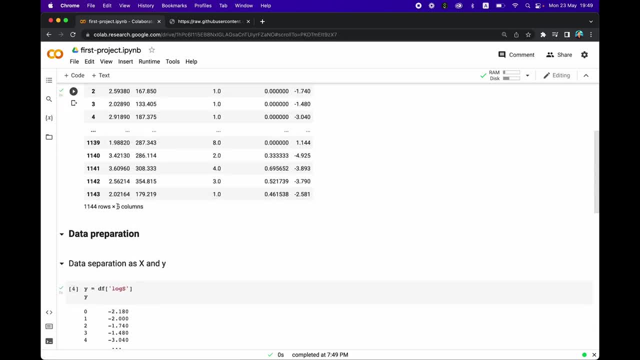 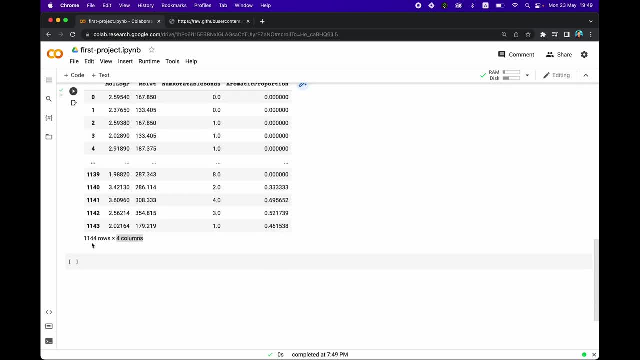 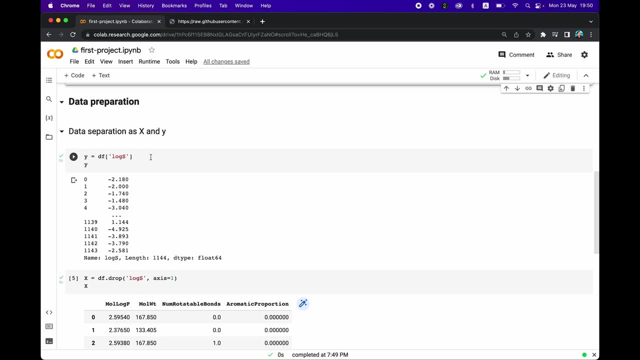 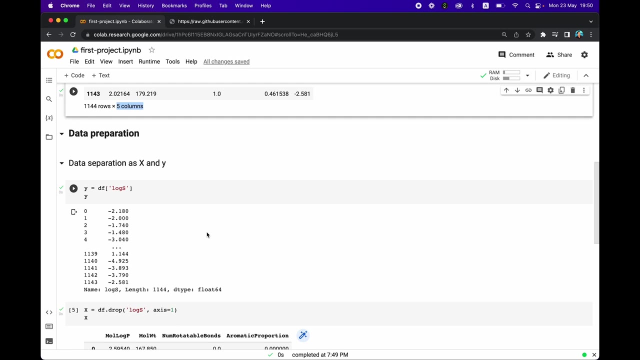 number of rows remain the same at 1144.. So now we have x and y in the separated form. So the next thing that we want to do is we're going to split the data set. we're going to split it as the training set and the testing set, So let's do it. So remember how many we need. we need three hash. 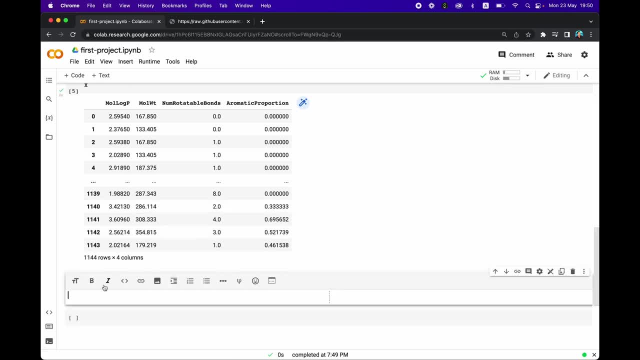 symbols here. So we're going to add text cell, click it three times and then type the data data splitting And we're going to use the scikit learn package for that. So you want to type in from SK learn dot model underscore selection And then you want to import the train test split train. 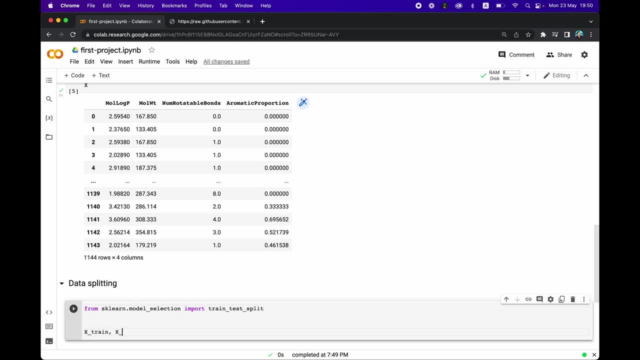 test split. And now we're going to type in x- train x test, y, train y test equals to train test splits x and y, And we're going to have the test size to be 0.2.. And let me see, I want to have the random. 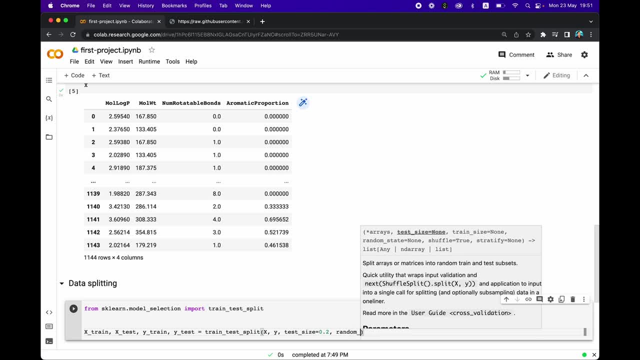 state to be assigned a specific number so that every time I run the code cell I will get the same data split. So we're going to have random state equals to, let's say, 100.. And now we're going to run it. So we should now have four new variables here. And let's have a look at the x. 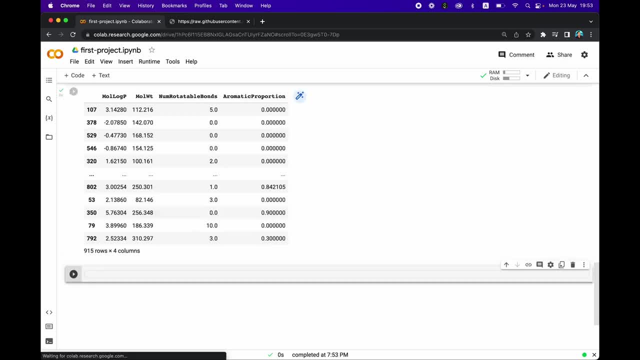 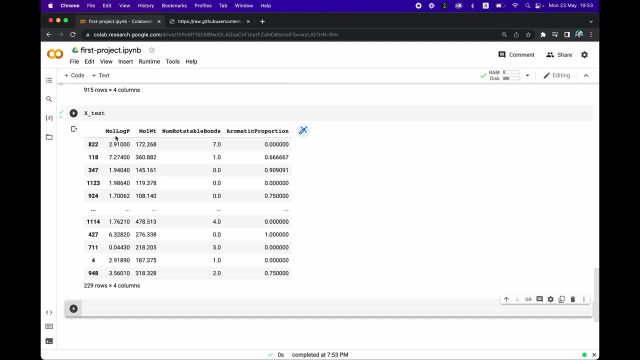 train And we see that we have 915 rows and four columns. let's have a look at x test. We have 229 rows And also four columns. So x tests or x train will come from the x variable. So we started out with: 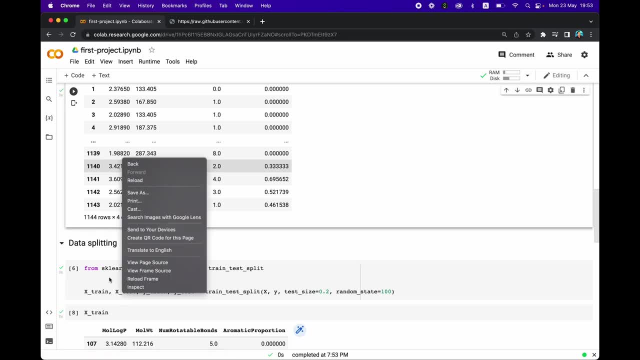 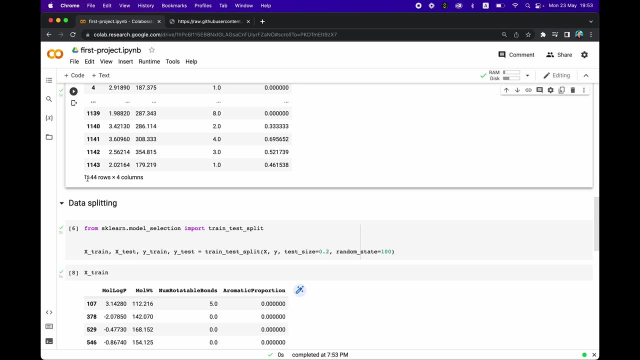 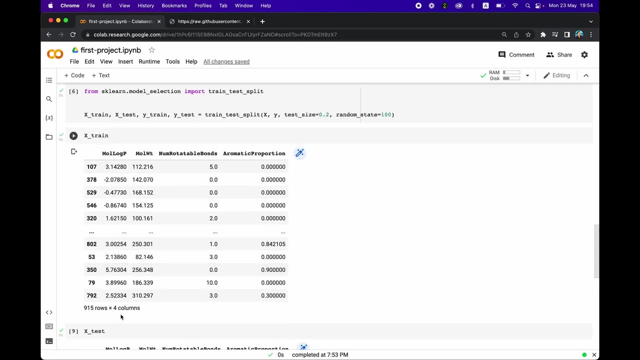 1144.. And so 80% of 1144 is 915 and 20% of 1144 is 229.. And so the training set here will have 80% of the data and the x test here, or the test set. 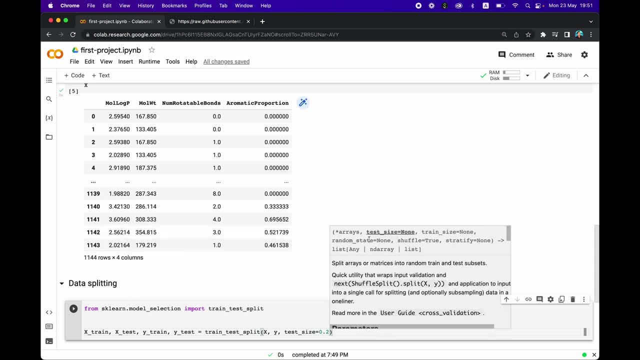 0.2.. And let me see, I want to have the random state to be assigned a specific number so that every time I run the code cell I will get the same data split. So we're going to have random state equals to, let's say, 100.. And now we're going to run it. So we should now have four new. 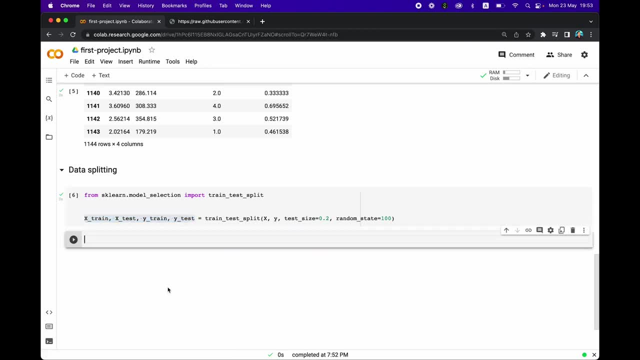 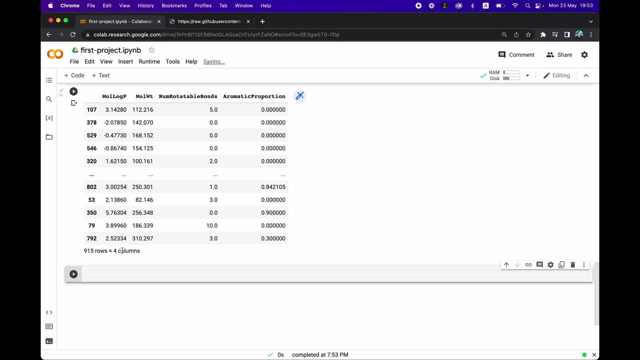 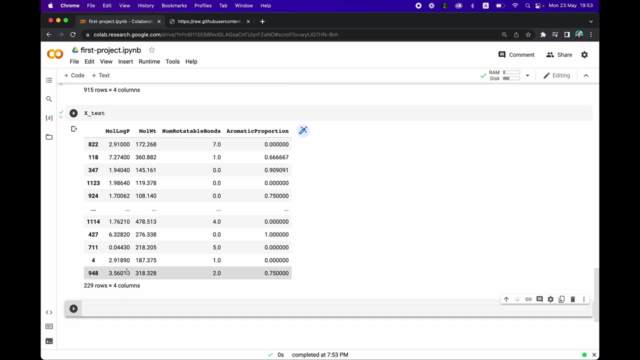 variables here. And let's have a look at the x train And we see that we have 915 rows and four columns. Let's have a look at x test: We have 229 rows and also four columns. So x tests. 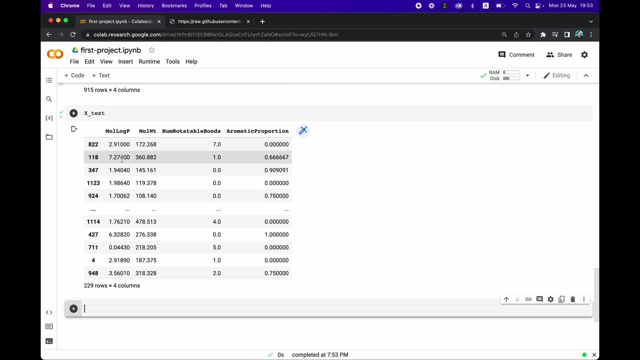 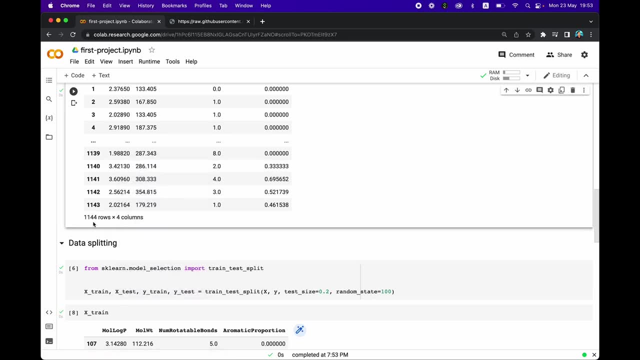 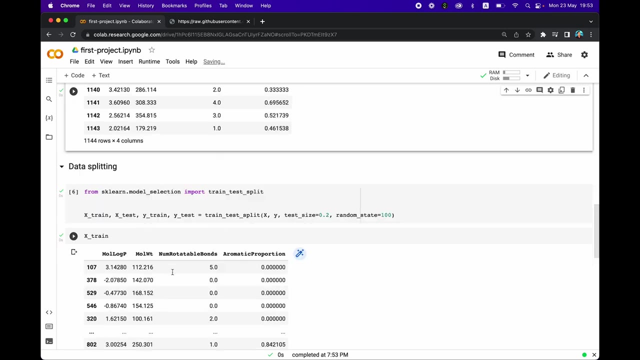 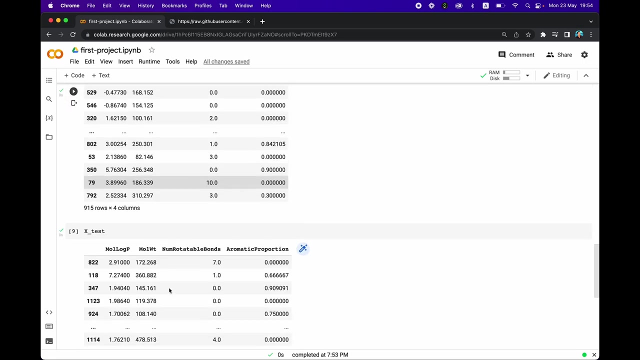 or x train will come from the x variable. So we started out with 1144. And so 80% of 1144 is 915. And 20% of 1144 is 229. And so the training set here will have 80% of the data and the x test here. 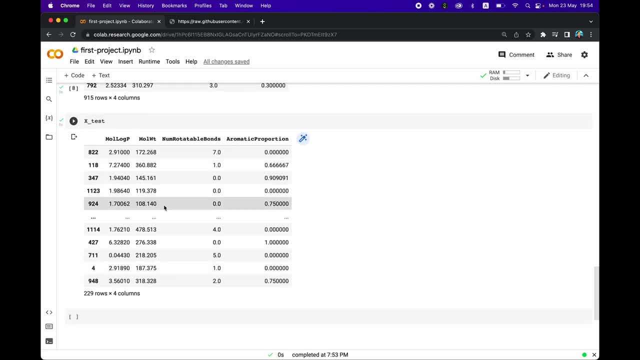 or the test set will have 20% of the data, And I actually written a blog post about this particular topic of building your machine learning model in Python using scikit learn, And I've drawn several illustration explaining about the data split. So let me go and let me show you- And it's this article- how to build a machine learning model. 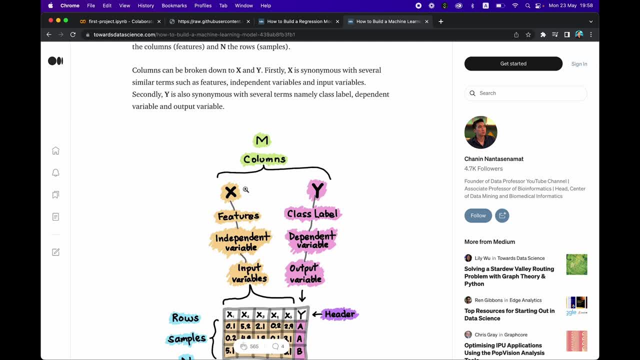 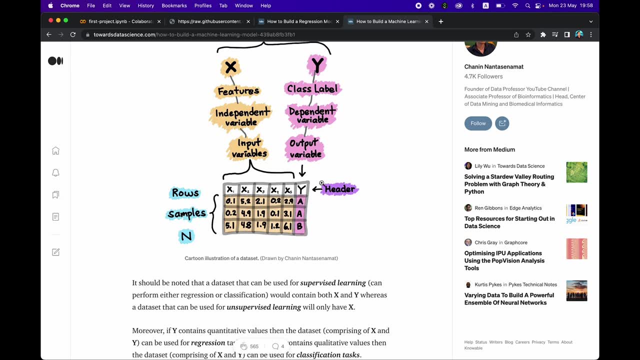 a visual guide to learning data science. So here we have the x and y that I mentioned already, And I've color coded here as orange and pink for the x and y, right, So you can see that I've already screened it in Python. So let me go into Python and change the. 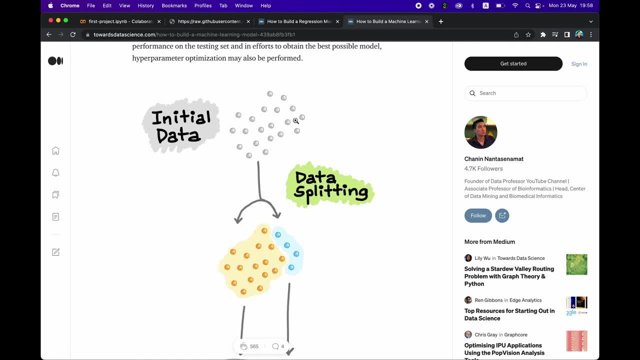 code right here And you can read So how I use Python here to show you a test setting a little bit better. so when it comes to the reminded way for a particularядi, you see that you're at the yeah printing- awesome. And then you get a test setting, which is the learning model. 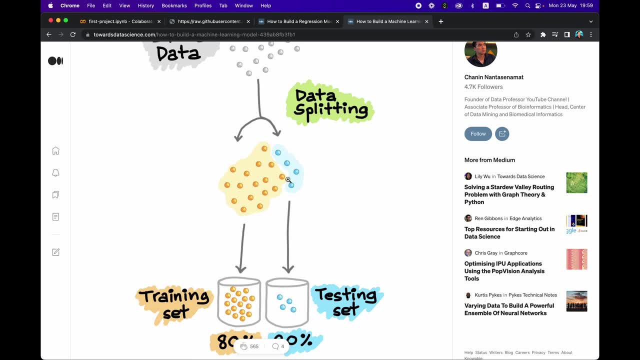 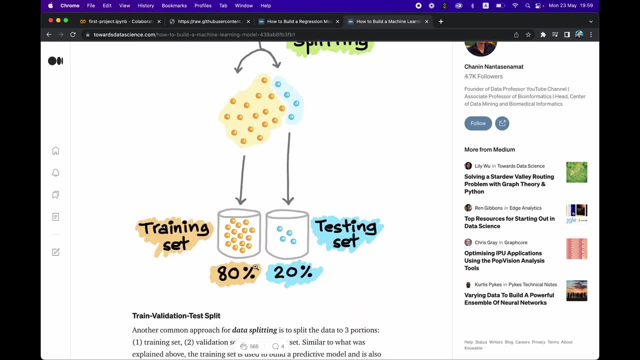 but you can get a strongeruh. As you can see in Katherine context, you can find this information that you can get at any time and that it is with blocks inside array function. That means you can simply put one passpoints in this general setting and now look at this data set. 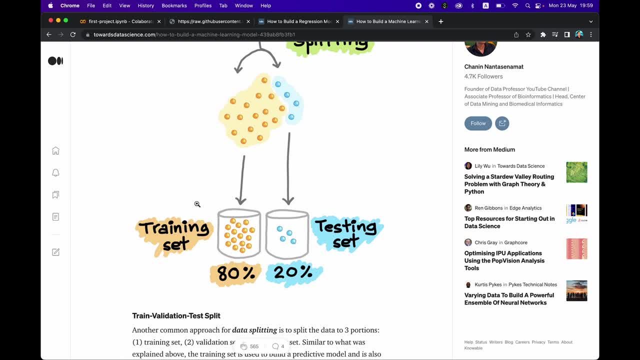 once again. you're getting into a training Set dialog part and so on. you can enter this data, Data stuff to be the training set here And then we want to use the testing set to serve as sort of a unknown data that you want to test training set for. You want to evaluate whether the model that you have built using the training set. 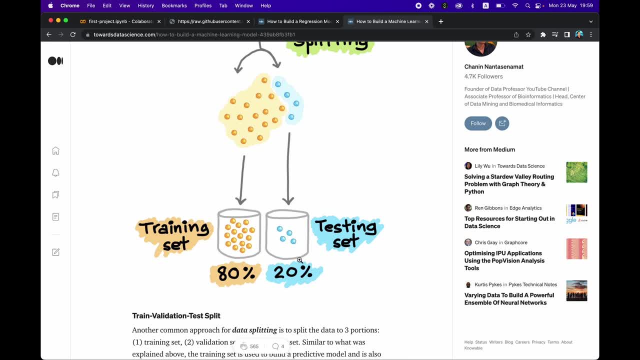 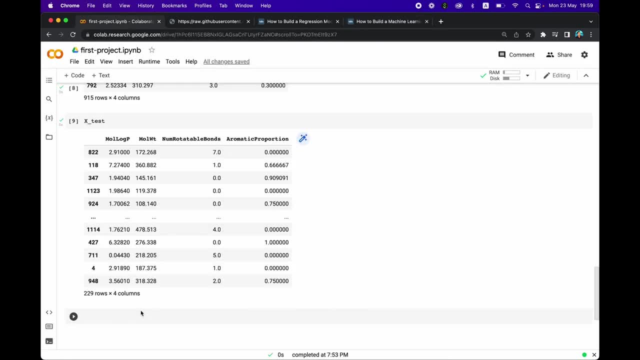 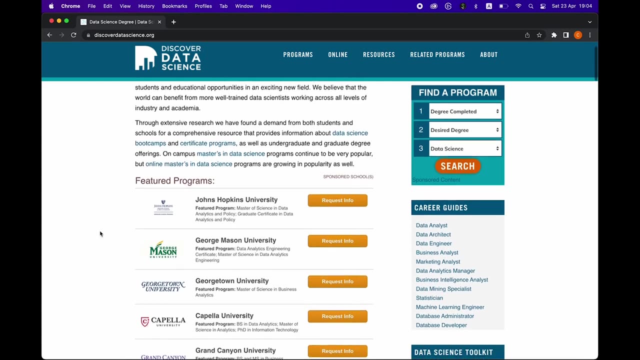 whether it performed in a robust manner against an unknown data that you simulate using the testing set. Okay And so, before continuing further, a quick word from our sponsor, And so a short message from our sponsor: Discover Data Science powered by Wiley, which is the premier information hub. 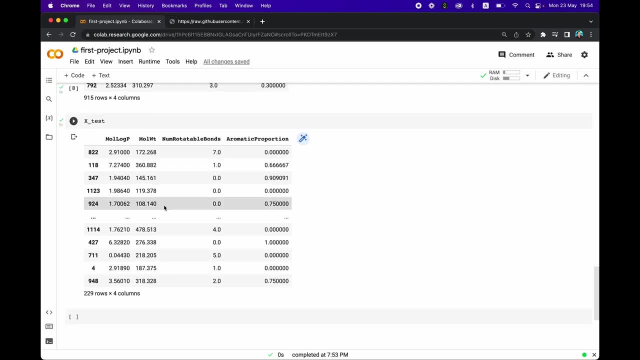 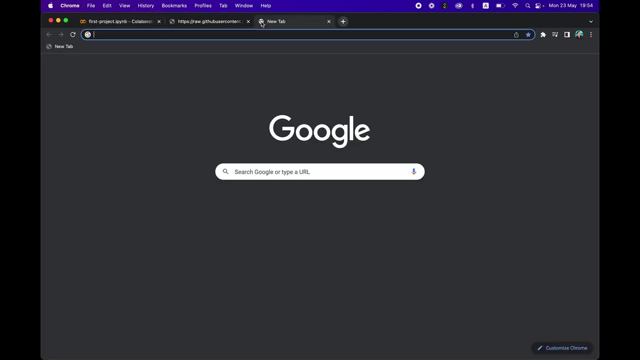 We'll have 20% of the data, And I've actually written a blog post about this particular topic of building your machine learning model in Python using scikit learn, And I've drawn several illustration explaining about the data split. So let me go and let me. 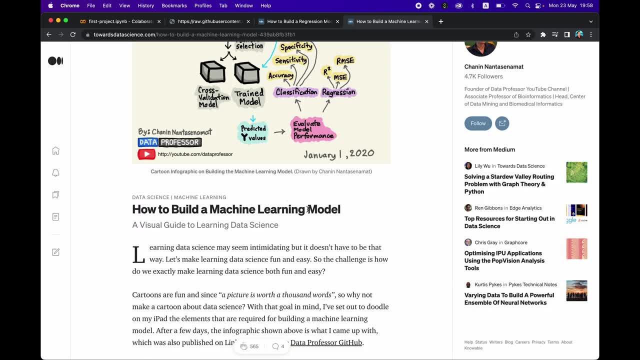 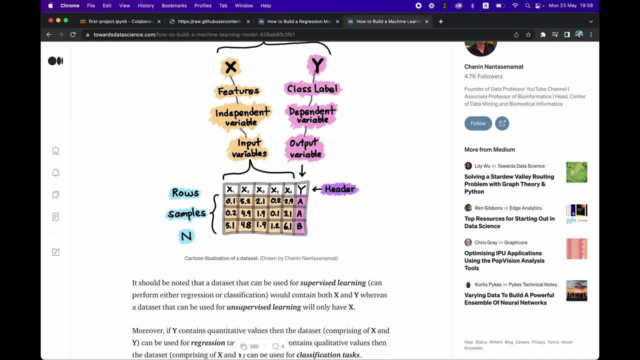 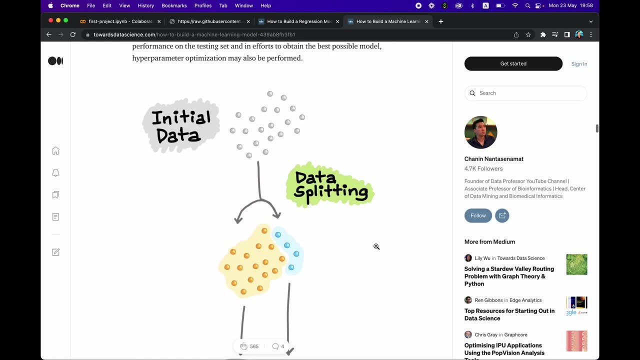 show you- and it's this article- how to build a machine learning model, a visual guide to learning data science. So here we have the x and y that I mentioned already And I've color coded as orange and pink for the x and y respectively. scroll down And here here's the data split. So 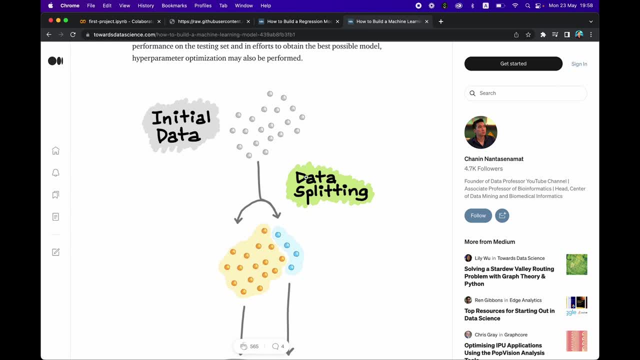 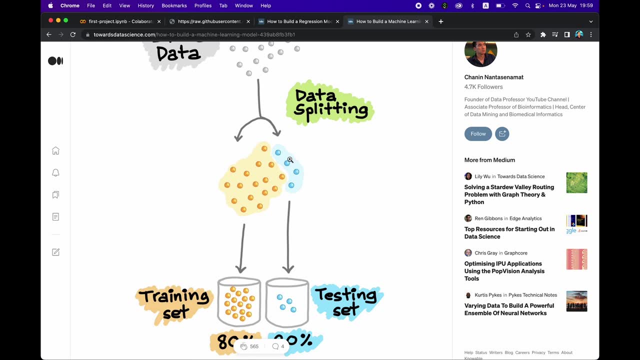 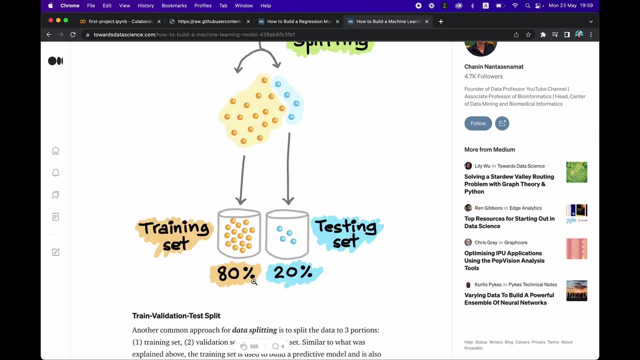 here you have the initial data sets And then you perform data splitting, where 80% of your data will go into a container that you call the training set, And then the remainder, or the 20%, will go to a container that you call the testing set, And the typical ratio is 80 to 20% for the 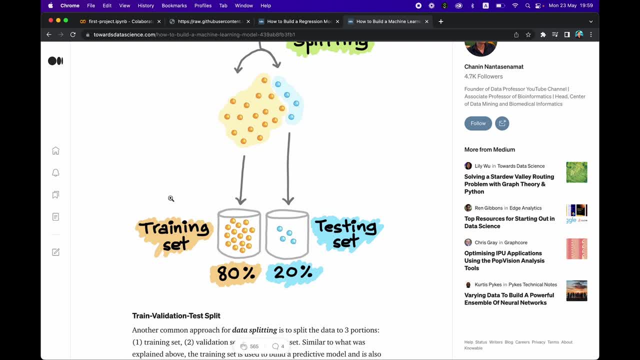 training set and the testing set. So typically the training set is 80 to 20% for the training set And the testing set. So typically we use the training set to build a model And then we want to use the testing set to serve as. 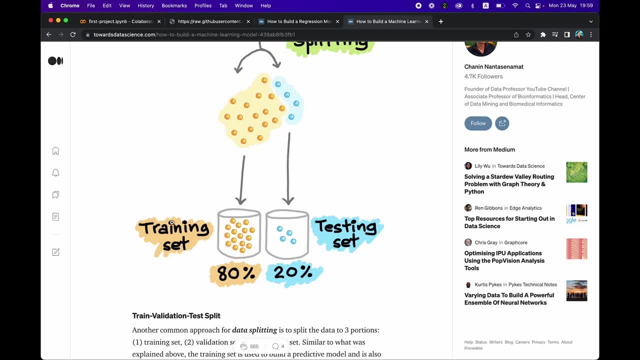 sort of a unknown data that you want to test training set for. you want to evaluate whether the model that you have built using the training set, whether it performed in a robust manner against an unknown data that you simulate using the testing set. Okay, And so, before continuing further, a quick word from our sponsor. 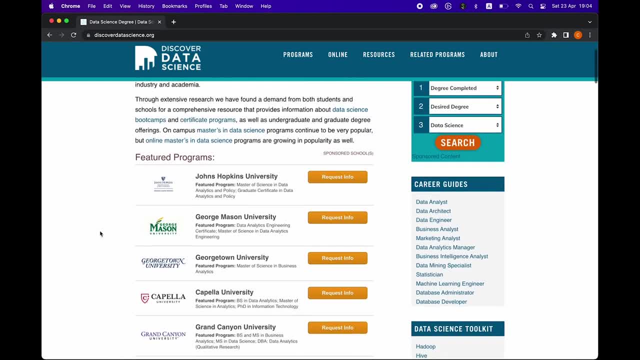 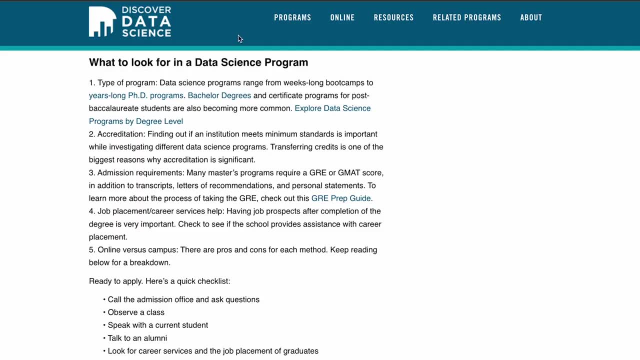 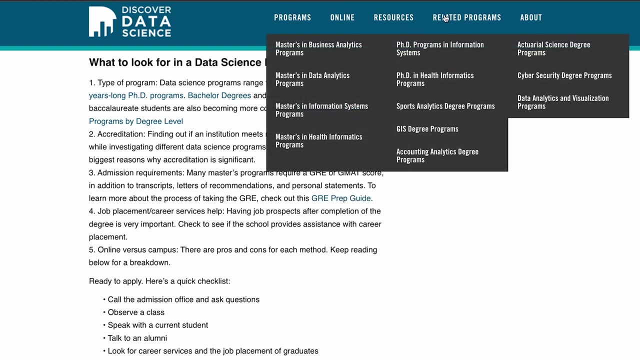 And so a short message from our sponsor, Discover Data Science, powered by Wiley, which is the premier information hub for the field of data science, with in depth guides on careers, degrees and industry leading programming languages. Discover Data Sciences goal is to provide accessible resources and materials for prospective students and professionals. 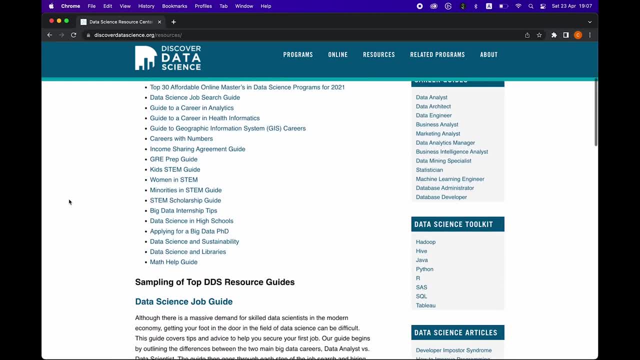 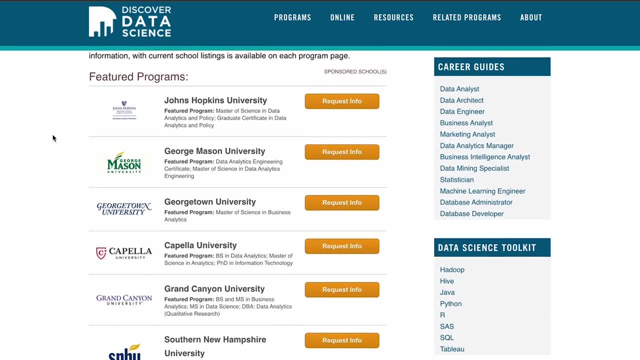 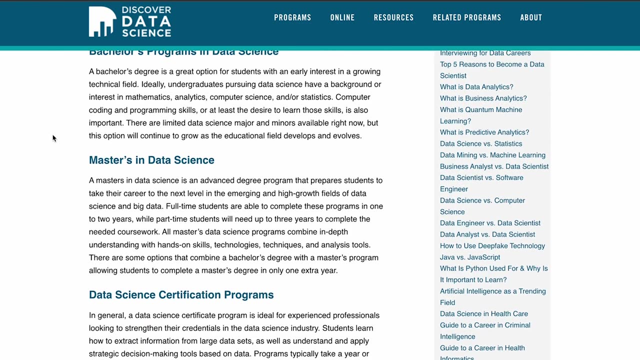 Through Discover Data Science expert driven articles and publications, you'll learn more about which data science degrees help accomplish your professional goals, the tools and skills that are necessary for a successful career in the field. which career paths appeal to your personal interest. how to land a job in data science. 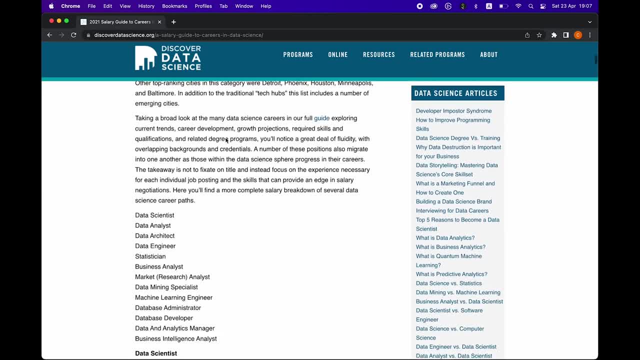 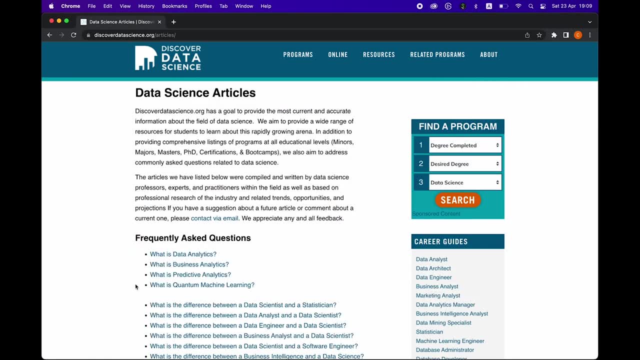 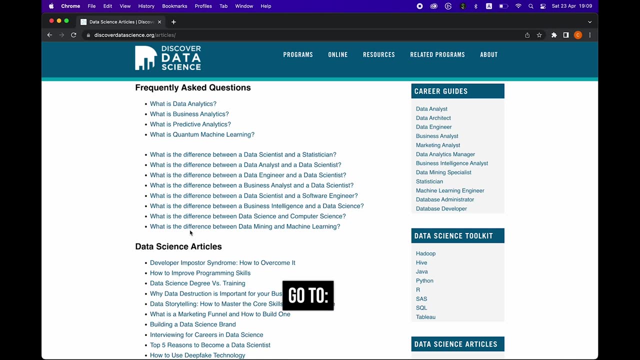 And, as you know, data science jobs are rapidly expanding on a global scale. with a growing need for qualified data science professionals, It's never been a better time to earn your degree and pursue a career- A career- in this rewarding field. you can begin your data science journey by visiting discoverdatascienceorg. 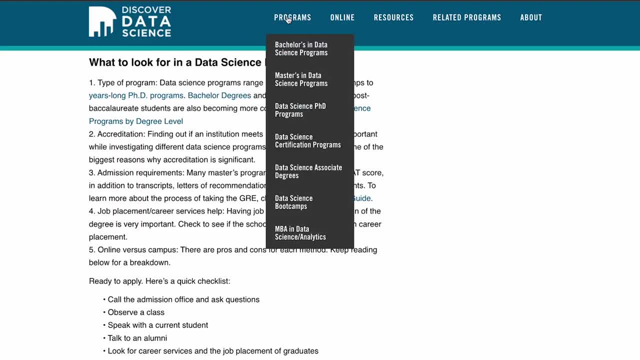 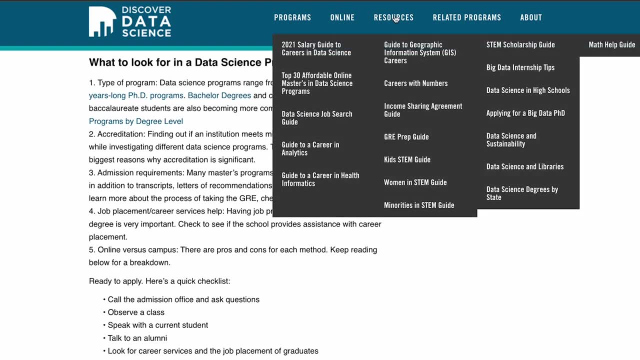 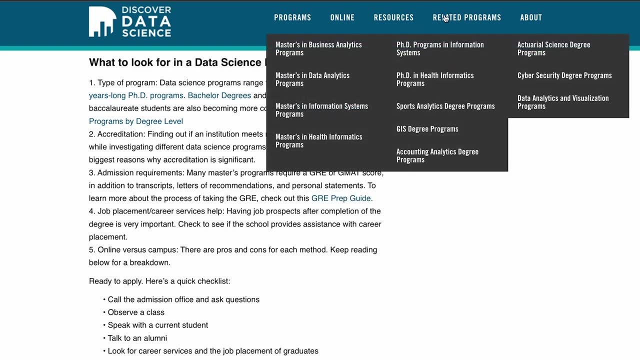 for the field of data science, With in-depth guides on careers, degrees and industry-leading programming languages. Discover Data Science's goal is to provide accessible resources and materials for prospective students and professionals Through Discover Data Science expert-driven articles and publications. 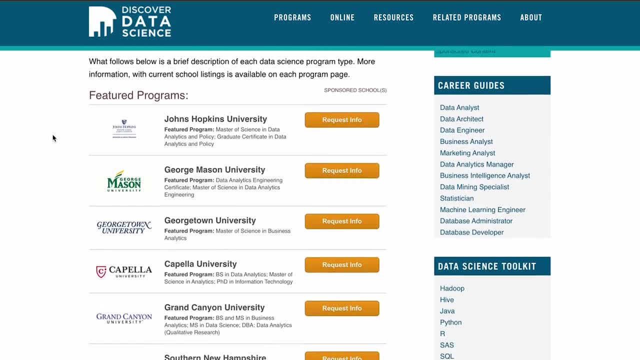 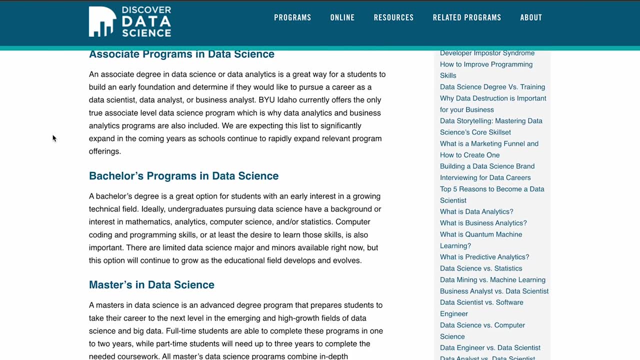 you'll learn more about the field of data science and how it can be used in the field of data science. You'll learn more about which data science degrees help accomplish your professional goals, the tools and skills that are necessary for a successful career in the field, which career. 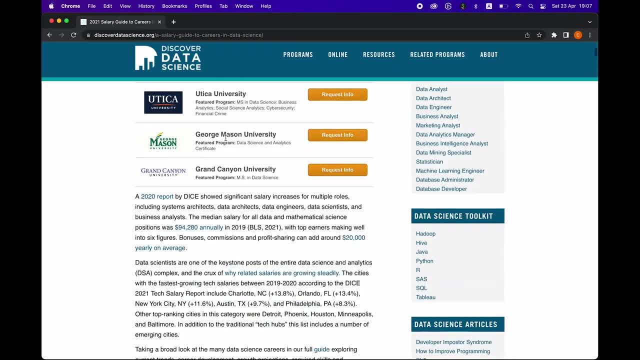 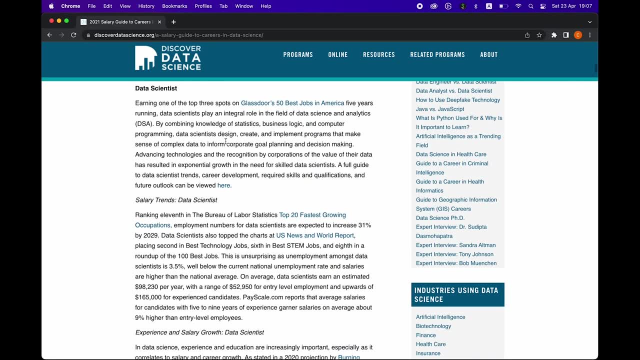 paths appeal to your personal interest. how to land a job in data science? And? as you know, data science jobs are rapidly expanding on a global scale. with a growing need for qualified data science professionals, It's never been a better time to earn your degree and pursue a. 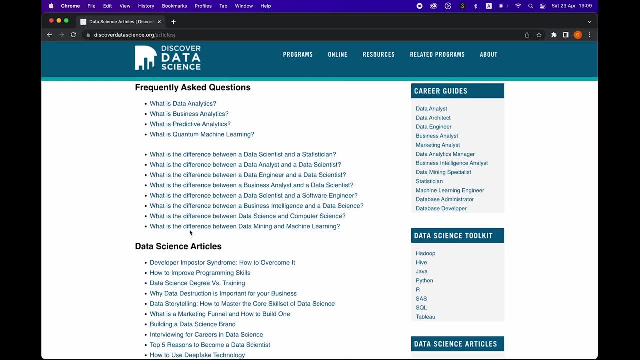 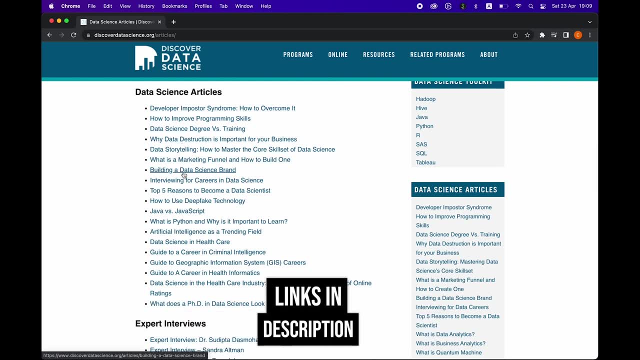 career in this rewarding field. So if you're interested in learning more about data science, you can begin your data science journey by visiting DiscoverDataScienceorg, powered by Wiley, or visit the link in the description below. All right, and so let's continue with the tutorial. 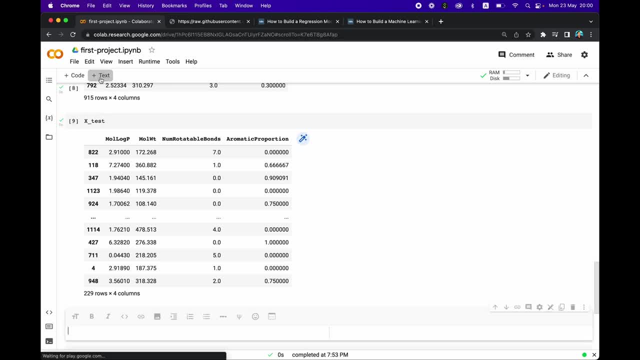 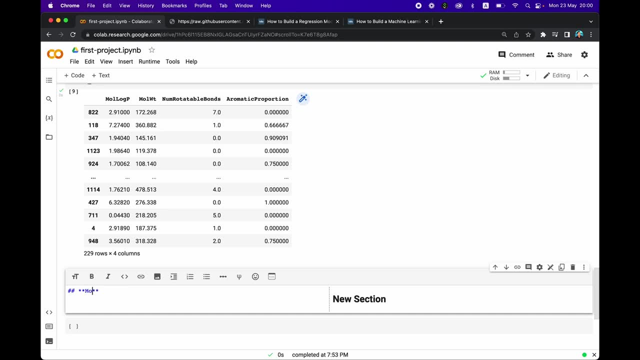 Okay, and now we're going to build the model. So let me add a text cell and I'll add here to be two hash. We'll make it bold, Let's call it model building. And here we're going to add another one. 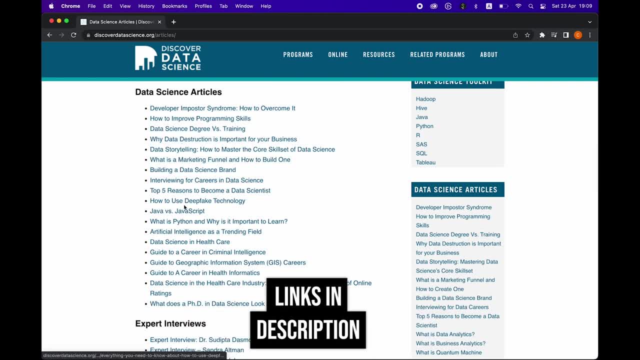 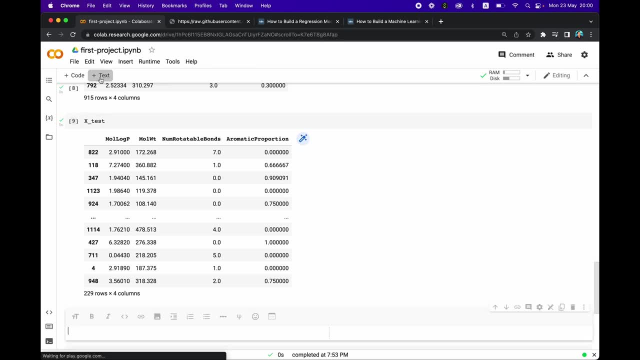 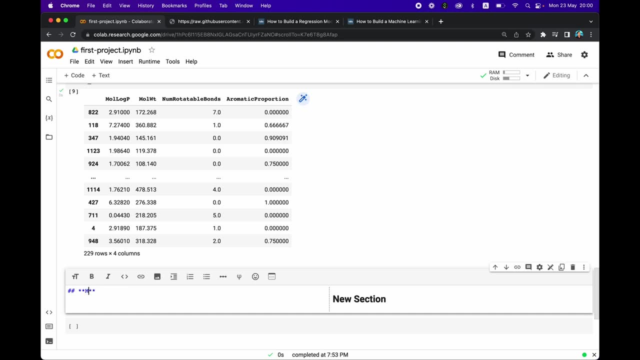 powered by Wiley, or visit the link in the description below. Alright, and so let's continue with the tutorial. Okay, and now we're going to build the model. So let me add a text cell and I'll add here to be two: hash will make it bold. Let's call it model building. And here we're going to build a model And our successes, But before that, I'm going to add a text cell. So let's do a query, let's call it model building, And let's call it model building, Okay, and so I'm going to do two hash. 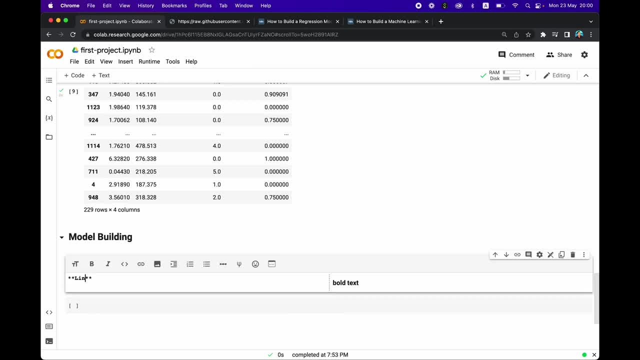 And I'll add text cells. And this is not actually a model And the goal is to get a lot of applications. we're going to add another one. we're going to say linear regression. Let's have it as three hash. we have two here, we have three here. So we have it in a hierarchical form. So if you click here, 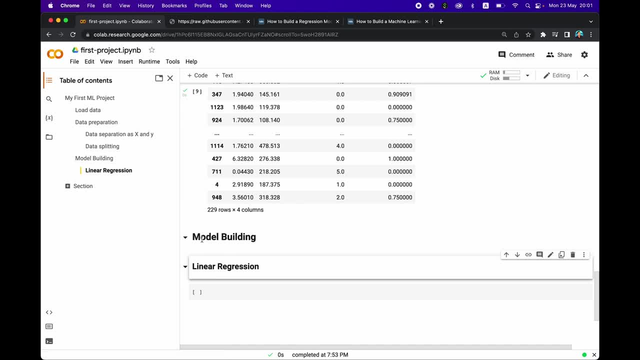 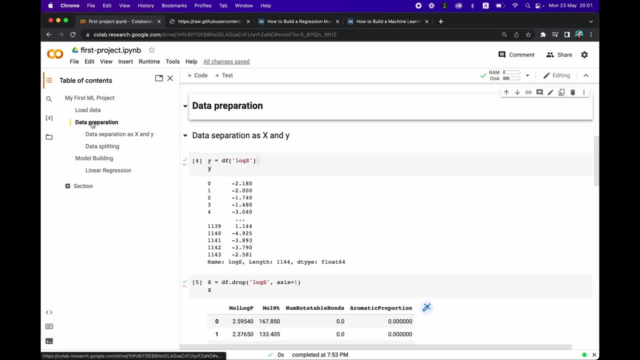 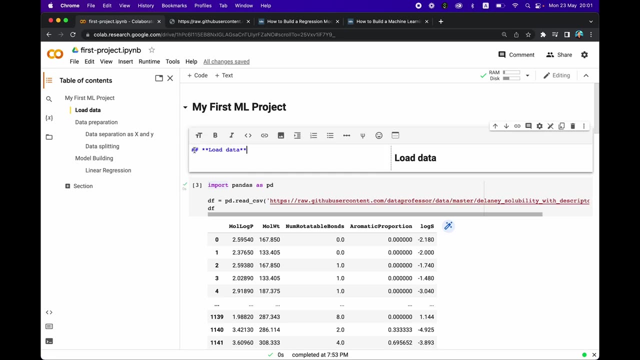 you're going to see the table of content of your code, And so the benefit of organizing your text cells in hierarchical form is that you could see the table of contents here And then you could click through the various sections. So actually, instead of making load data, having two hash, 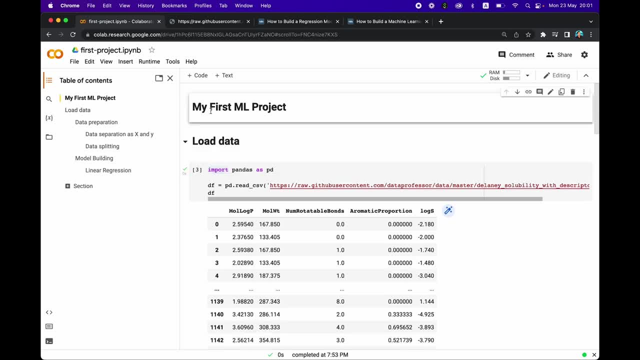 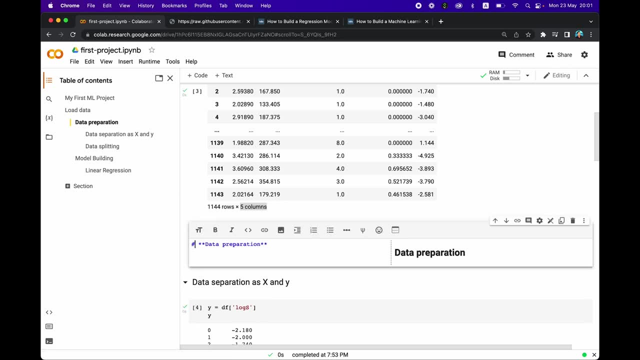 symbol. I'm going to make it into having one, So it's going to be the same as the title, And then you're going to see that this one move to the left a bit, And then we're going to make data preparation to be one as well, one hash. we're going to make data modeling to be one hash like. 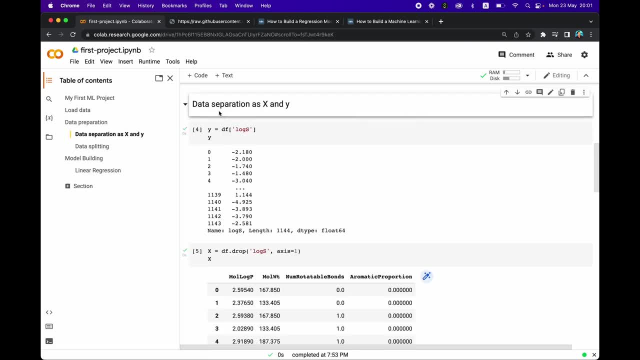 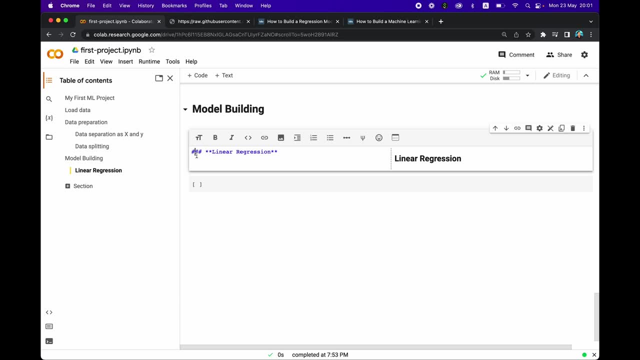 that. And now we're going to make data separation to be two, data splitting to be two, Linear regression to be two. Okay, and now it looks good to me. Okay, And now we're going to continue by populating the code cell underneath the linear regression. So we're going to use 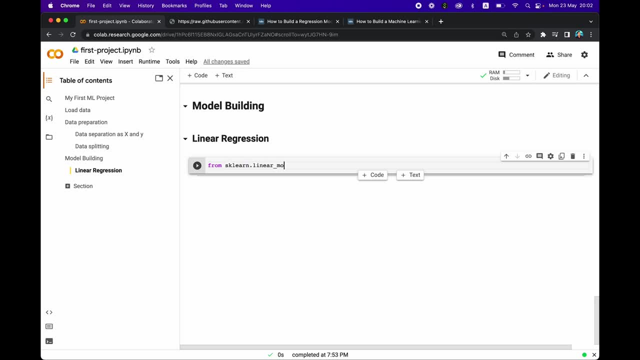 scikit learn from sk learn dot linear model, import linear regression. So you're going to see here that scikit learn has several functions that you could use not only to prepare your data set but also to build a machine learning model. And here we're going to build a typical linear regression. 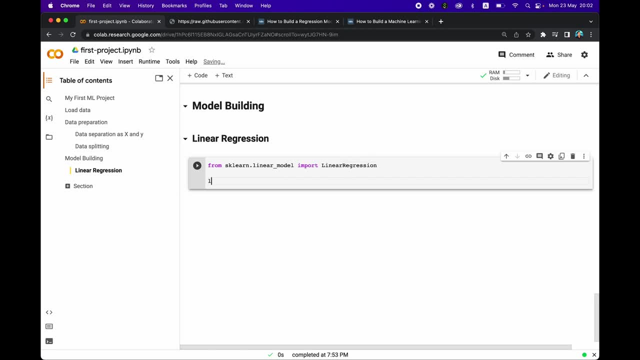 model. And now that we have imported the function, we're going to create a variable called our R, to stand for linear regression. we're going to type in linear regression function here, which will be represented by our R, And then, on the next line, we're going: 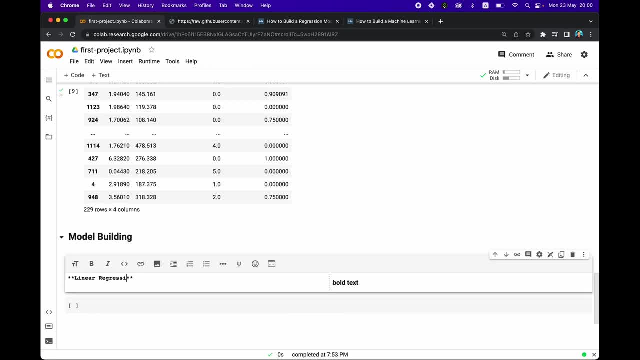 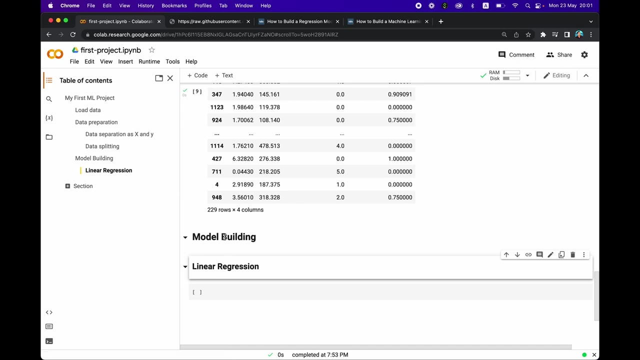 We're going to say linear regression, Let's have it as three hash. We have two here, we have three here. So we have it in a hierarchical form. So if you click here, you're going to see the table of content of your code, And so the benefit of organizing your text cells in hierarchical form. 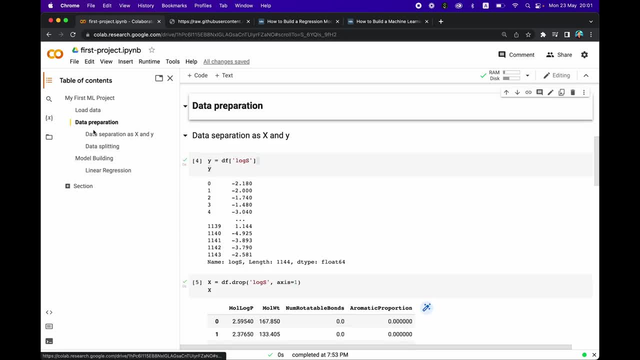 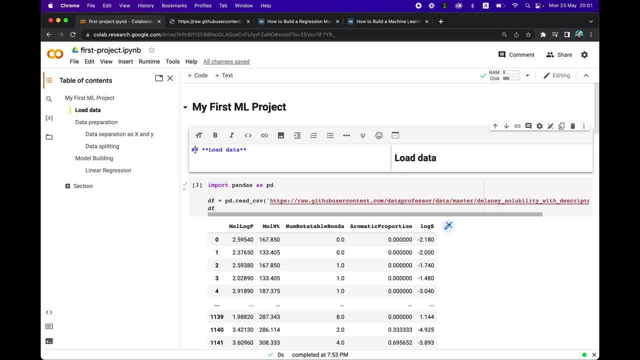 is that you could see the table of contents here And then you could click through the various sections. So actually, instead of making load data having two hash, we're going to say linear regression to hash symbol. I'm going to make it into having one, So it's going to be the same as 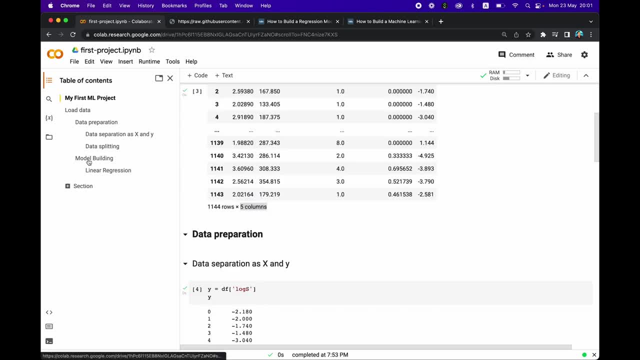 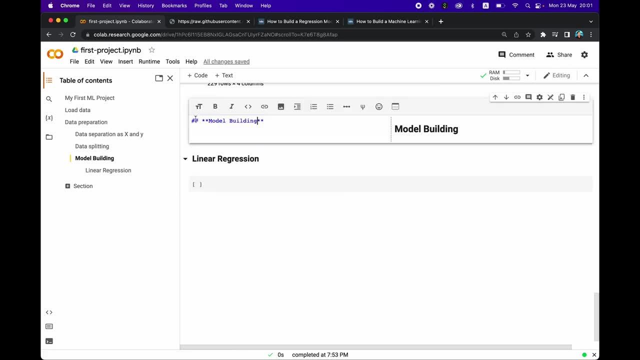 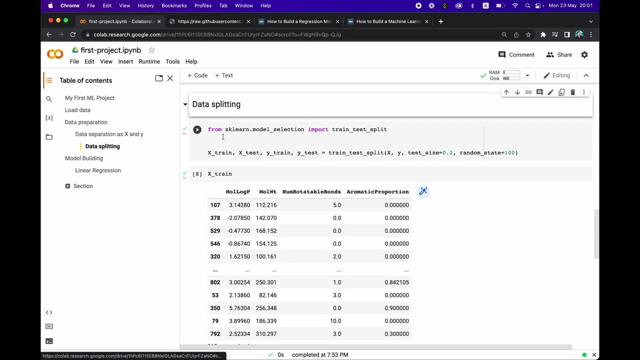 the title, And then you're going to see that this one move to the left a bit, And now we're going to make data preparation to be one as well, One hash. we're going to make data modeling to be one hash, like that. And now we're going to make data separation to be two, data splitting to be two. 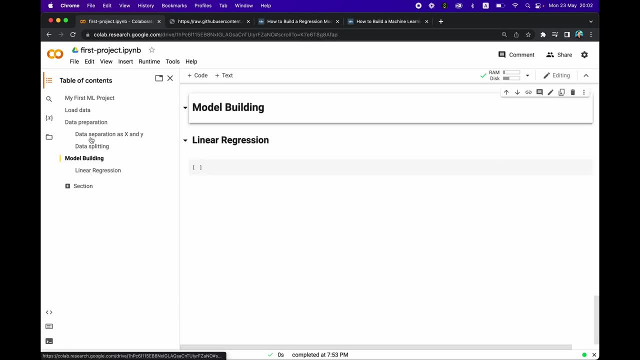 linear regression to be two. Okay, and now it looks good to me. Okay, and now we're going to continue with the tutorial. So let's go ahead and start the tutorial. So let's go ahead and start the tutorial by populating the code cell underneath the linear regression. So we're going to use 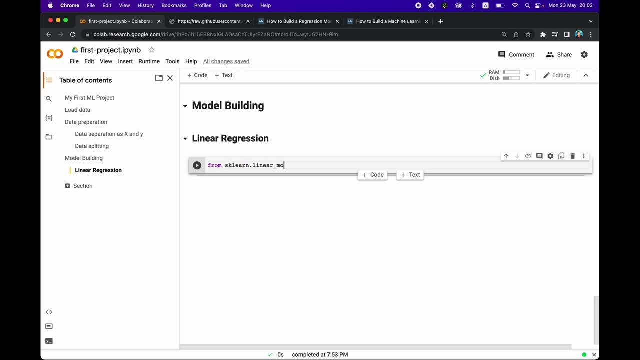 scikit learn from sk learn dot linear model, import linear regression. So you're going to see here that scikit learn has several functions that you could use not only to prepare your data set but also to build a machine learning model. And here we're going to build a typical linear regression. 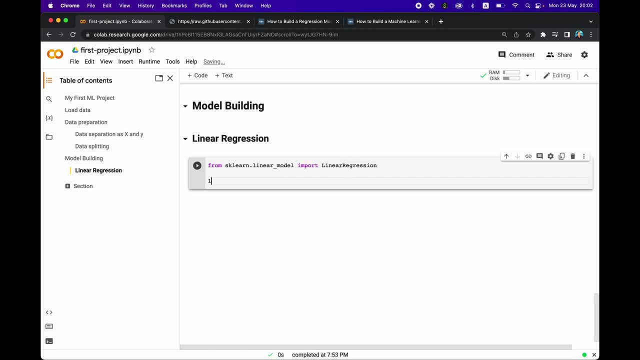 model, And now that we have imported the function, we're going to create a variable called our to stand for linear regression. We're going to type in linear regression function here, which will be represented by LR, And then, on the next line, we're going to run our dot fits, which means that we want to train the empty linear 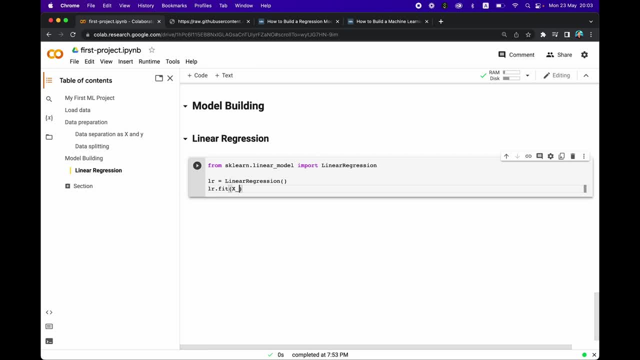 regression model on the following data set, which we specify to be extreme comma y train, and then we run it. you could click here, or what I like to do is I like to use the keyboard shift enter, which is quicker for me, and the model is: 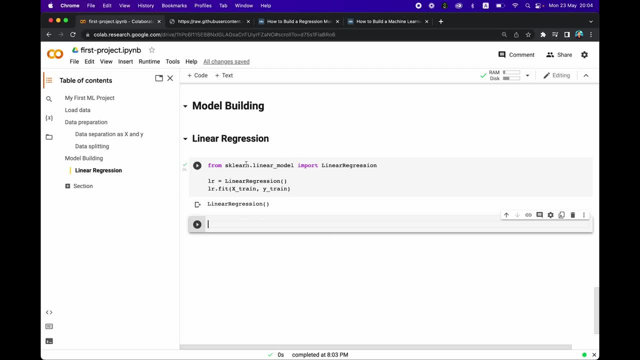 built And now that the model is built, we want to apply this particular model to make a prediction. So let me add the text here so that we could annotate it a bit more. we could say: training the model, make it bold, applying the model to make prediction. 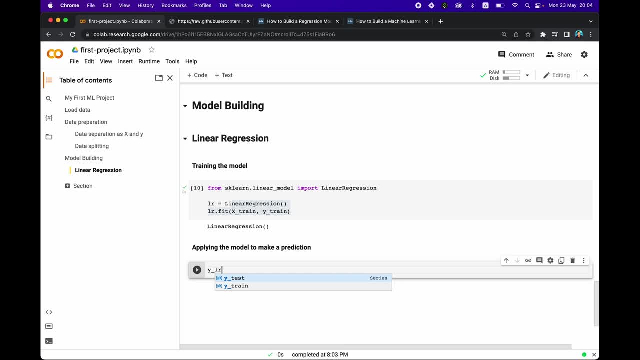 And we're going to call it y underscore, LR underscore train, underscore pred. So we're going to apply the model to make a prediction on the training set And the prediction to notify that we're going to use pred And then to make note of the algorithm. 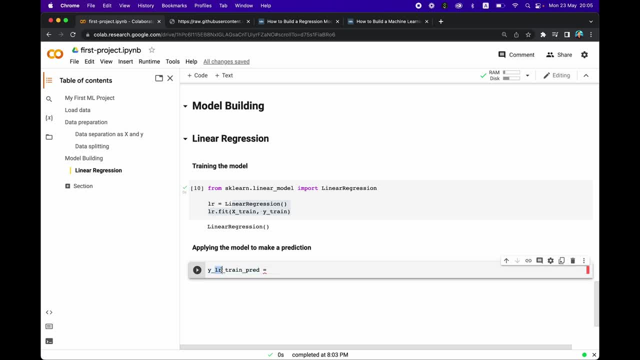 that we're using to train the model we're going to specify to be what our here, and then we're going to start with the y underscore. So this naming convention will be helpful when we have several machine learning algorithms that we want to try out, And also whether our prediction is. 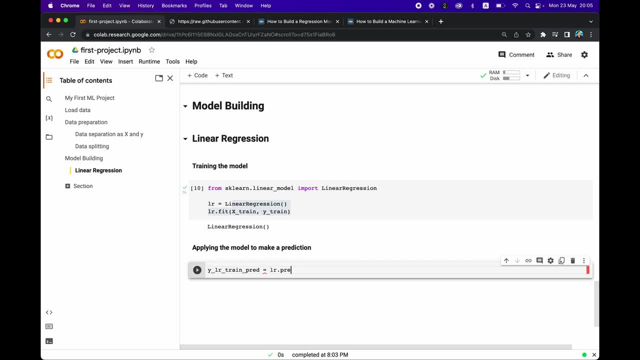 made on the training set or the testing set. So type in our dot predict, and then I'm going to specify x, train And this is going to be the data, because we want to make the prediction here on the x train. So essentially, 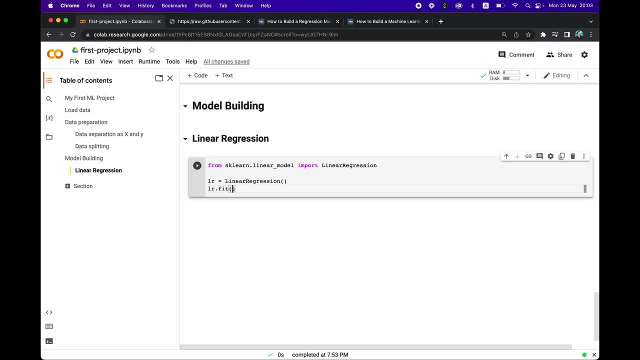 to run our R dot fit, which means that we want to train the empty linear regression model on the following data set, which we specify to be extreme comma y train, and then we run it. you could click here or whatever. Okay, and then as well, just on the right there, we have a place here where we can use this through. 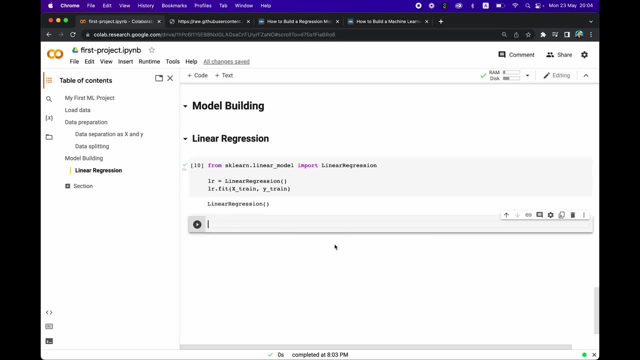 our pool And we can try to make itILеля Corinth, which in this case we'll call, is variable And I'd like to do is- I'd like to use the keyboard Shift Enter, which is quicker for me, and the model is built. And now that the model is built, we want to apply this particular model. 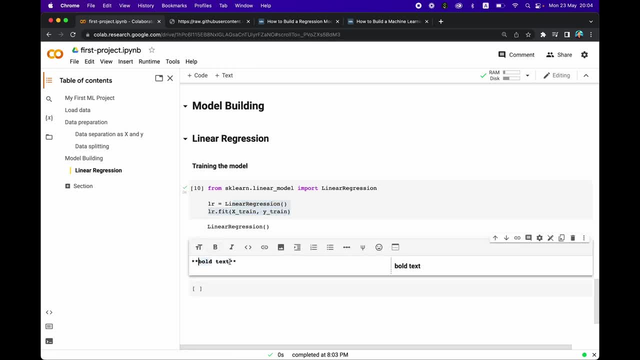 to make a prediction. So let me add the taps here so that we could annotate it a bit more. we could say: training the model and make it bold: flying the model to underscore train, underscore pred. So we're going to apply the model to make a prediction on the 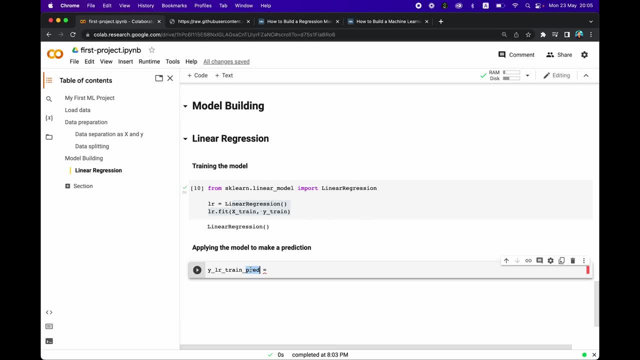 training set and the prediction to notify that we're going to use pred and then to make note of the algorithm that we're using to train the model we're going to specify to be lr here, and then we're going to start with the y underscore. So this naming convention will be helpful when we 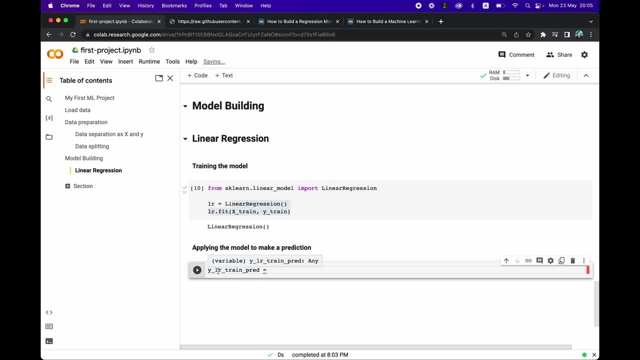 have several machine learning algorithms that we want to try out and also whether our prediction is made on the training set or the testing set. So type in lr dot predict and then I'm going to specify x train to be the data, because we want to make the prediction here on the x train. So 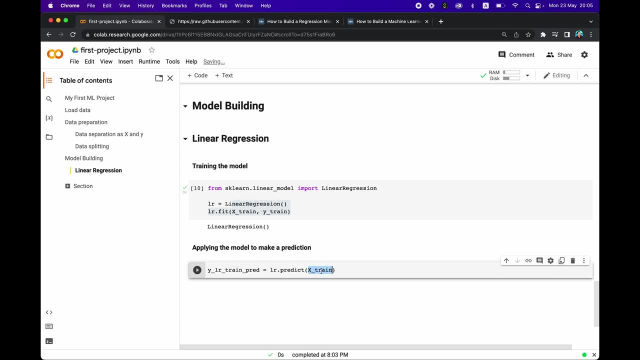 essentially, we're going to do the recall. It's going to be making prediction on the original data set that it has been trained on, and so that will allow us to evaluate the performance of the algorithm. So here we're going to call it: y underscore, lr underscore test. 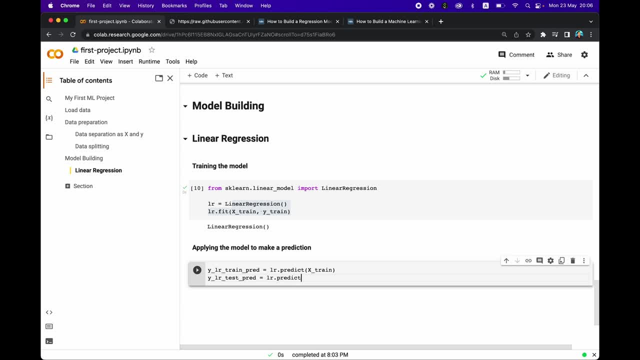 and then we're going to make the prediction on the training set. So type in lr dot predict and underscore pred equals lr dot predict and, as you've guessed, y underscore test. Let's do it. Let's print out the results: Y underscore lr train pred. y underscore lr test pred. 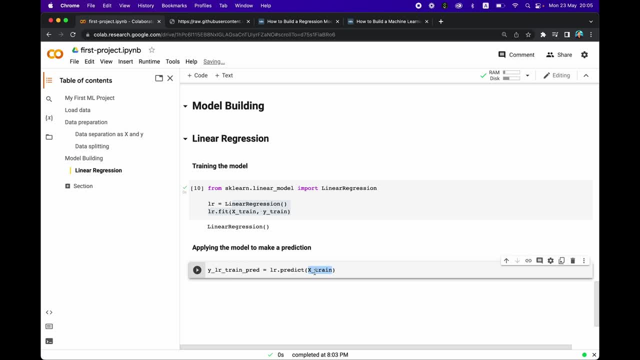 we're going to do the recall. it's going to be making prediction on the original data set that it has been trained on, And so that will allow us to evaluate the performance of the algorithm. So here we're going to call it: y underscore, LR, underscore, test, underscore pred equals our dot predicts, And as you've guessed, 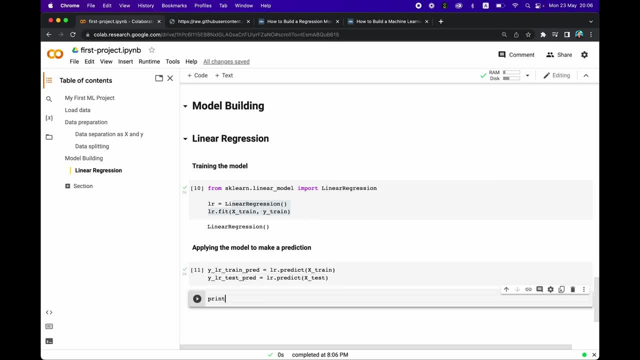 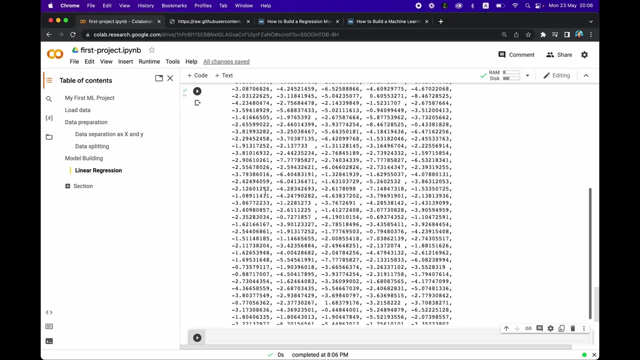 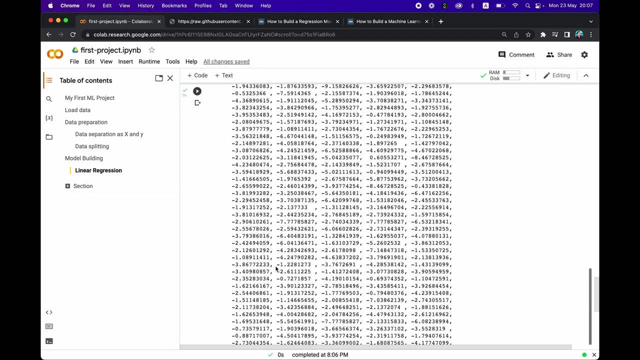 y underscore test. let's do it. Let's print out the results: y underscore LR train pred. y underscore LR- test spread. Actually, let's just make it like that. Okay, so these are all of the predictions of. look here. So these represents the 80% of the data. 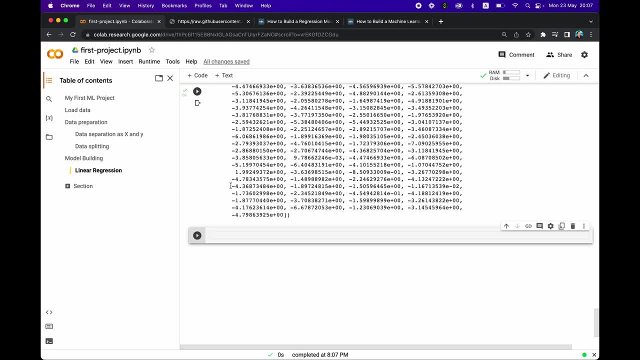 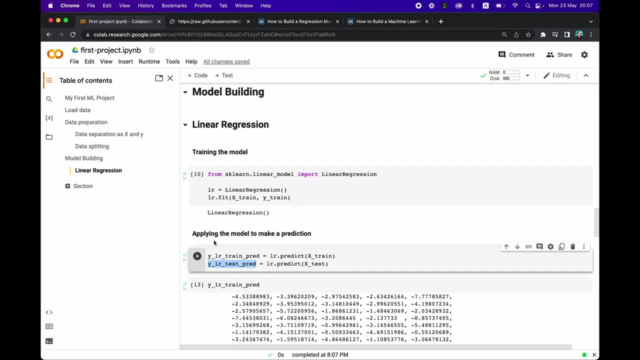 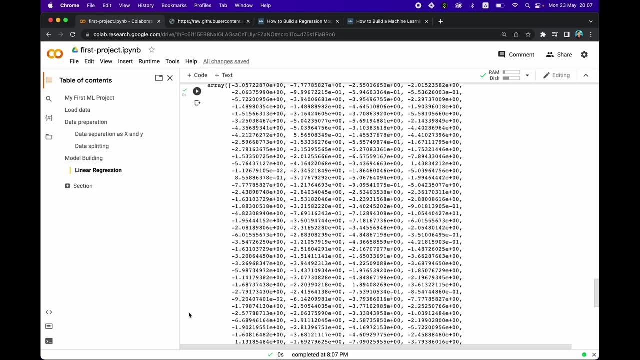 And there you go. the remainder 20% of the data has been predicted And we have the predicted value. And the next part here is we're going to compare the predicted value with the original value or the actual value And we're going to call the new section here to be model. 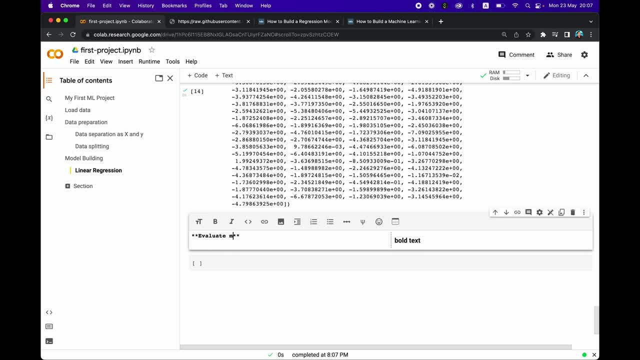 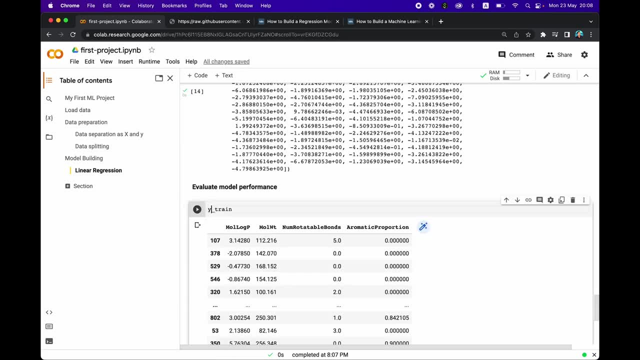 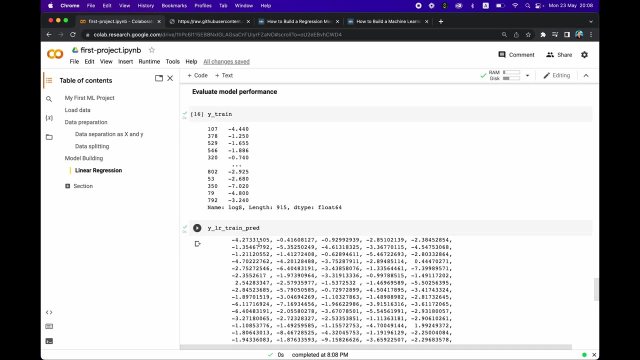 performance. We're going to say evaluate model performance, Because we want to compare x train here, No, not not extreme y train with the here y LR train. So you're going to notice that they are the actual value and the predicted value. 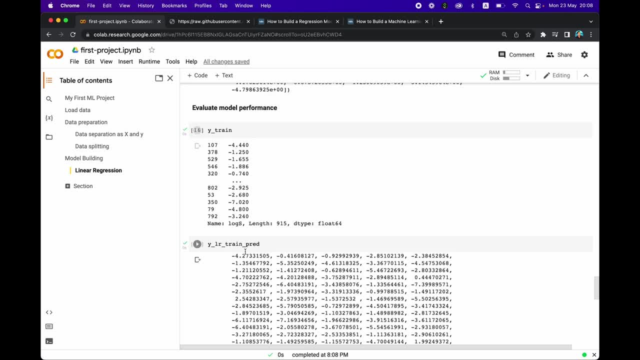 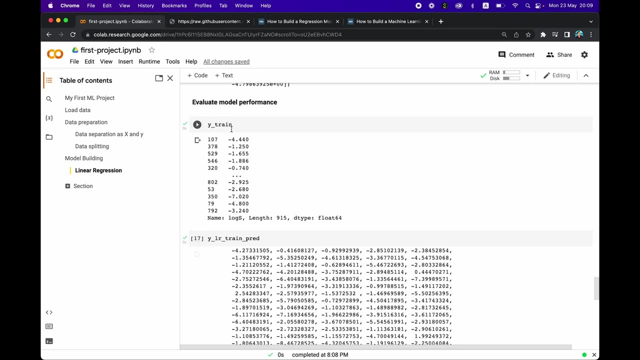 Okay, so in just a moment I'm going to show you a scatter plot of these two values and if they lined up in a diagonal trendline and see whether they have high dispersion or low dispersion. So if the dispersion is low, we will expect that the performance will be good. Okay, and so now that we see, 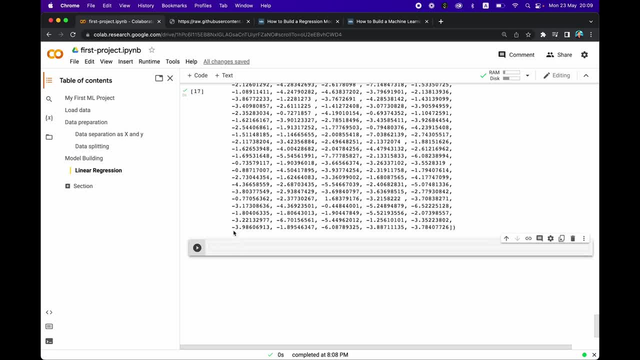 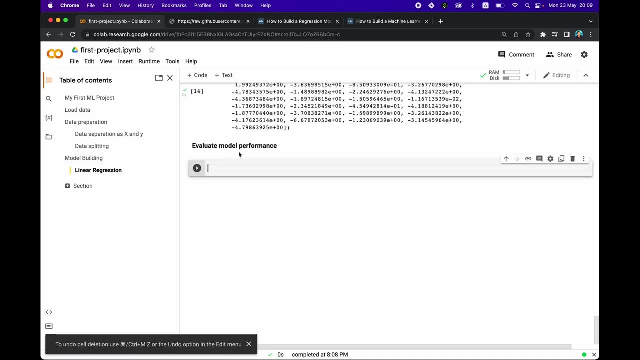 the data that we are going to use. we're now going to actually perform the model evaluation. Let me delete it here first. delete, delete. delete. add the code cell and we're going to type in from sklearnmetric import: mean underscore, squared underscore, error and we're going to use the r2 score. function lr underscore train mean squared error equals to mean squared error. function y train underscore y out train cred. 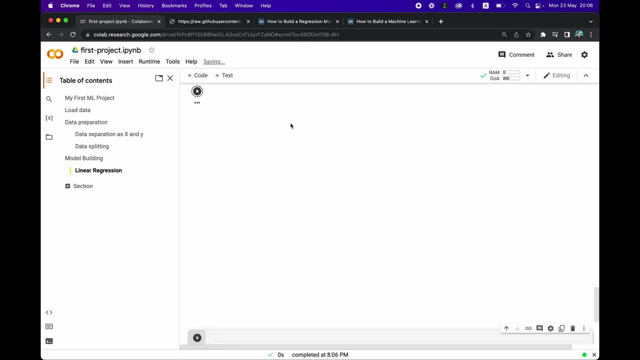 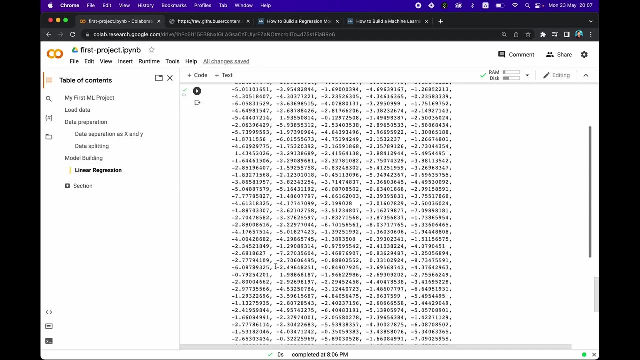 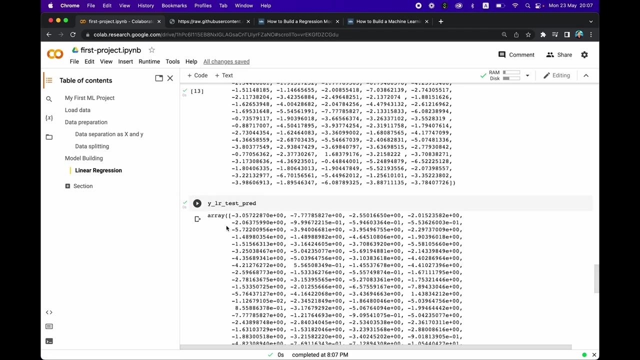 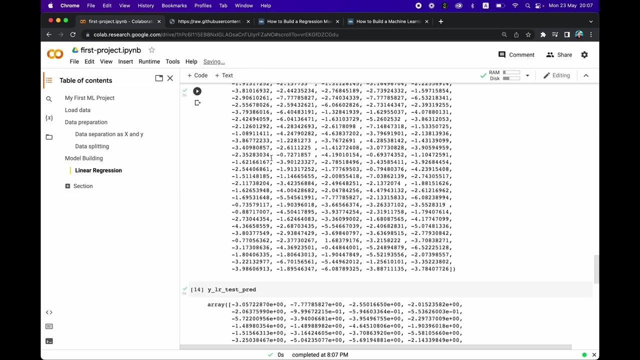 Actually, let's just make it like that. Okay, so these are all of the predictions. Have a look here. So these represents the 80% of the data, and there you go. the remainder 20% has been predicted and we have the predicted value. and the next part here is we're going to. 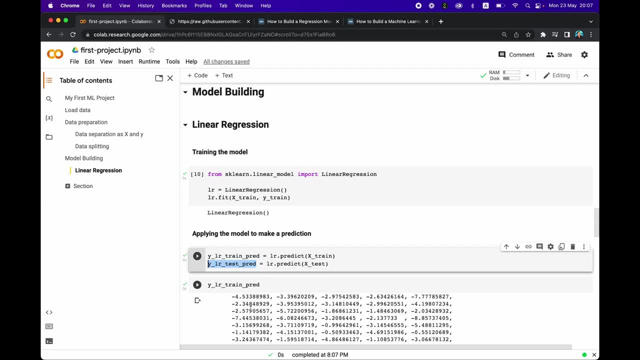 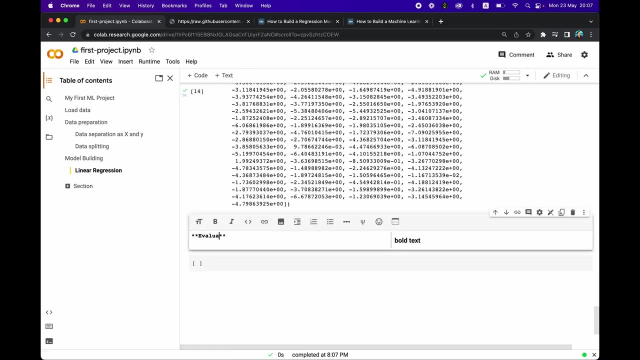 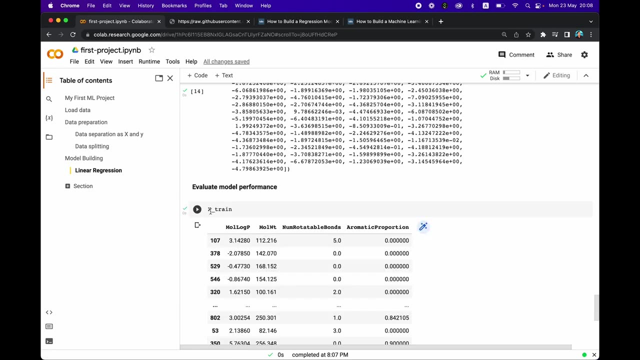 compare the predicted value with the original value or the actual value. and we're going to call the new section here to be model performance. We're going to say evaluate model performance Because we want to compare x train here, no, not not x train, y train with the here y lr train. 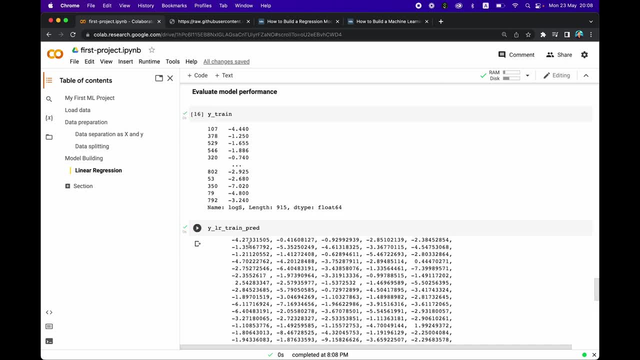 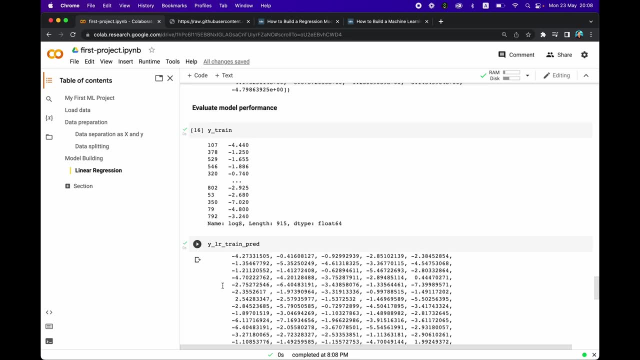 So you're going to notice that they are the actual value and the predicted value. Okay, so in just a moment I'm going to show you a scatter plot of these two values and if they lined up in a diagonal trend line and see whether they have high dispersion or 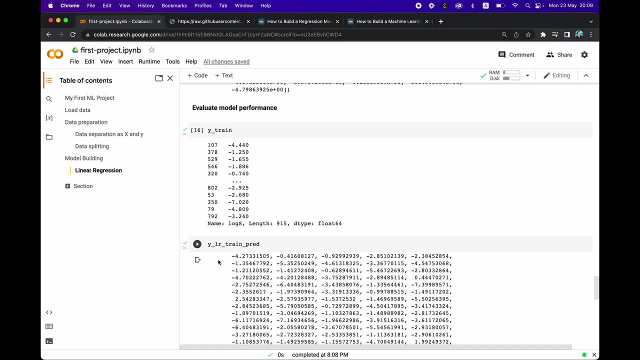 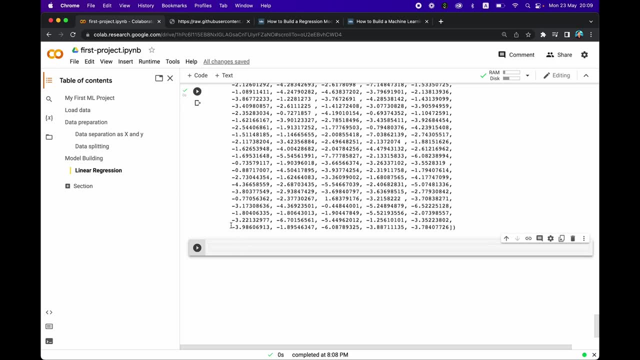 low dispersion. So if the dispersion is low, we will expect that the performance will be good. Okay, Okay, and so now that we see the data that we are going to use, we're now going to actually perform the model evaluation. let me delete it here first. delete- delete at the code cell. 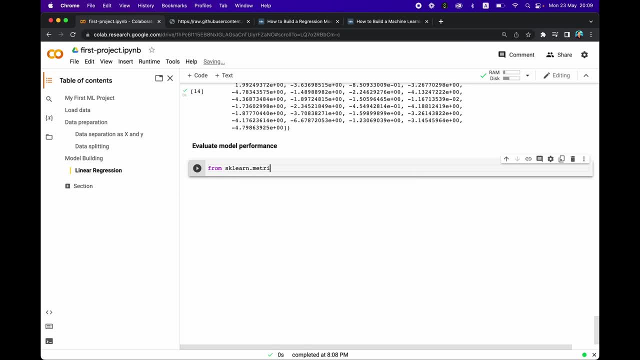 And we're going to type in from sklearnmetric import: mean underscore, squared underscore error and we're going to use the R 2 SCORE function: L R underscore train mean squared error equals to mean squared error function. Mean squared error function L R underscore train equation equals to mean squared error function. 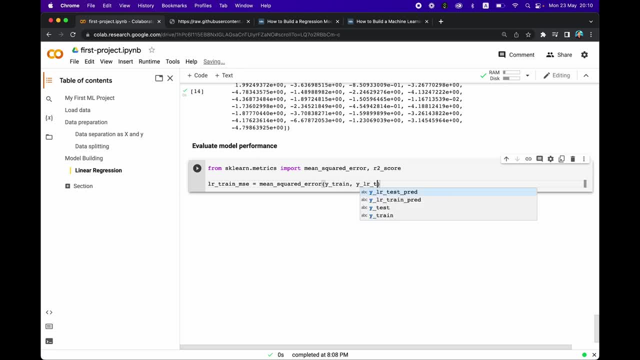 y train underscore y l train pred. and so these are the two variables that we have taken a look just a moment ago and now we're going to calculate the mean squared error. we're going to calculate the squared correlation coefficient using the r2 score function: y train and you guessed y l r train. 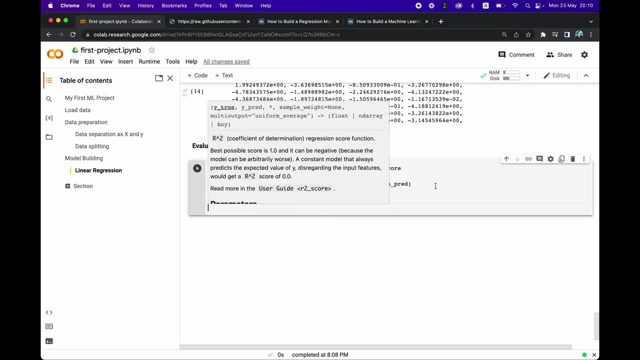 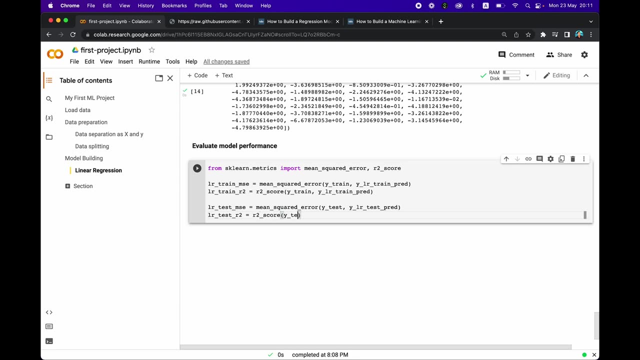 pred. and so these two blocks are for the training set. now we're going to do the same for the testing set. mean squared error. one test, r underscore test pred l r test under two equals r2 score and we have y test and the y l r test underscore pred. run it. let's run values here. 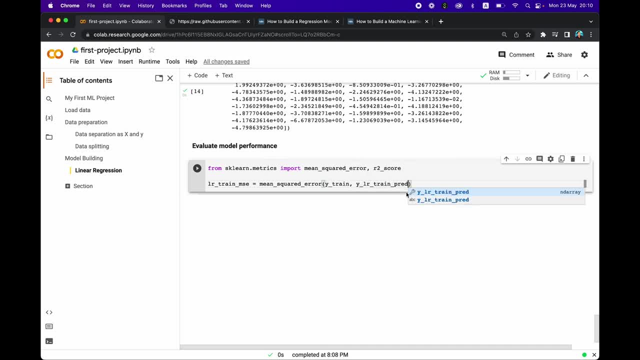 And so these are the two variables that we have taken a look just a moment ago, And now we're going to calculate the mean squared error. we're going to calculate the squared correlation coefficient using the r2 score function: y train, and you guessed y- lr train, cred. 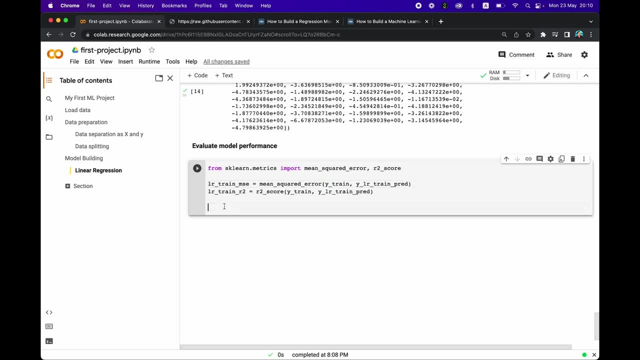 And so these two blocks are for the training set. Now we're going to do the same for the testing set. mean squared error. one test: r underscore test, cred lr test. two equals r2 score and we have y test and the y lr test underscore cred. run it. let's run values here. 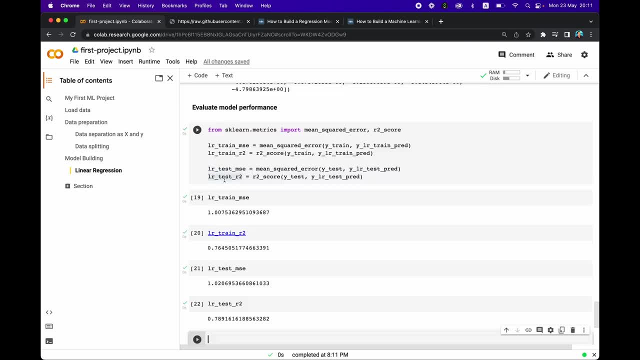 Okay, they're reasonably similar performance here. So we could tidy it up a bit by saying the lr mse and then we say training or to train equal, or colon print, and then we're going to have this one here, we're going to re use it r2, that will be our train r2 case here, and then we're going to to to be test. 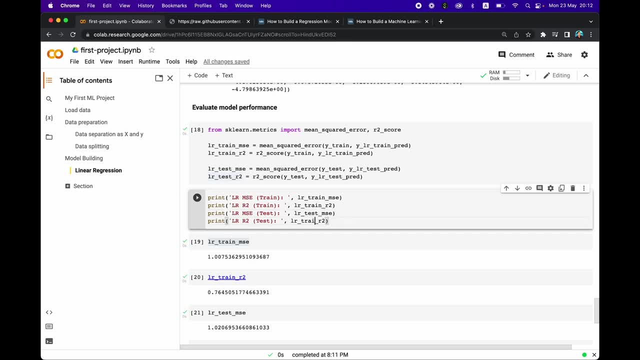 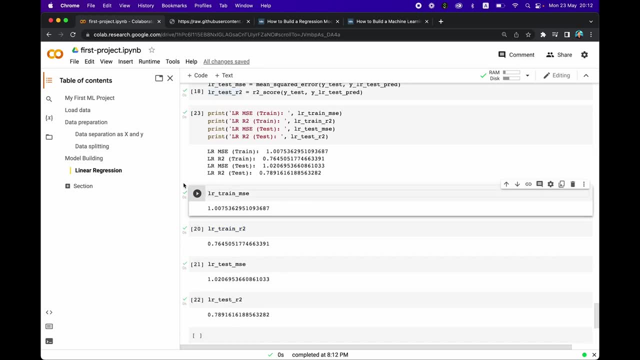 test. this would be test. this would be the test. Okay, there you go. So, instead of having four of these, we're going to delete them, So you could highlight multiple cells just by highlighting it, and then you could click on: either you want to move it or, in this case, I'm going to delete them. 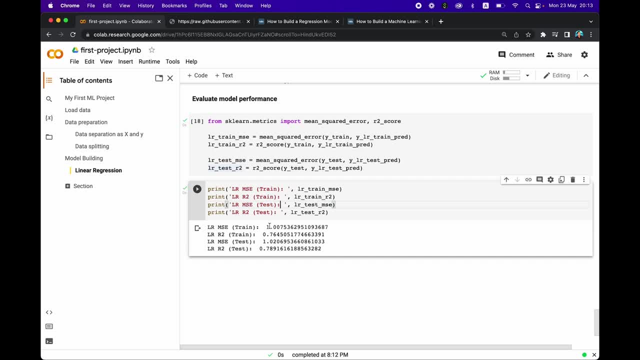 Okay, Okay. so we see all of it at a glance here. However, we could tidy up this particular layout a bit more. Let me show you our results, And then we're gonna create a pandas data frame. We're gonna call this linear regression. 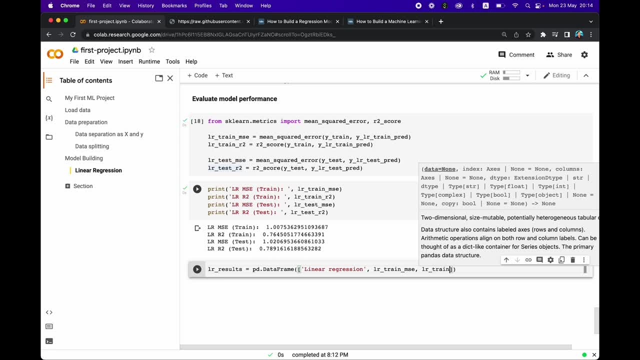 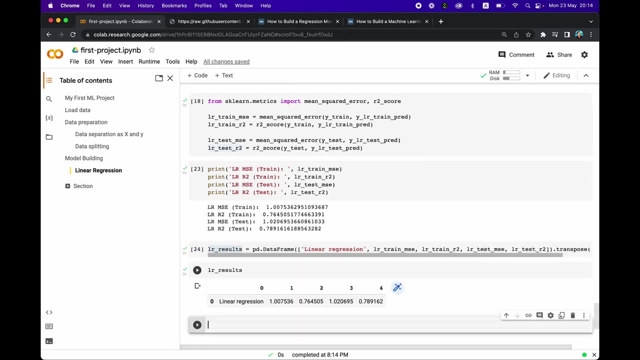 lr train mse. lr train r square. lr test mse. lr test underscore r two. And then we're going to transpose it And let's have a look, Looks like that. And now we need to change the column names here: Zero one, two, three, four. 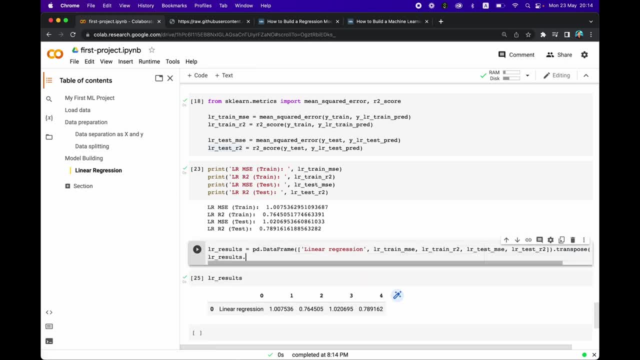 So what we want to do here, lr results dot columns, And we're gonna rename it. We're gonna call it the first column to be method, second column to be training mse, And then we have training r square, And then we have 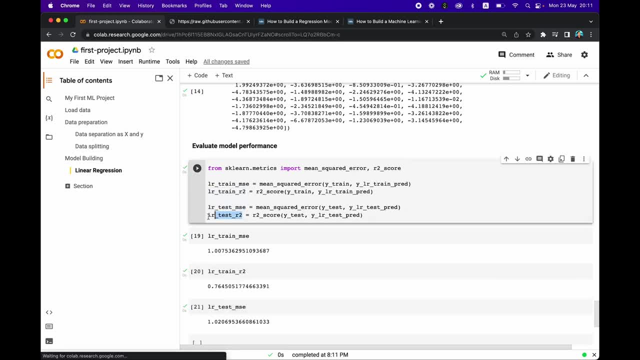 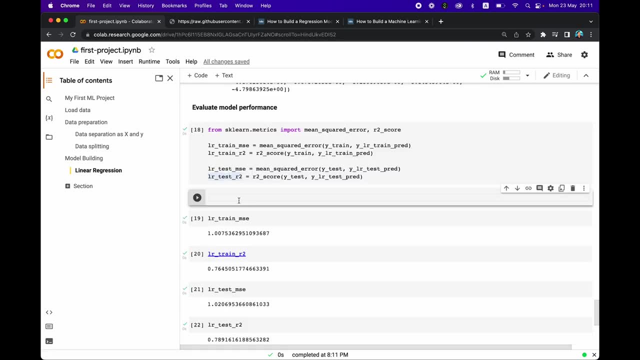 okay, they're reasonably similar performance here. so we could tidy it up a bit by saying the l r mse, and then we say e, and then we say training or to train equal, or colon print, and then we're going to have this one here, we're gonna reuse it r2, but that will be our train. r2 is here and now we're going to train. 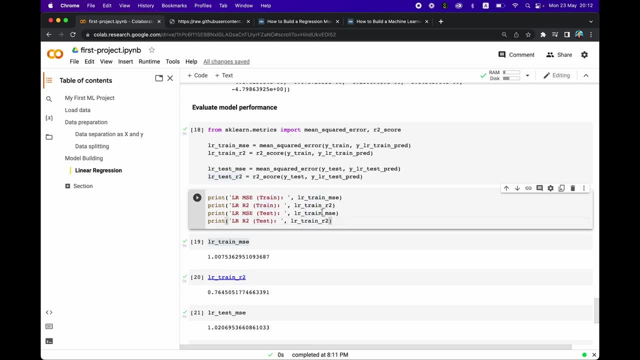 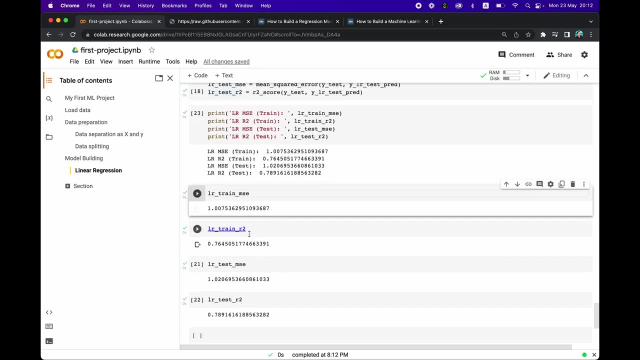 this to be test test. this would be test. this would be test. okay, there you go. so, instead of having four of these, we're gonna delete them, so you could highlight multiple cells just by highlighting it, and then you could click on either you want to move it or, in this case, i'm going to delete them. 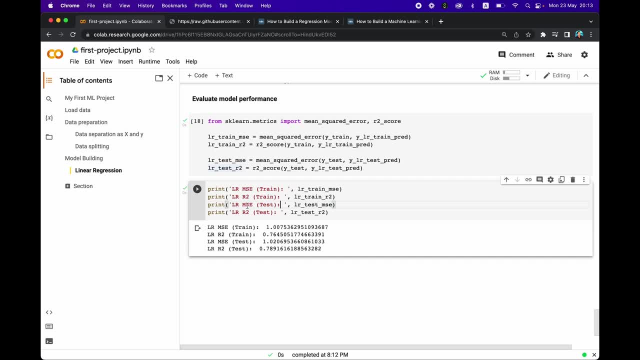 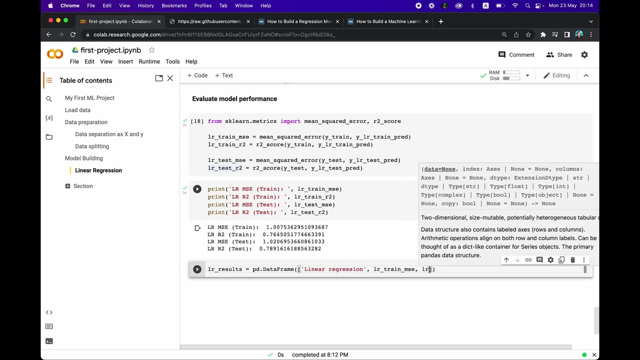 okay. so we see all of it at a glance here. however, we could tidy up this particular layout a bit more. let me show you lr results. and then we're going to create a pandas data frame. we're going to call this linear regression. lr mean mse, lr train r square. 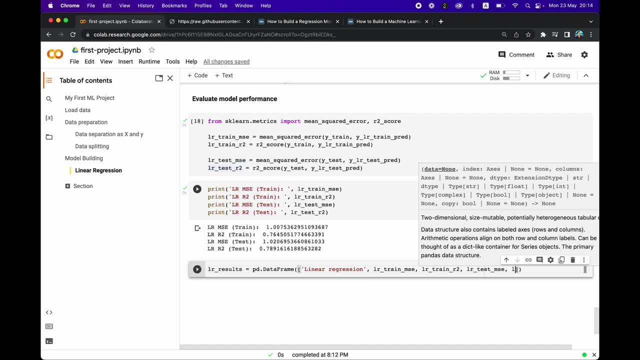 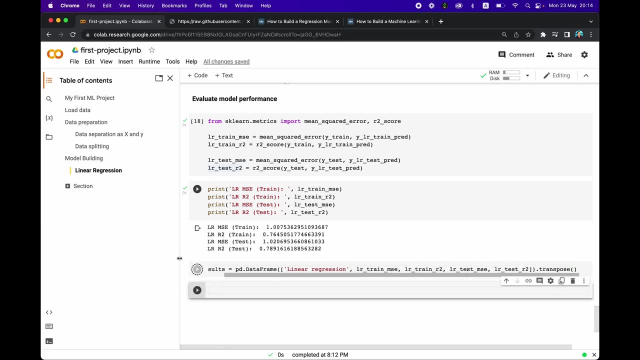 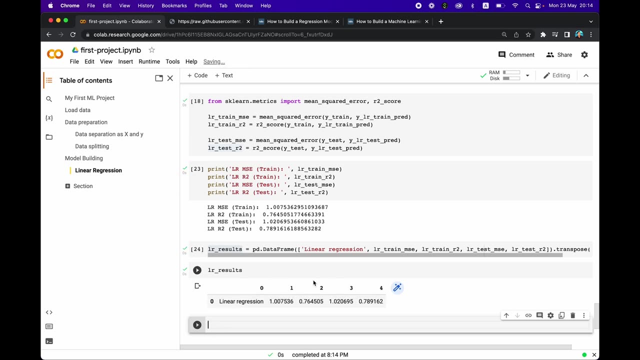 lr test, mse. lr test: underscore r2. and then we're going to transpose it and let's have a look. it looks like that and now we need to change the column names here: 0, 1, 2, 3, 4. so what we want to do here, lr results dot columns and we're going to rename it. we're 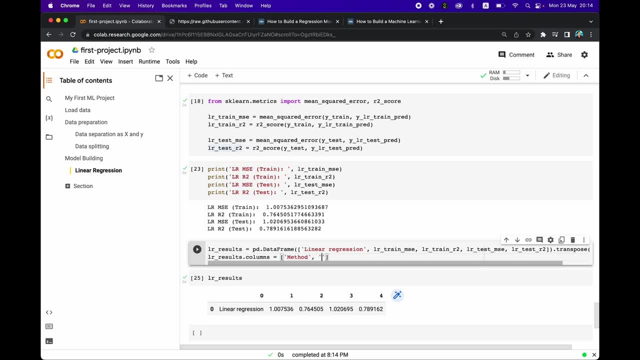 going to call the first column to be method, second column to be training mse, and then we have training r square, and then we have test mse, and then we have test r square. run it. there you go. it looks much cleaner, much cleaner than this in a tabular form, and so the 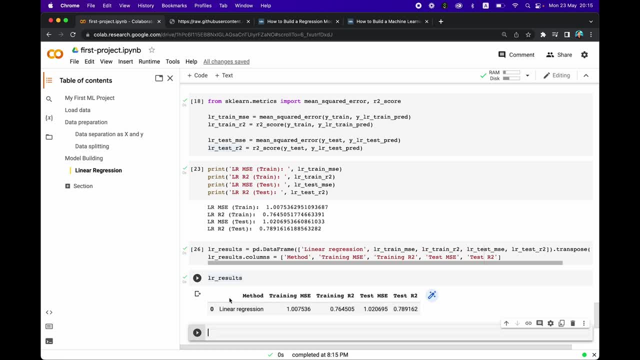 great thing about having it in a pandas data frame like this is that it's not going to be a lot of work, but it's going to be a lot of work. and it's going to be a lot of work if you evaluate more and more machine learning models like random forest k- nearest neighbor. 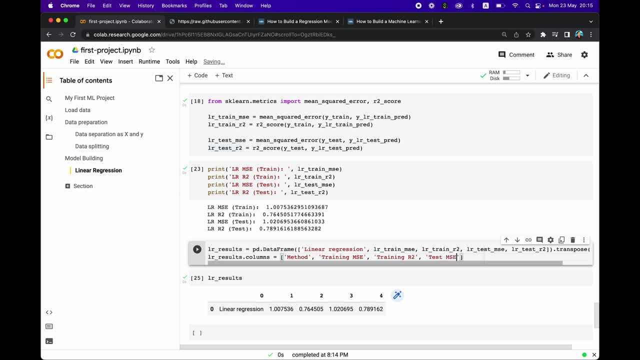 test mse, and then we have test r square, Run it. There you go. It looks much cleaner, much cleaner than this in a tabular form, And so the great thing about having it in a pandas data frame like this is that, if you evaluate more and more machine learning models, 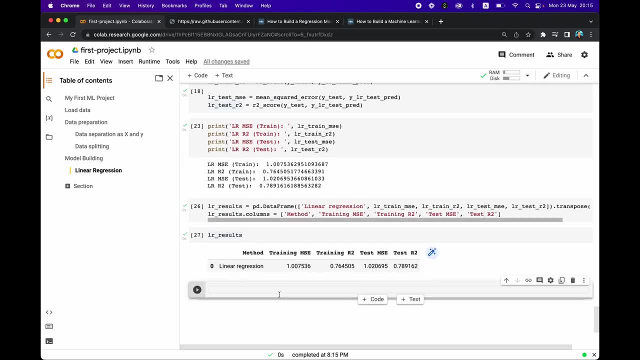 like random forest k nearest neighbor support vector machine neural network. then you're gonna have a data frame that will allow you to easily compare. You could also sort by column the performance and that will help you to evaluate which one was the best. 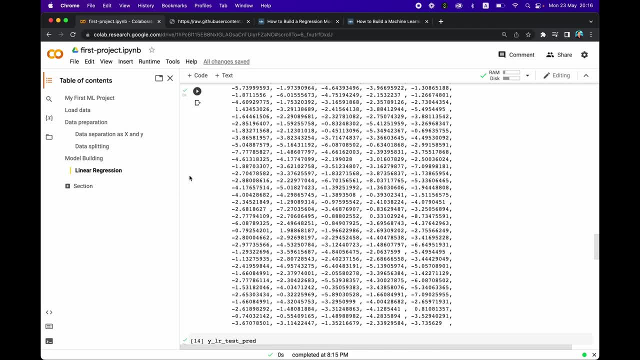 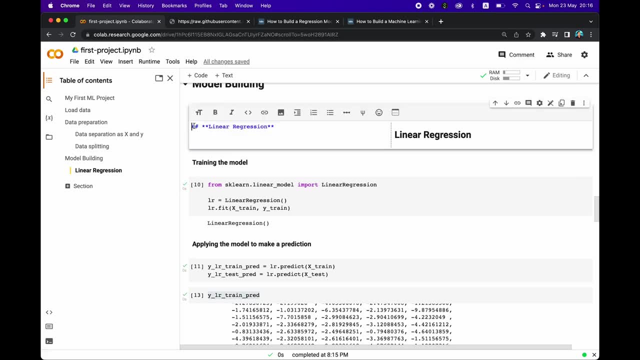 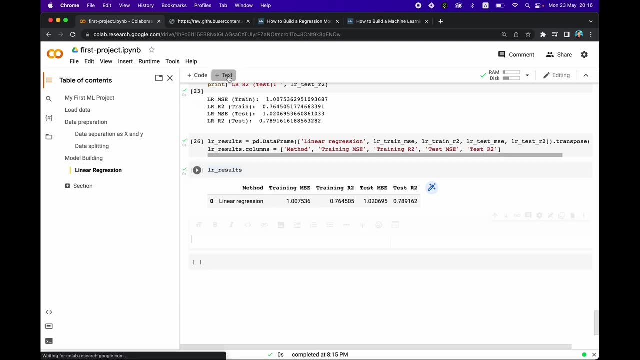 So here you have already built a linear regression model and we're gonna try out another one, which is the random forest. Let's see, We have two hash symbol here. So we're going to add a text cell, add two, And then we're gonna call it random forest. 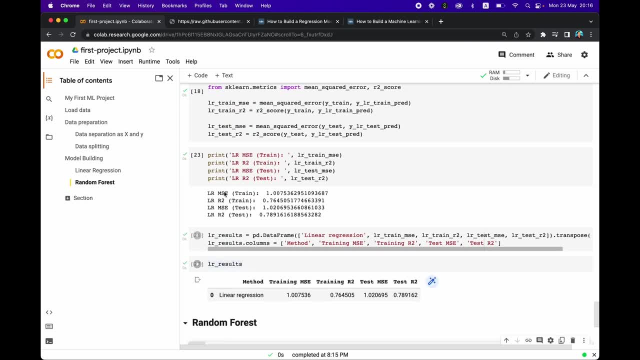 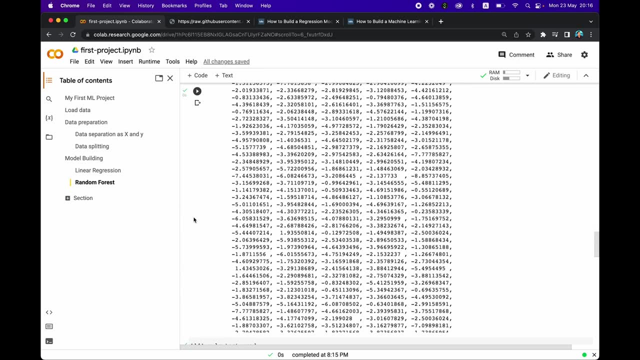 Random forest, And then you could see it here, but notice that you don't see the bold text, cause it needs to be in a hash symbol which will give it a heading one, heading two, heading three, you know, like the hierarchical ordering. 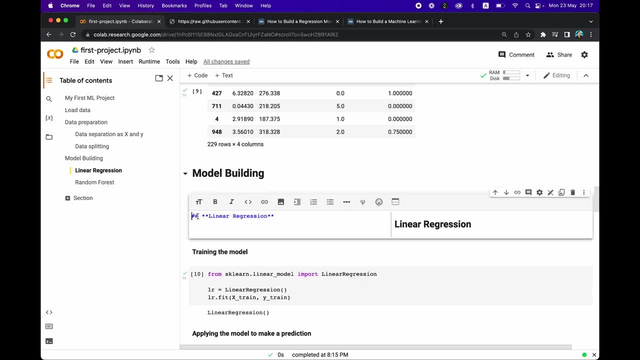 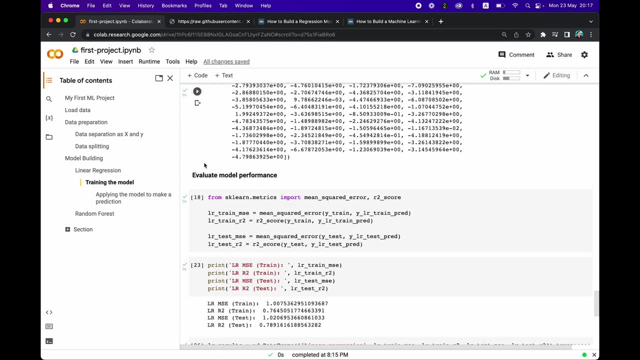 So if you want this to appear here, then we need to add more. So this is two, then we need to make three here. add three And you're gonna notice it appears here. Add three. It might be good because you could also, you know. 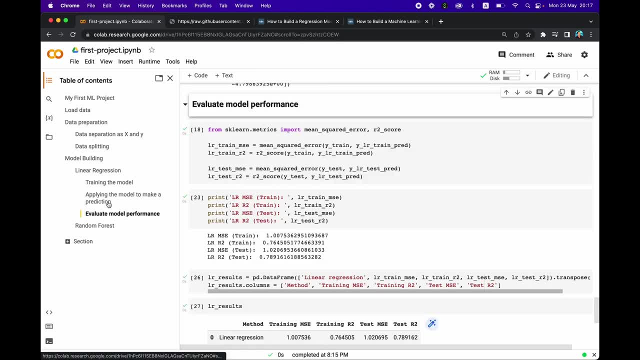 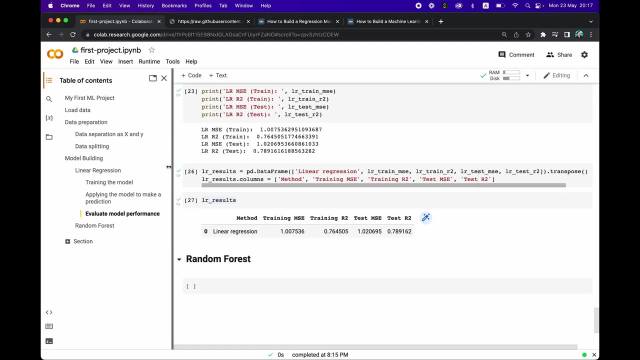 hop around the notebook like this, you know, like on the various topic of your choice, And then you could skim through your Jupyter Notebook. And also the great thing is that you could take a look at your table of content without you know. 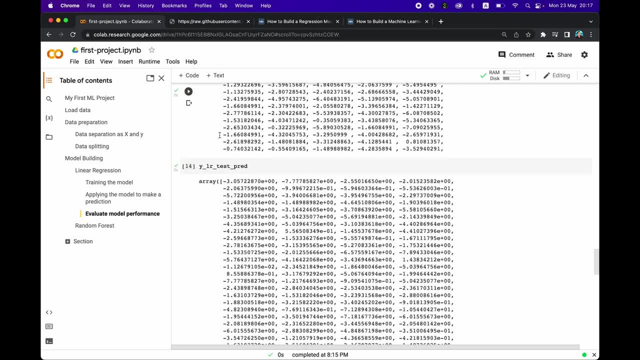 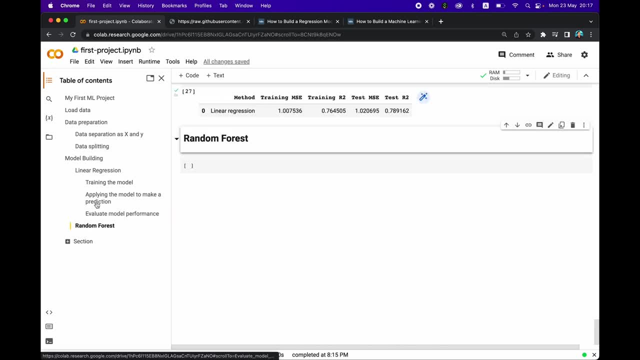 scrolling up and down to see what's the name of the cell, because sometimes your output might be quite long here and it might take some time right. But it'll be much quicker to just navigate by clicking on the particular link. So we could see here that we have training the model here. 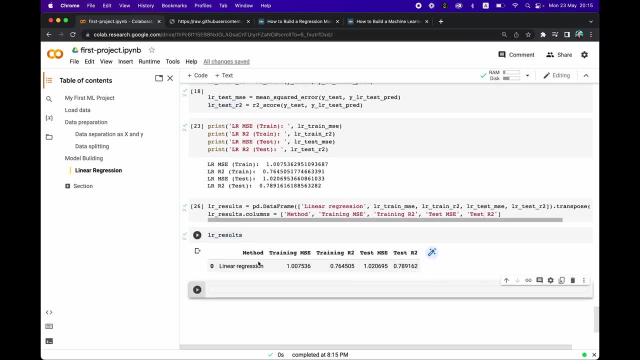 support vector machine neural network, then you're going to have a data frame that will allow you to easily compare. you could also sort by column the performance, and that will help you to evaluate which one was the best. so here you have already built a linear regression model and we're going 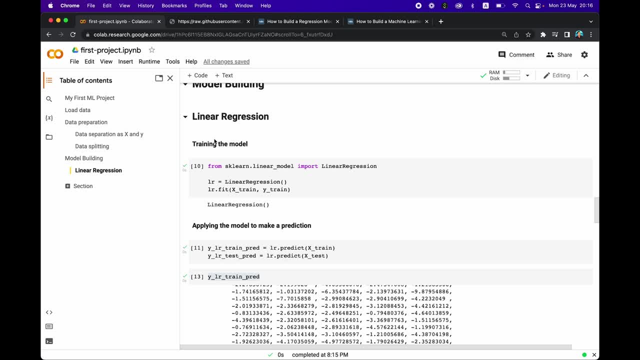 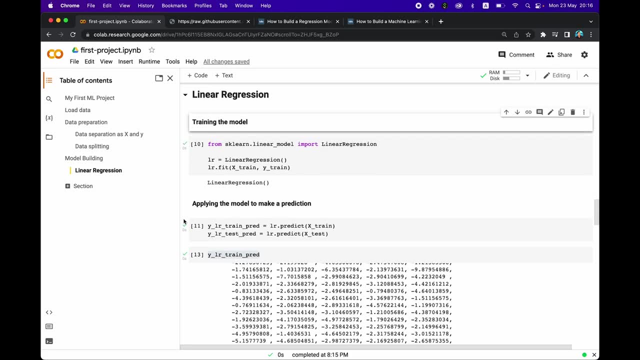 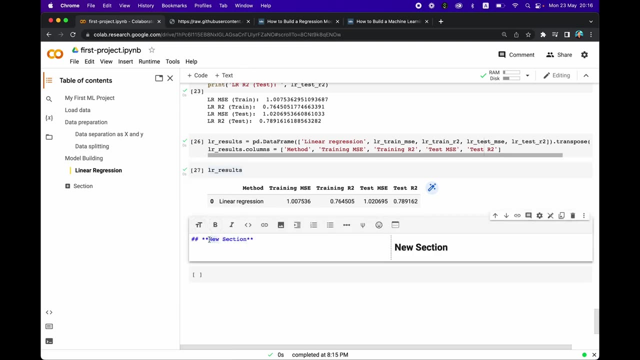 to try out another one, which is the random forest. let's see, we have two hash symbol here, so we're going to add a text cell, add two, and then we're going to call it random forest, random forest, and then you can see it here, but notice that you don't see the bold text because 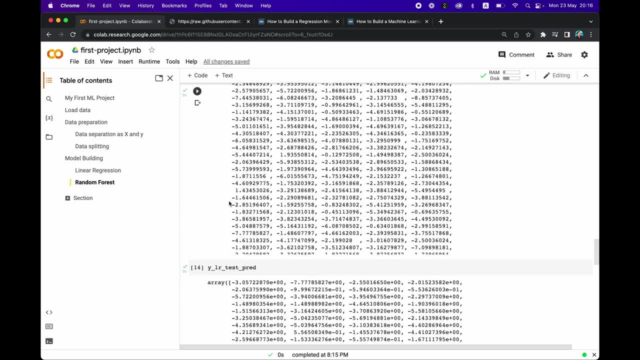 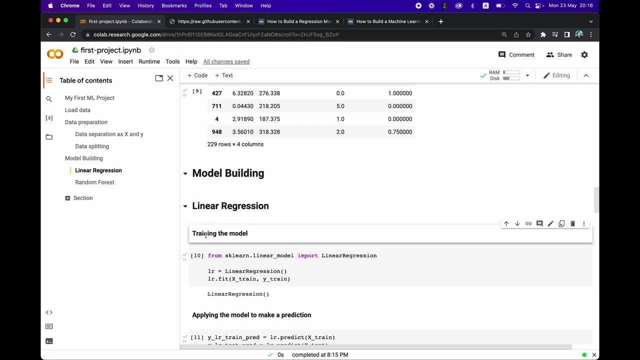 it needs to be in a hash symbol which will give it a heading one, heading two, hitting three, you know, like the hierarchical order of the hash symbol. so we're going to call it random forest. so if you want this to appear here, then we need to add more. so this is two, then we need to make: 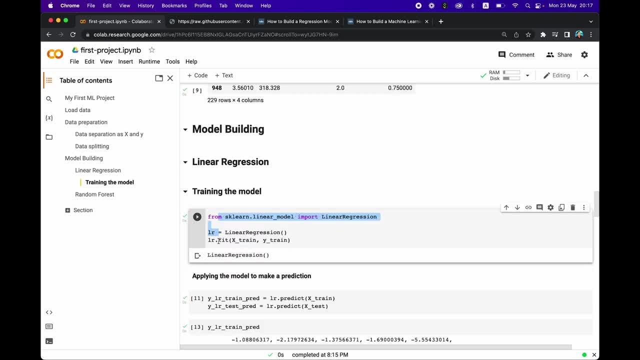 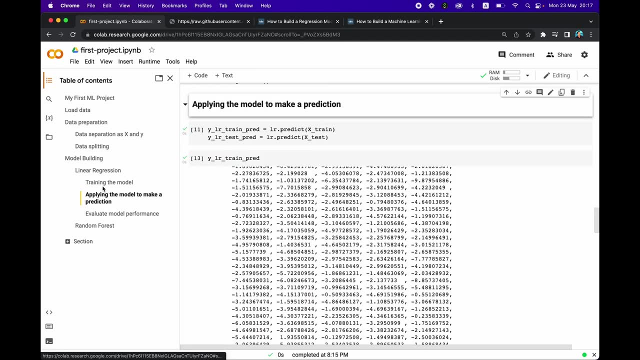 three here, add three and you're going to notice it appears here at three. it might be good because you could also, you know, hop around the notebook like this, you know, like on the various topic of your choice, and then you could skim through your jupyter notebook. and also the great thing. 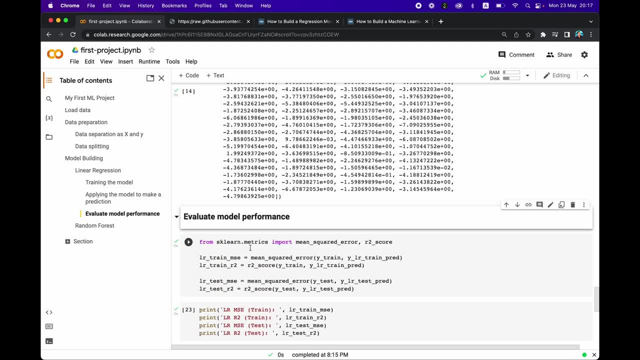 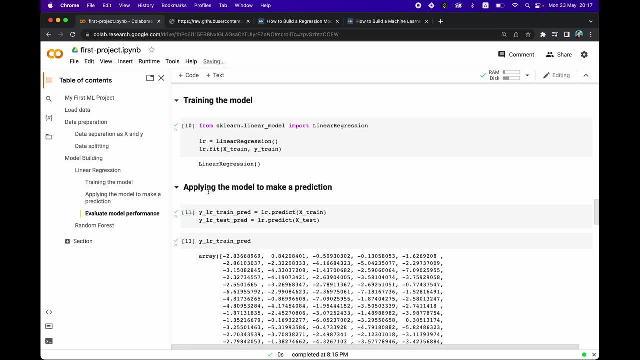 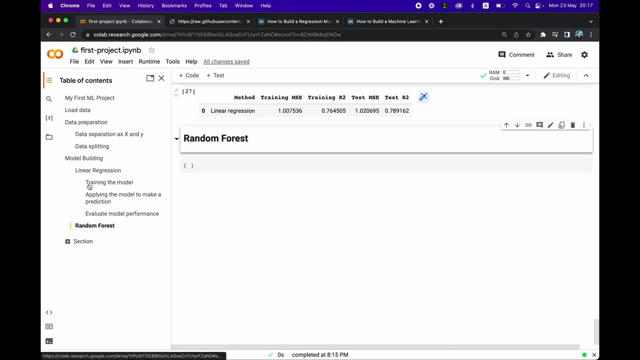 is that you could take a look at your table of content without you know, scrolling up and down to see what's the name of the cell, because sometimes your output might be quite long here and it might take some time, right, but it'll be much quicker to just navigate by clicking on the particular link. so we could see here that we have 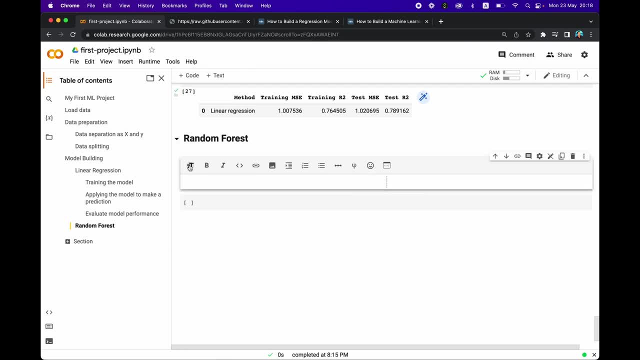 training the model here. so we could just add section called training the model, training the model, and then let's just add the headings and then applying the model to make a prediction, then evaluate model performance. so we could move this up a bit. so we're going to train the model. 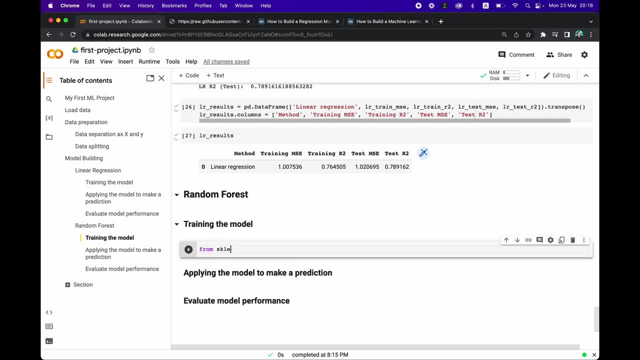 using the random forest algorithm. so from sklearn dot ensemble import random forest regressor. so a point of note here is that this particular tutorial video makes use of regressor because we're building regression models and it is because the y variable, which is called log s. let me show you log s right here. 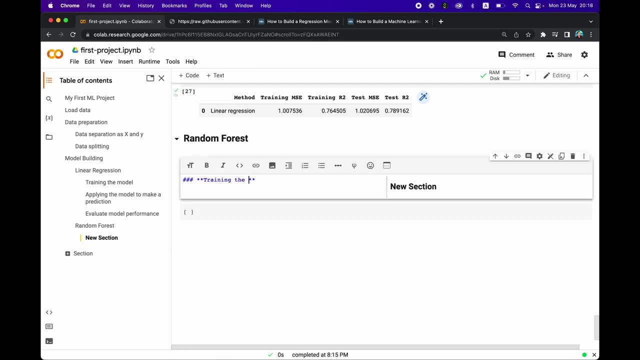 So we could just add section called training the model, training the model, And then let's just add the headings and then applying the model to make a prediction, then evaluate model performance. So we could move this up a bit. So we're gonna train the model. 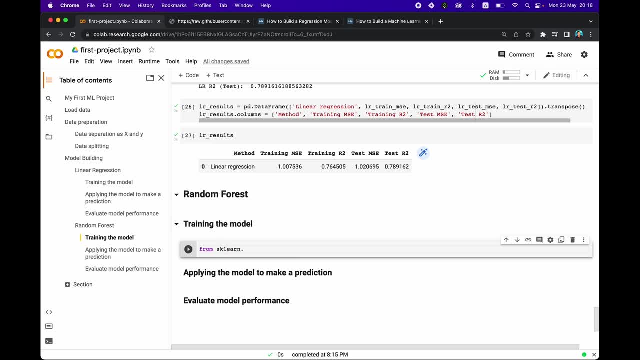 using the random forest algorithm. So from sklearnensemble import random forest regressor. So a point of note here is that this particular tutorial video makes use of regressor because we're building regression models And it is because the Y variable, which is called log S. 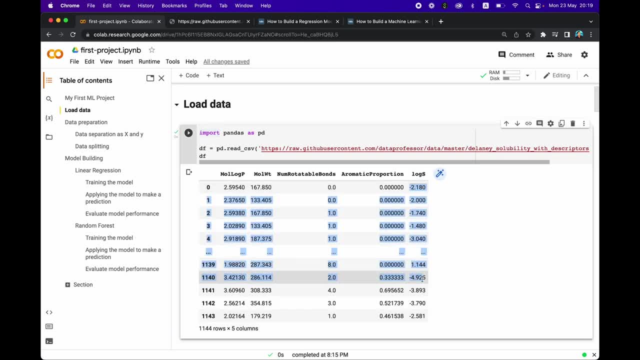 let me show you log S right here. It's a quantitative value. So if the Y variable is quantitative, we're going to build a regression model, Whereas if it is categorical, then we're going to build a classification model. okay, So in this tutorial the log S is quantitative. 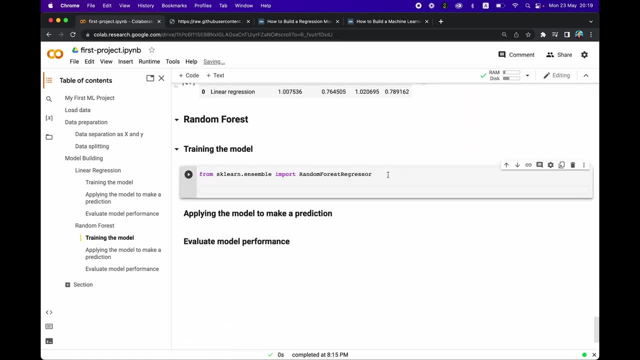 Therefore we built the regression model, Because random forest here has two versions: random forest regressor and random forest classifier- And here we're using the regressor. So we're gonna create a RF variable to house the random forest algorithm And we're gonna specify some of the parameters. 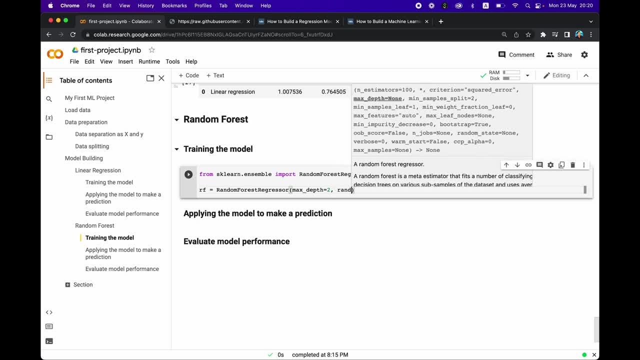 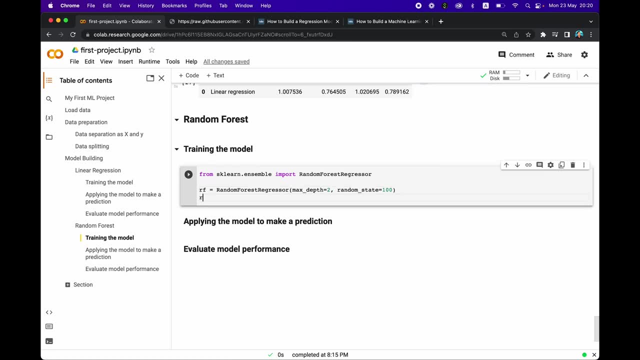 for the model here: maximum depth of two and the random state of what about 100?? Because in the prior random state we used 100. And now we're gonna train the model, So we're gonna type in RF fits and then we're gonna use X train. 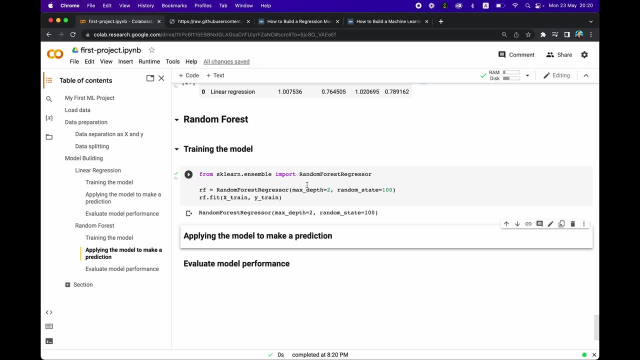 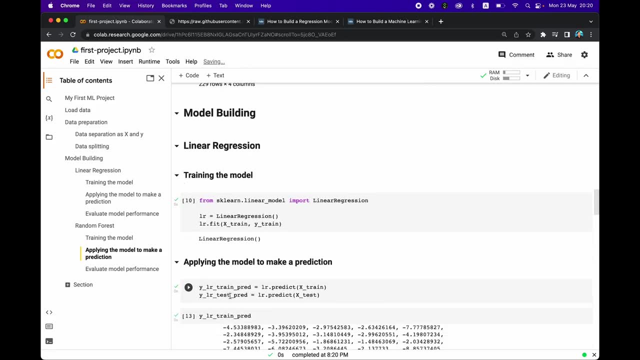 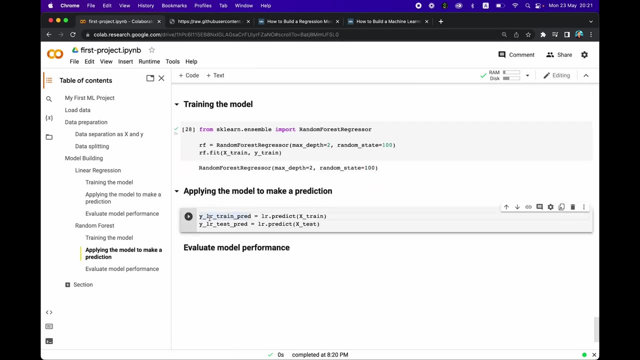 And Y train, And then we run it to train the model, and the model is trained. We're now gonna make the prediction in here, So actually we could just copy the code cell above here, Scroll down, And we're gonna change this to be RF, RF. 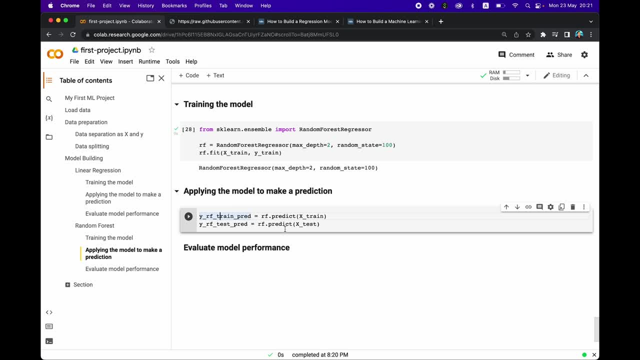 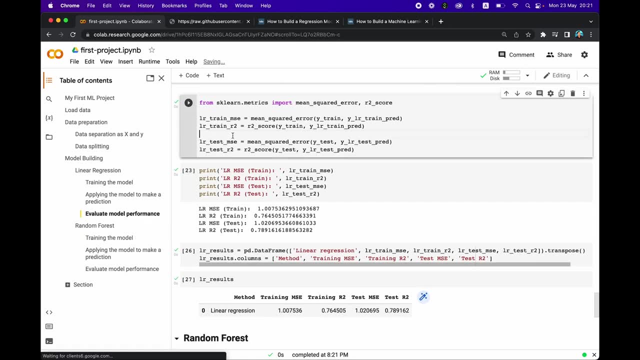 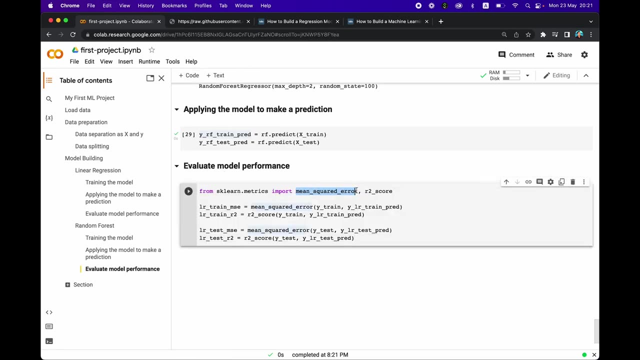 LR to be RF, RF, And now it looks correct to me and we're gonna run it. Okay, And now we're gonna do the model performance Evaluation. I'm gonna copy the code here, paste it. We're gonna use the mean squared error. 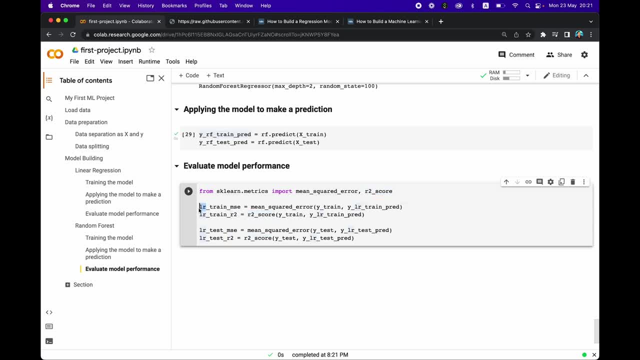 and we're gonna use the R2 score And here, instead of LR, we're gonna replace that to be RF. okay, So replace all of the LR to be RF And be mindful maybe you might type in wrong- like me just a moment ago- to be FR. 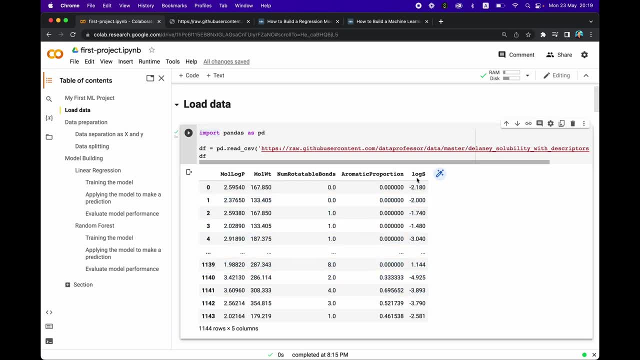 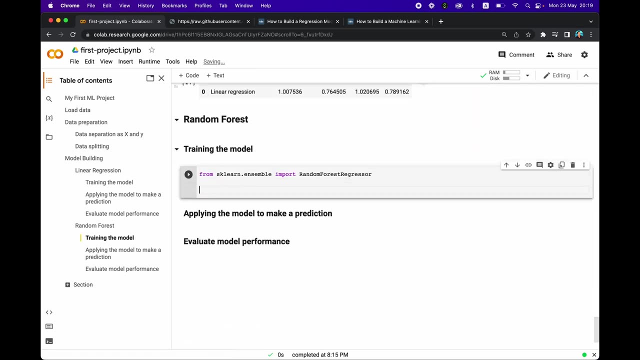 it's a quantitative value. so if the y variable is quantitative, we're going to build a regression model, whereas if it is categorical, then we're going to build a class classification model. okay, so in this tutorial the log s is quantitative. therefore, we built the regression model, because random forest here has two versions: random forest regressor and random. 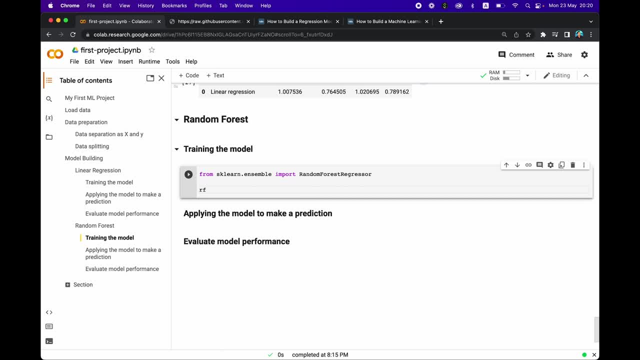 forest classifier, and here we're using the regressor. so we're going to create a rf variable to house the random forest algorithm and we're going to specify some of the parameters for the model here: maximum depth of 2 and the random state of what about 100? because in the prior 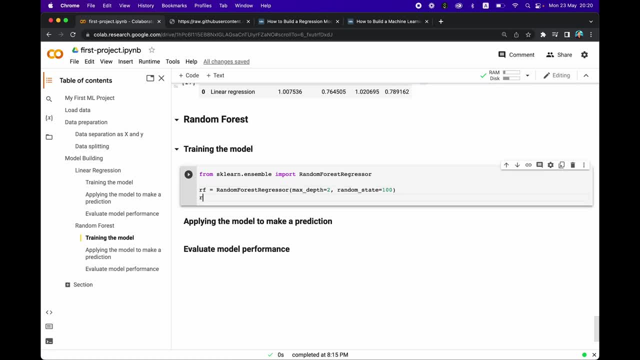 random state. we used 100, and now we're going to train the model, so we're going to type in rf fits and then we're going to use x train and y train and then we run it to train the model and the model is trained. we're now going to make the prediction in here, so actually we could just copy. 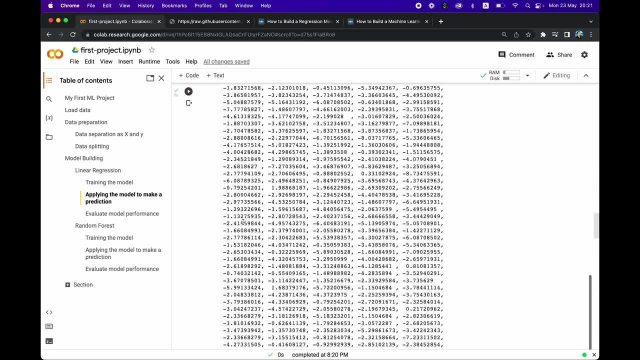 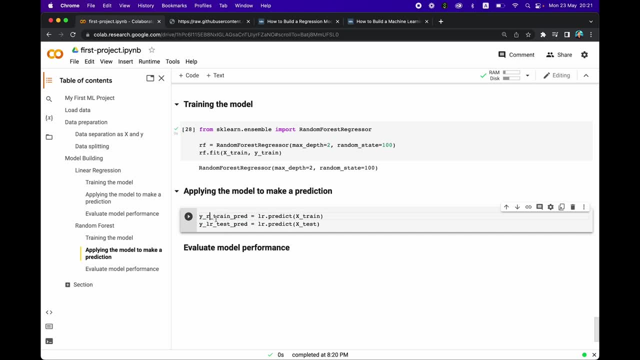 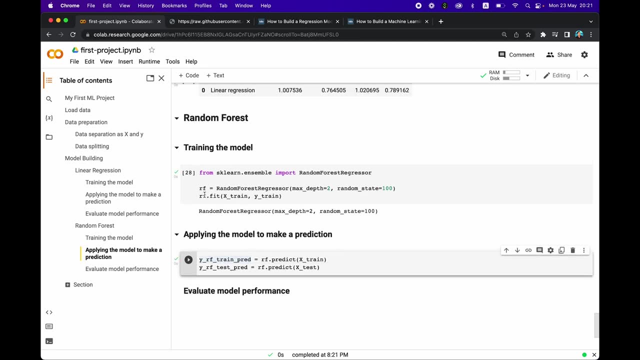 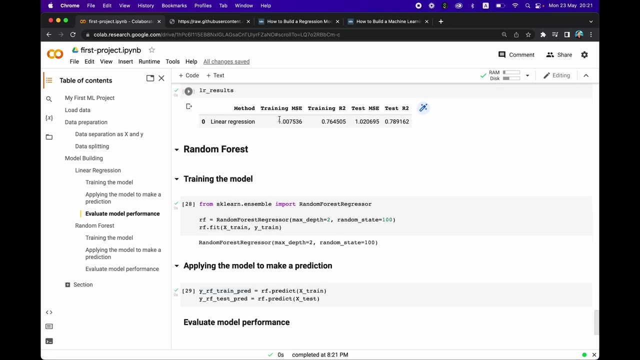 the code cell above here, scroll down, and we're going to change this to be rf, rf, lr, to be rf, part f, and now it looks correct to me and we're going to run it. okay. and now we're going to do the model performance evaluation. i'm going to copy the code here, paste it. we're going to use the mean squared. 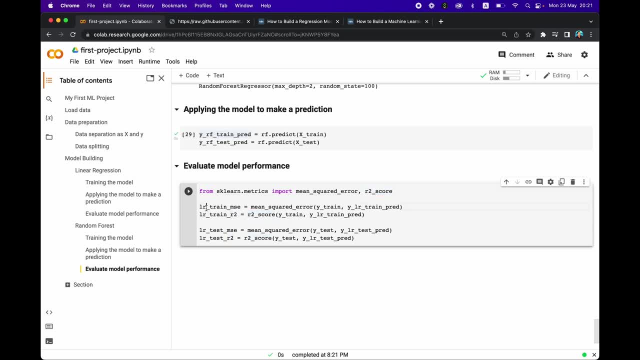 error and we're going to use the r2 score and here, instead of lr, we're going to replace that to be rf. okay, so replace all of the lr to be rf and be mindful maybe you might type in wrong- like me just a moment ago- to be fr. so 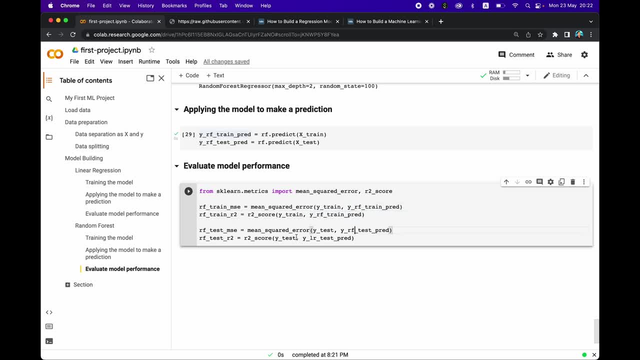 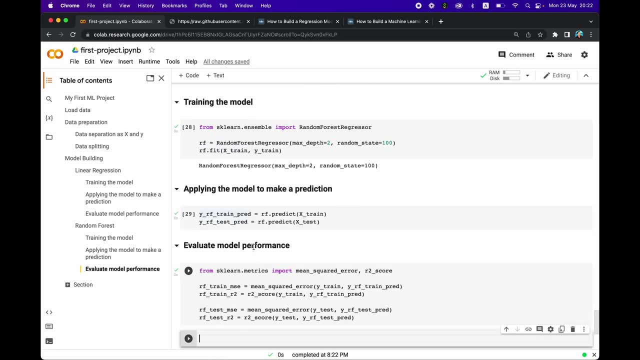 So RF here will be RF, LR here will be RF, RF and R. Did I say RF just a moment ago? It say LR and now it's RF. Okay, Let's run it and let's copy the code here which we used to make the table. 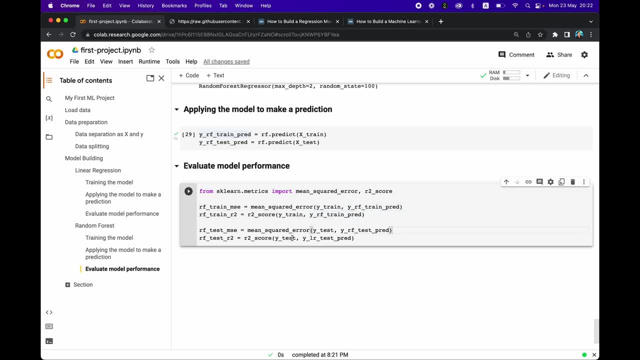 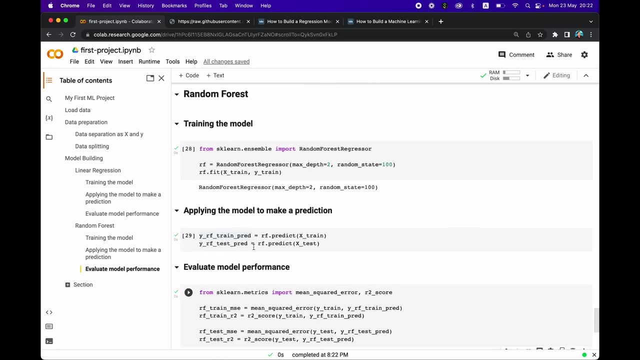 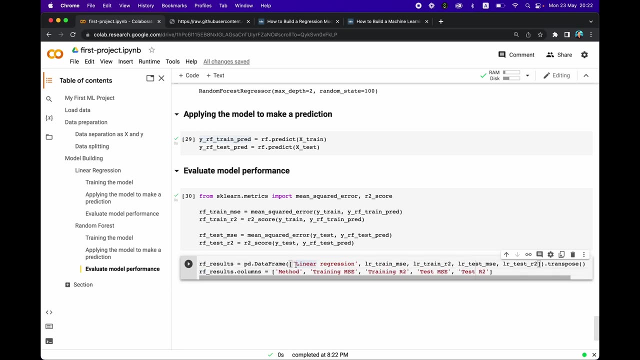 rf, here will be rf. how r? here will be rf, rf and r. did i say rf just a moment ago? i meant to say lr and now it's rf. okay, let's run it and let's copy the code here which we use to make the table, and we're gonna change this to be rf again and this will be random forest rf. okay, and here. 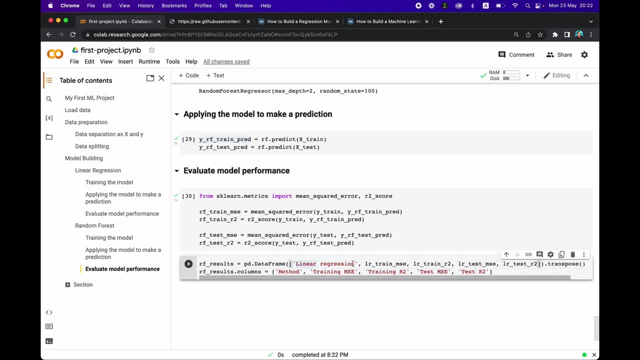 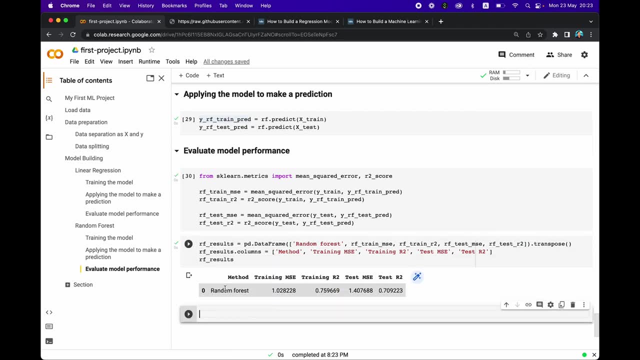 And we're gonna change this to be RF again And this will be Random Forest RF. okay, And here RF has showed the table, okay, And now we have two tables: We have the linear regression table and we have the random forest table. 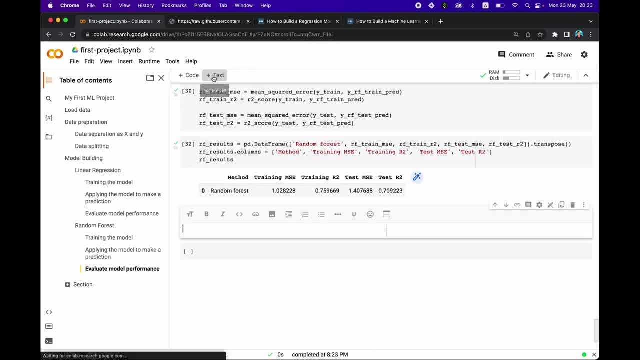 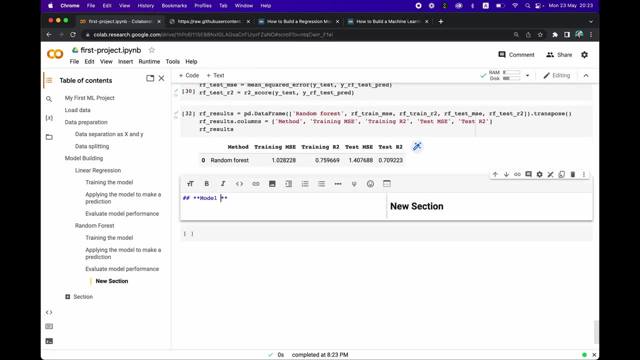 So why don't we combine the two tables together? Okay, Let me create another level. See What level is this? this random for us with the two hash. so one, two model comparison, and now we're going to compare it. so we're going to combine the two results table into one. and let me see: df models: equal pdconcat. 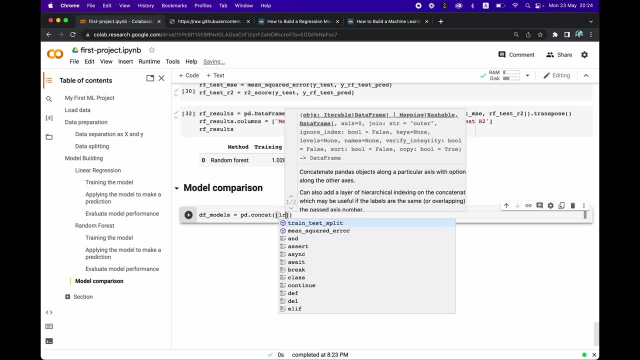 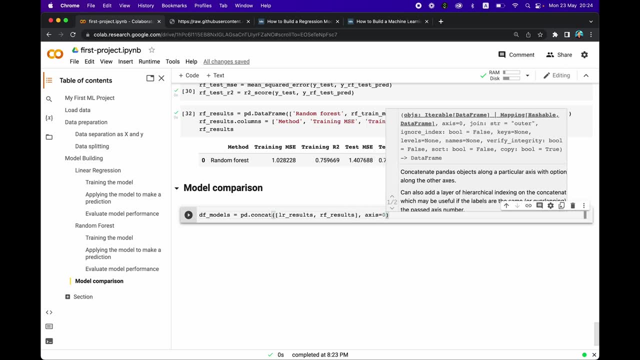 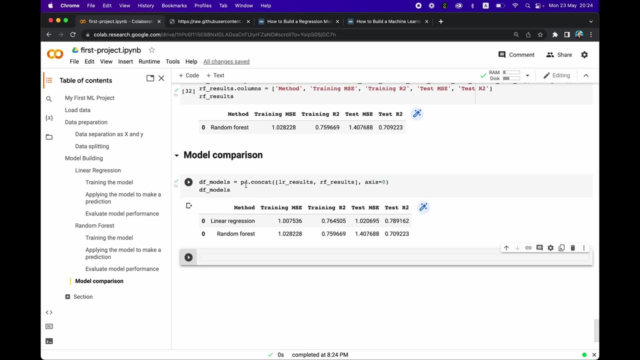 and then i'm going to specify the name of lr results and rf results. see, do i have x equals to 0, because i want to combine it in a worldwide manner. let me try if it works. all right, it worked. yeah, so x is equal to 0 if you want to combine in a row wise manner, whereas if you use axis 1, it. 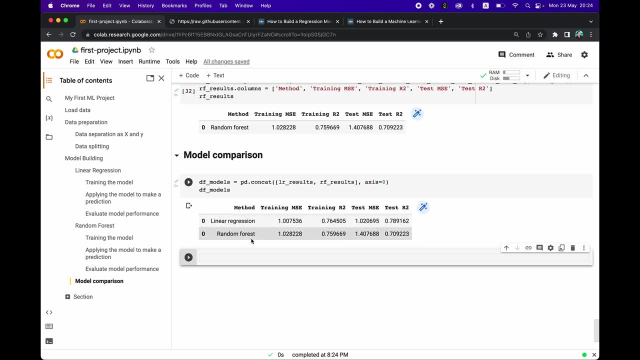 will be in a column wise manner. so here we're stacking them on top of one another. okay, so you can see now that the two are in the same table, but then the index number is a bit off, so we need to re-index that. so let me see if it's as simple as doing this index. 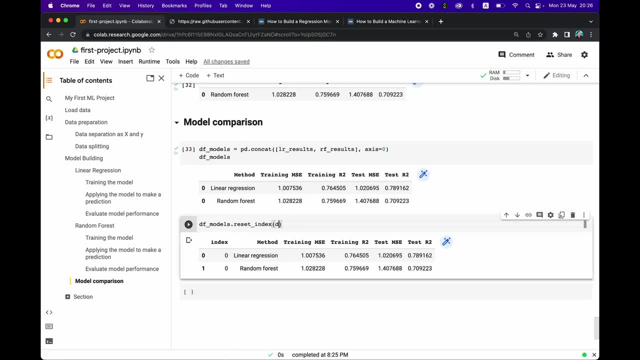 okay. and then it also added a new column here. we took, say, draw it true, oh, and now it worked. we could have also added this to the back of here: run again and the number is correct, okay, but i'm just gonna separate it so that it looks a bit more tidy and 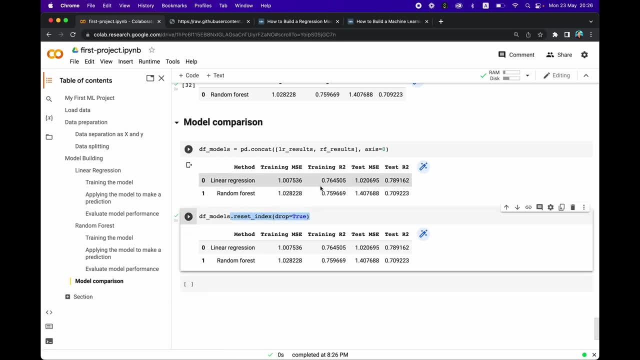 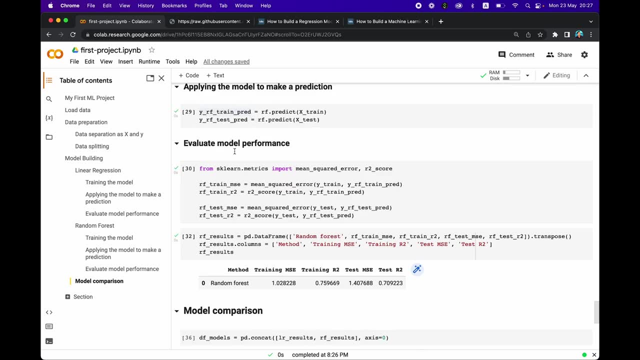 you could see it, but you know how to make it into a one-liner: you could just copy here and paste it at the end. so here you can see that we have already compared linear regression model and the random forest model. let's have a look at the scikit-learn. okay, and if you click here, regression. 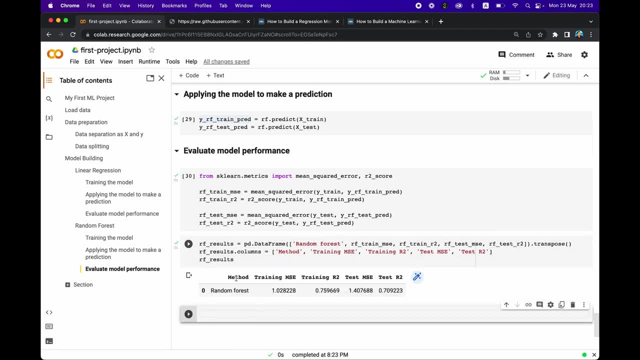 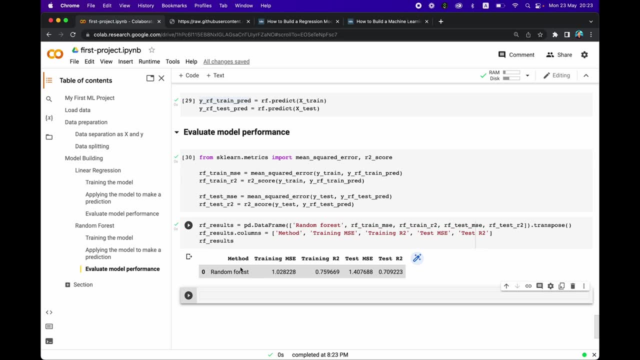 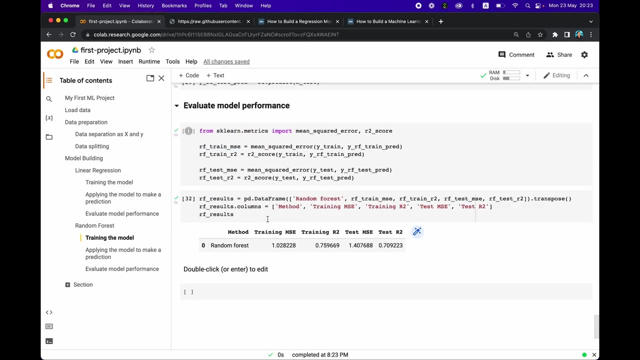 rff show the table. okay, and now we have two tables. we have the linear regression table and we have rf table. so why don't we combine the two tables together? okay, let me create another level. see what level is this random for us with the two hash. so one, two model comparison. and now we're gonna. 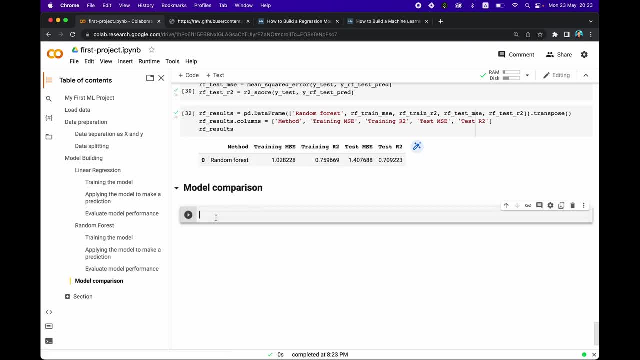 compare it. so we're gonna combine the two results table into one. and let me see: df models, equal, pd, dot, concat, and then i'm going to specify the name of lr results and rf results. see, do i have x? equals to zero, because i want to combine it in a row wise manner. let me try. if it works, all right. 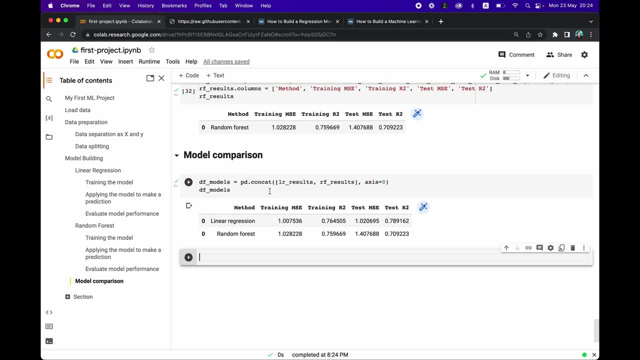 it worked. yeah, so x is equal to zero if you want to combine in a row wise manner, whereas if you use axis one, it will be in a column wise manner. so here we're stacking them on top of one another. okay, so you can see now that the two are in the same table, but then the index number is a bit. 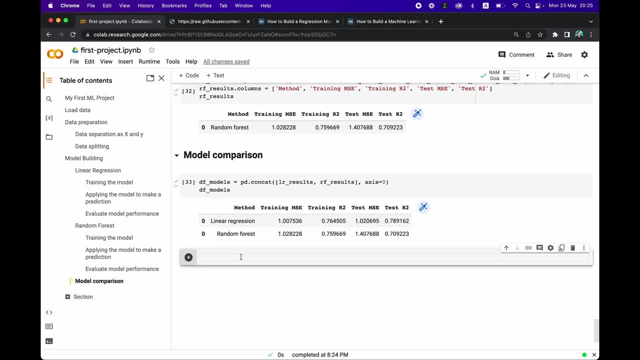 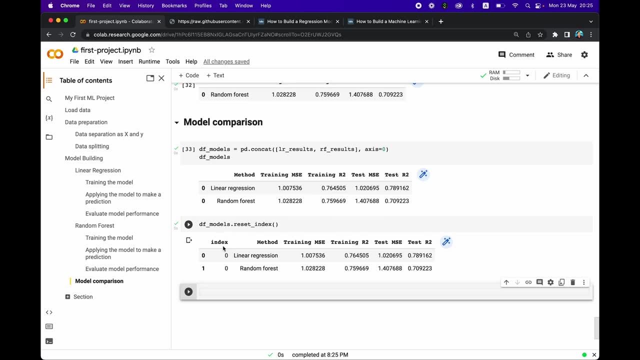 off, so we need to re-index that. so let me see if it's as simple as doing this index. okay, and then it also added a new column here. we just say: draw it true. oh, and now it worked. we could have also added this to the back of here: run again and the number is correct, okay. 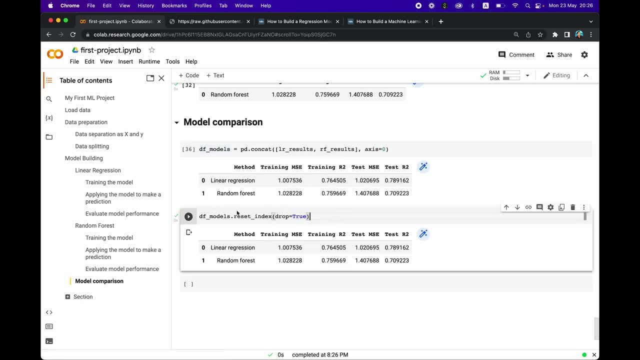 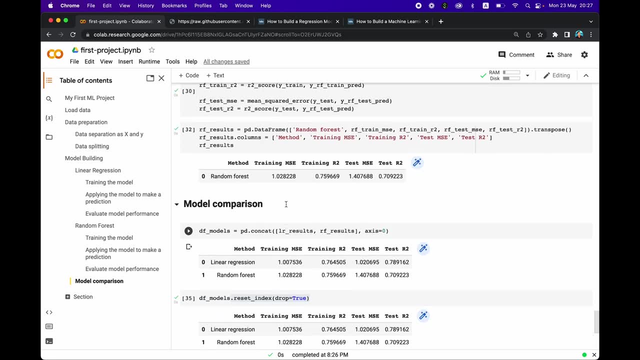 but i'm just gonna separate it so that it looks a bit more tidy and you could see it. but you know how to make it into a one-liner. you could just copy here and paste it at the end here. so here you can see that we have already compared linear regression model and the random. 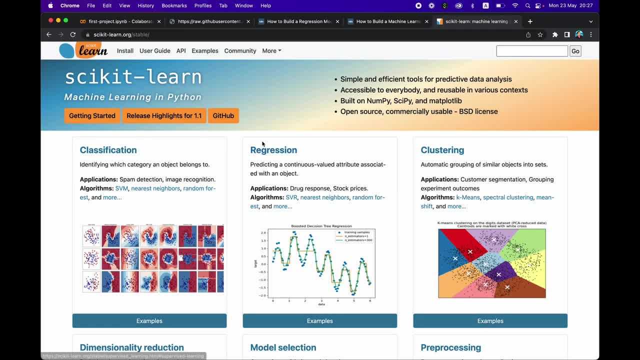 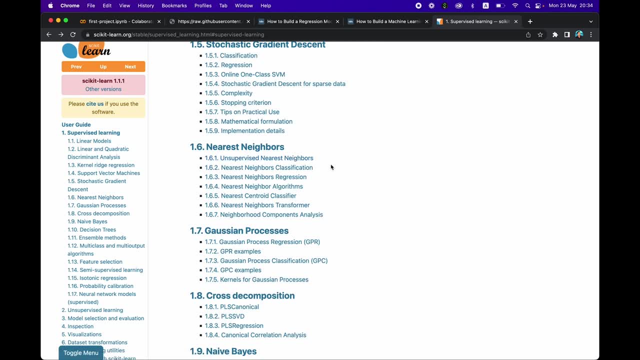 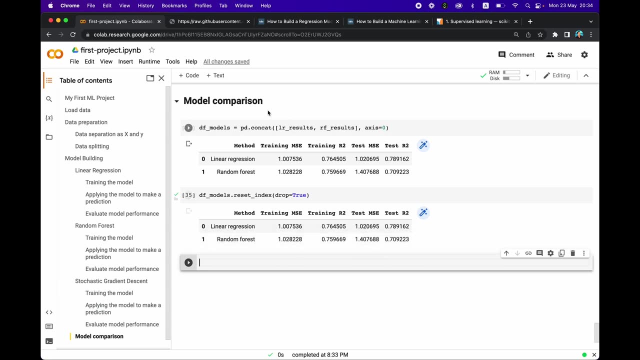 forest model. let's have a look at the scikit-learn, okay, and if you click here, regression and so here, you could find other regression model that you like and you could use it to build your own in the colette mood book here and then you could then add the resulting performance into the data. 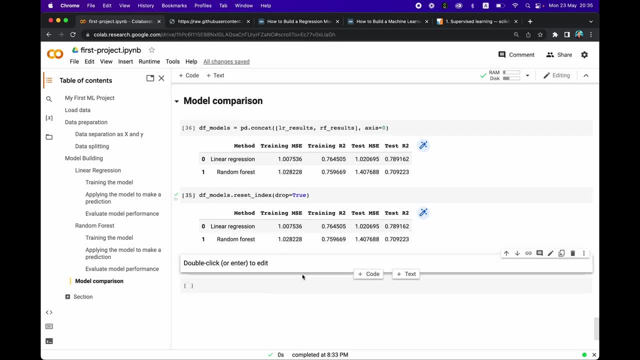 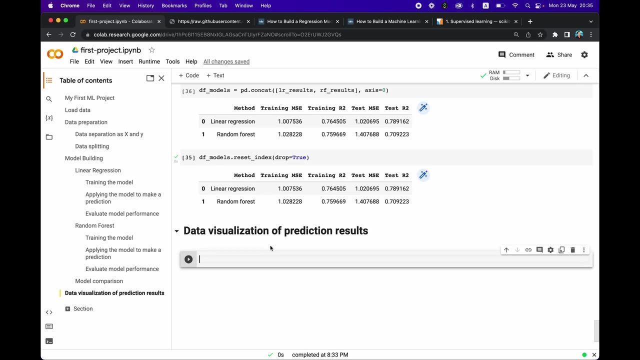 frame here to make your comparison. and so now we're going to perform data visualization to take the predicted value and the actual value and make a scatter plot. let's do it. let's say data visualization of prediction results, and we're going to make use of the 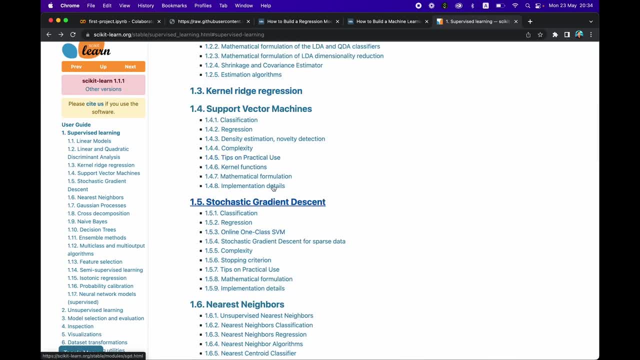 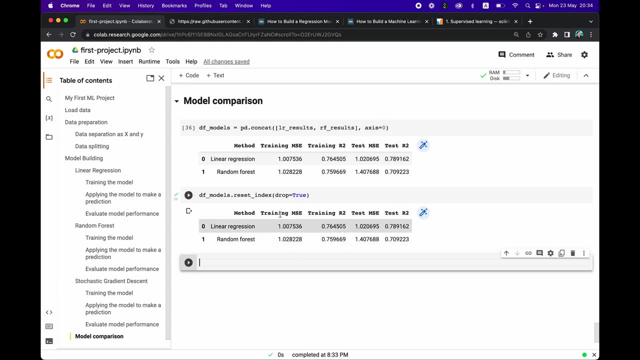 and so here you could find other regression model that you like and you could use it to build your own in the colette mood book here, and then you could then add the resulting performance into the data frame here to make your comparison. and so now we're going to perform data visualization to take the predicted 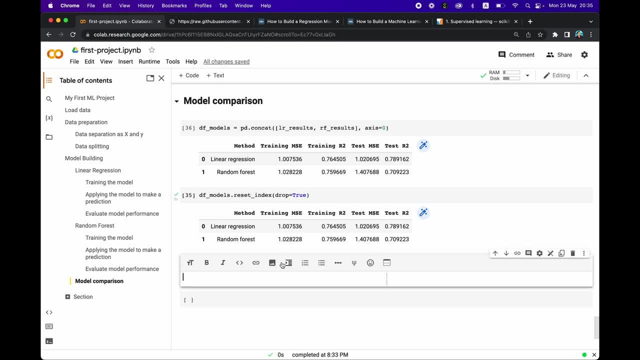 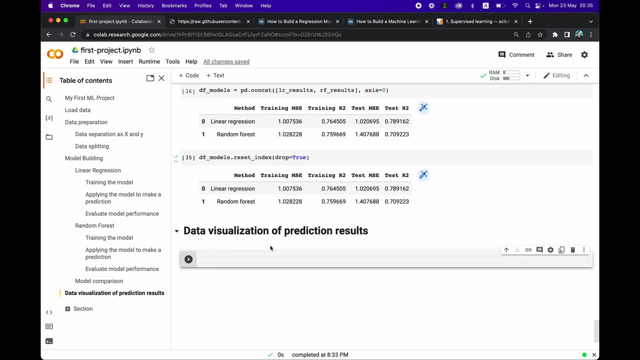 value and the actual value and make a scatter plot. let's do it. let's say data visualization of prediction results, and we're going to make use of the matplotlib library. so we're going to import matplotlib dot pi plot as plt. let's say plt scatter. i'm going to assign to the x-axis y-train and to the y-axis. 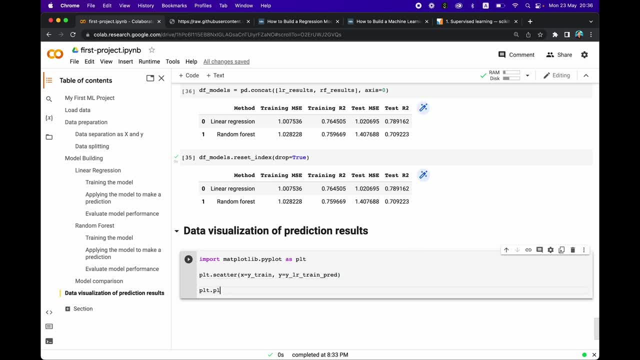 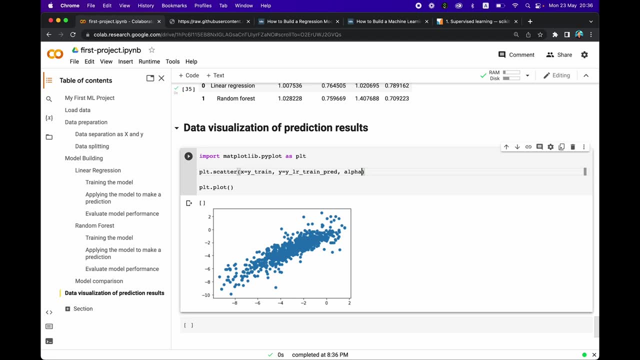 vl, our train pred, and let's make plots. okay, this is our first attempt. let's make it a bit lighter. you could adjust the darkness of the samples that you see here that are represented by the circles. the alpha option: we're making alpha to be 0.3 so that regions that are highly overlapping will be. 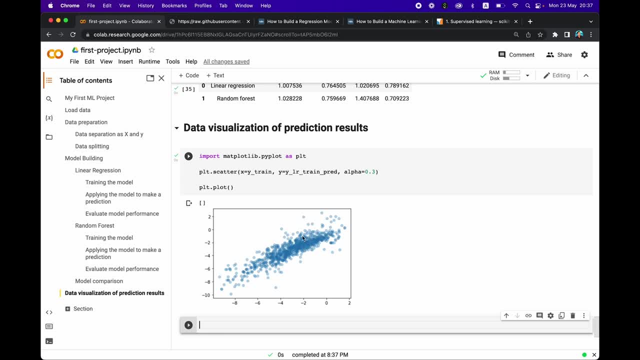 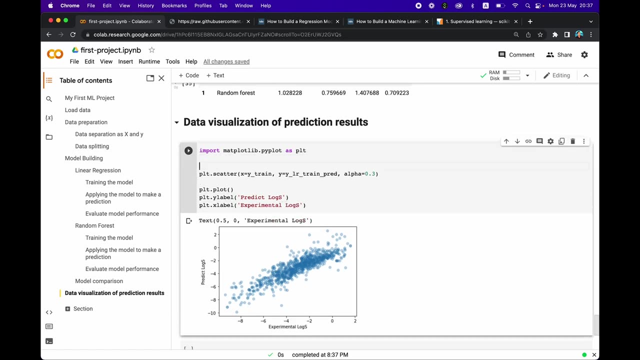 a bit darker, whereas those that are not overlapping will be lighter color, and you're going to see that the x and y axis is not yet labeled. we're going to do that. plt y label: predicted log s sc at label experimental s. okay, now we have the labels here, why don't we make it have same width and height? 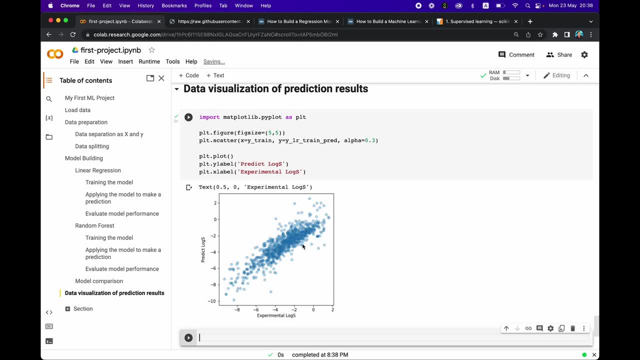 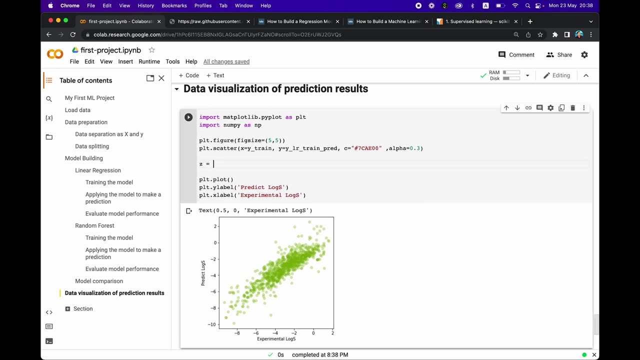 make fixed size to be 5 and 5. okay, why don't we make the dots here to be another color c color option? and we're going to use color green. and what about a trend line? let's add a trend line for that. we're going to use numpy, get the fitted line creating a z variable, np, dot, polyfit and then 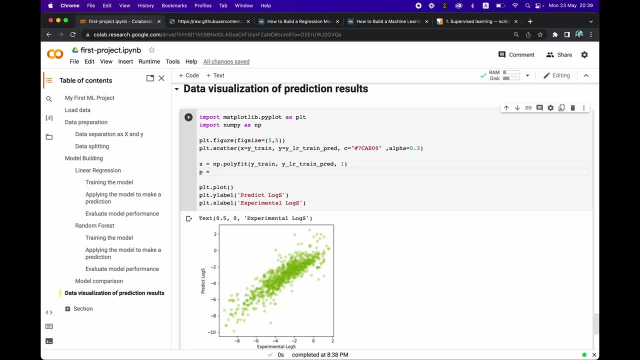 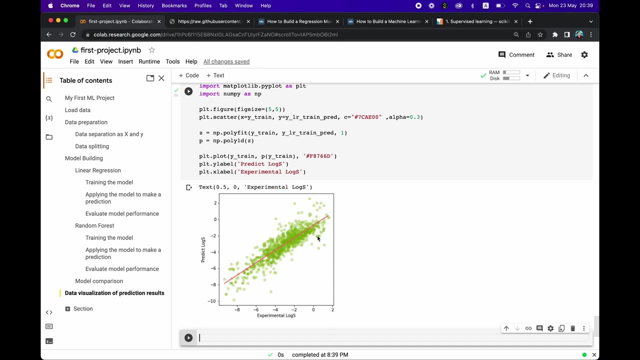 the y train and then lr train. red p equals z train each. then we're going to color to it: eight, seven, eight, seven, eight, seven. okay, there we go. so we added this red line as trend line that are fitted with the data here. so congratulations. you built your first machine learning model in python using the scikit learn. 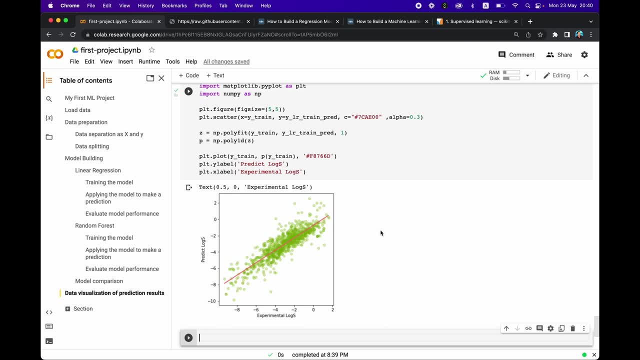 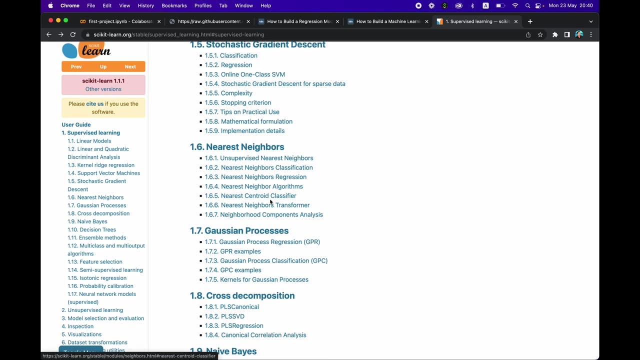 library so you can see how easy it is now to build models in python, particularly for your tabular data sets, and so please feel free to build more models and you could tweak the learning parameters and, as i have shown you this api documentation from scikit-learn you could go through the 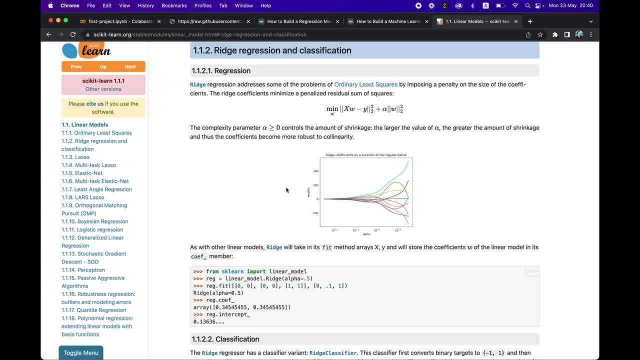 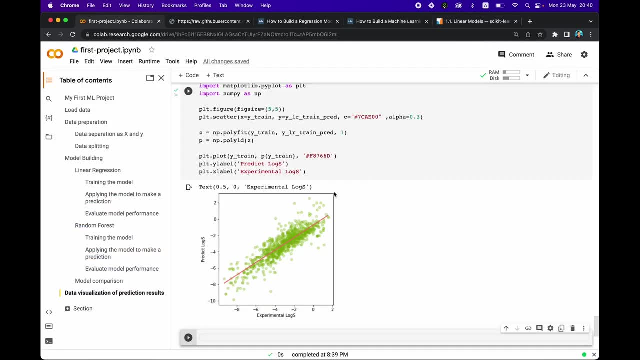 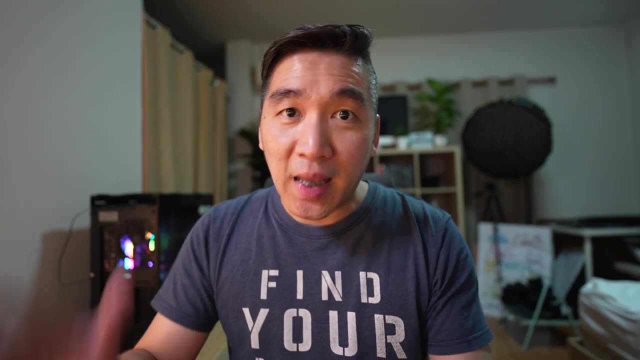 documentation. you could click on an algorithm that you're interested in, read about it and look at some of the parameters that it allows you to adjust. so give it some try. let me know in the comments down below what models that you are building, and have fun. thank you for watching until the end of. 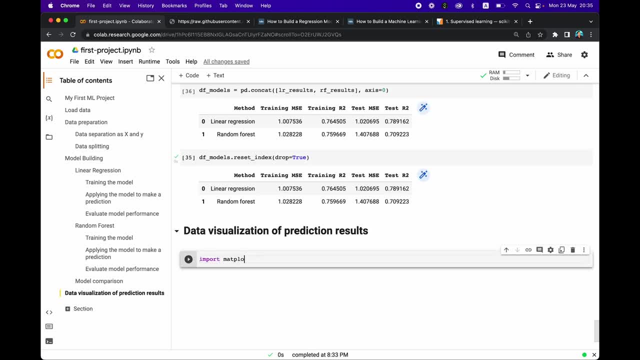 matplotlib library. so we're going to import matplotlib dot piplot as plt, let's say plt scatter. we're going to assign to the x-axis y-train and to the y-axis the lr train pred, and let's make plots. okay, this is our first attempt. let's make it a bit lighter, you could. 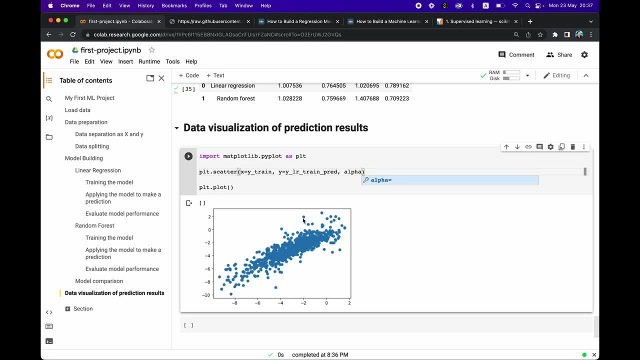 the darkness of the samples that you see here that are represented by the circles. using the alpha option. we're making alpha to be 0.3, so that regions that are highly overlapping will be a bit darker, whereas those that are not overlapping will be lighter color, and you're going to see that. 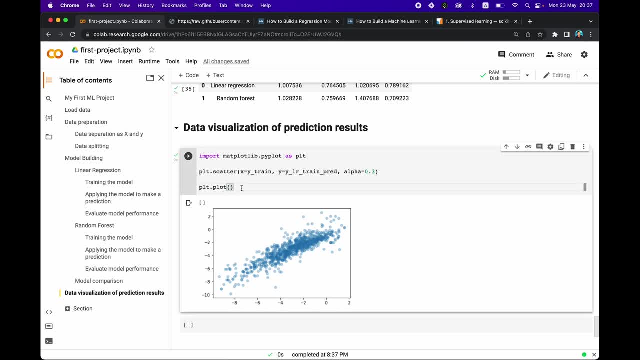 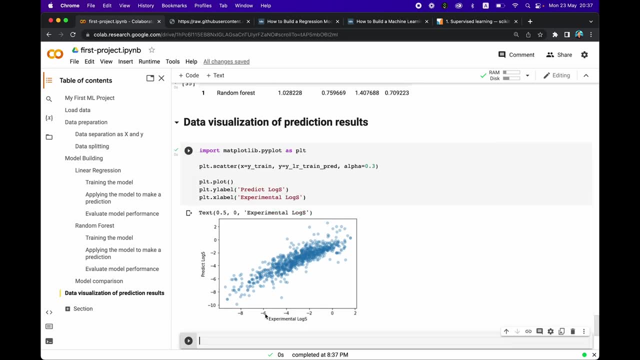 the x and y-axis is not yet labeled. we're gonna do that. plt y label, predicted log s, sc. add label experimental s. okay, now we have the labels, the parameters and you can see here that the below and here: why don't we make it have same width and height, make fixed size to be five and five okay. 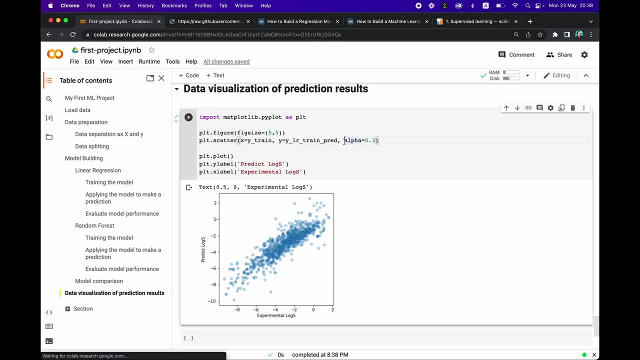 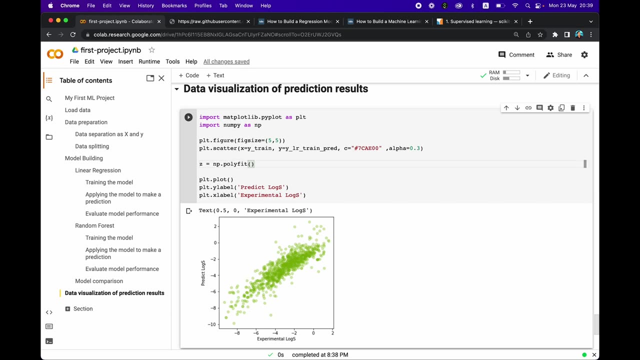 why don't we make the dots here to be another color c color option? and we're going to use color green. and what about a trend line? let's add a trend line for that. we're going to use numpy, get the fitted line, creating a z variable, np dot polyfit, and then the y train and then lr train. 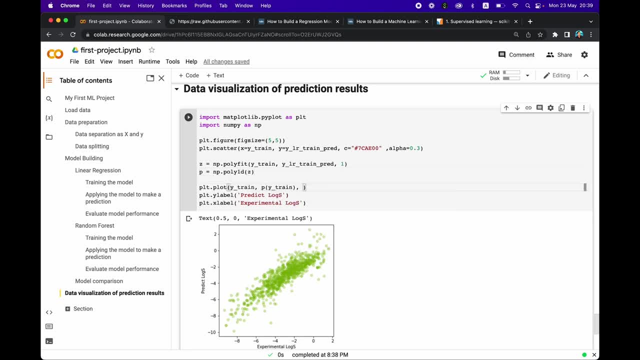 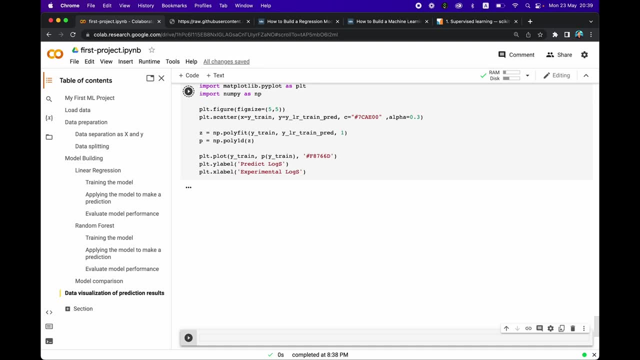 p equals z train each, then we're going to color to it. okay, there we go. so we added this red line as trend line that are fitted with the data here. so congratulations. you built your first machine learning model in python using the scikit-learn library, so you can see how easy it is now to build models in python particularly. 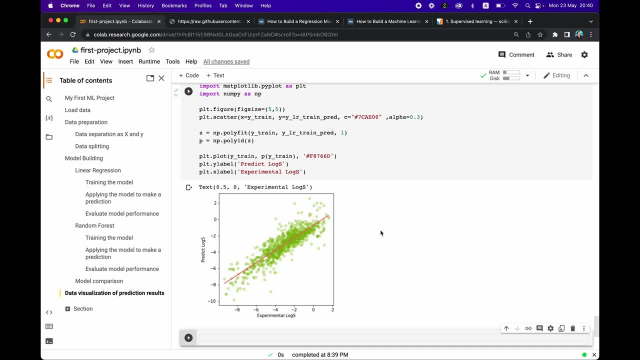 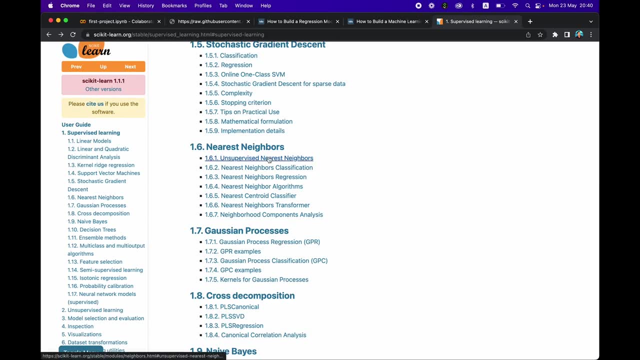 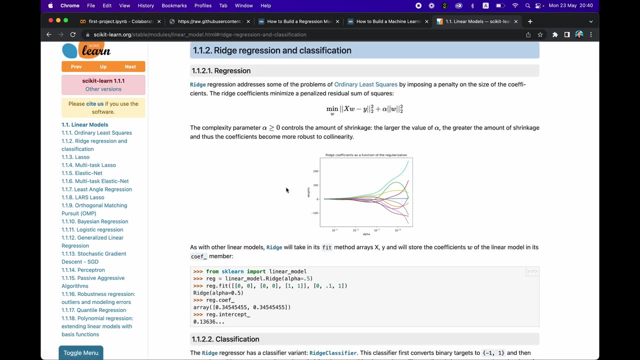 you can see how easy it is to build models in python, particularly for your tabular data sets, and so please feel free to build more models and you could tweak the learning parameters and, as i have shown you this api documentation from scikit-learn. you could go through the documentation. you could click on an algorithm that you're interested in. 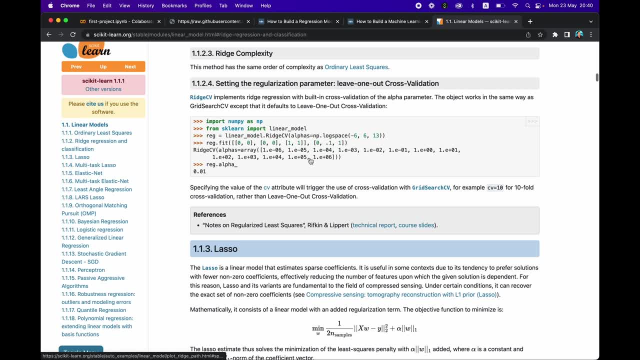 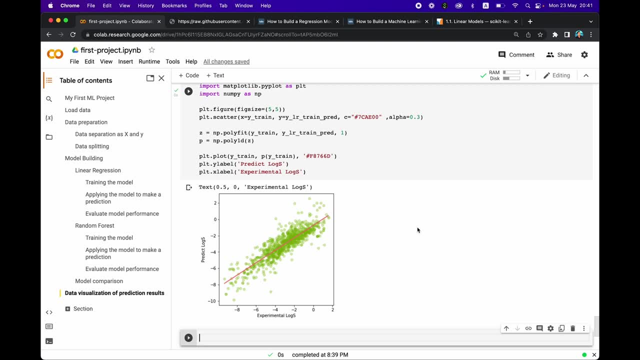 read about it and then look at some of the parameters that it allows you to adjust, and so give it some try. let me know in the comments down below what models that you are building and have a look at them, and then we'll see you in the next video.